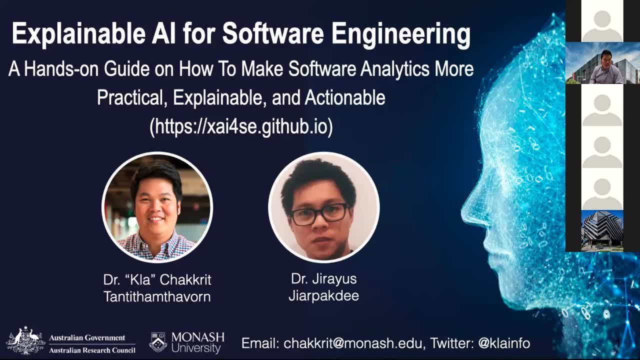 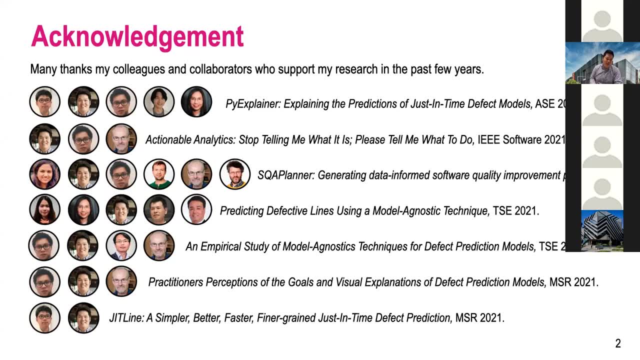 uh, if you have time or if you are interested, please, uh yeah, check it out as well. okay, so, before i uh start my talk, i just uh want to acknowledge, uh, my colleagues and my collaborators who support my research in the past few years. i think this topic is quite topical, but 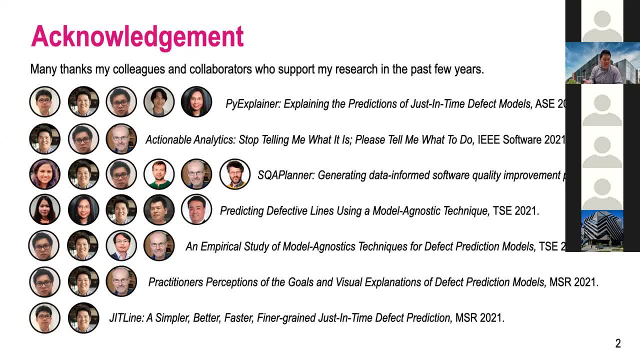 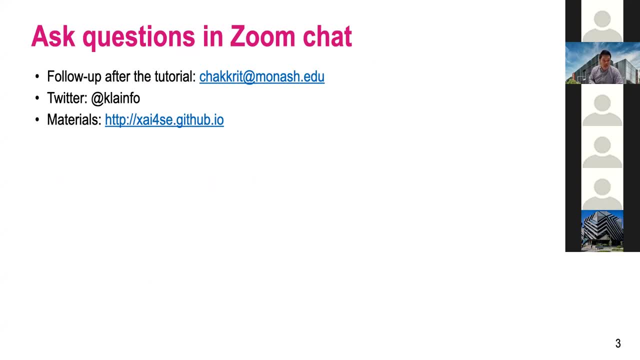 it has been rarely explored, uh, it still remains, uh challenging, you know. so, uh, i just want to say thank you to everyone who support my research. yeah, so, uh, if you have any questions, you can ask questions in the zoom chat, but after the tutorial, you can send me an email if you have any questions, or ask me on the twitter as well. and again, the, the. 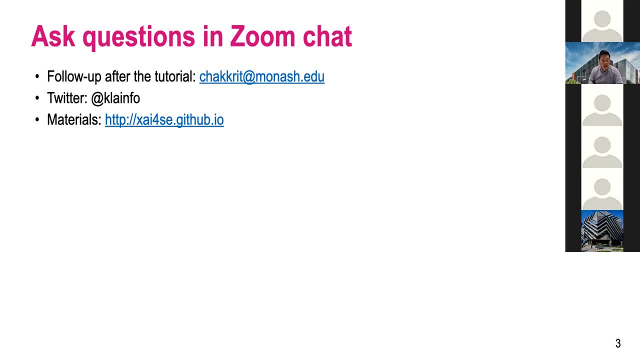 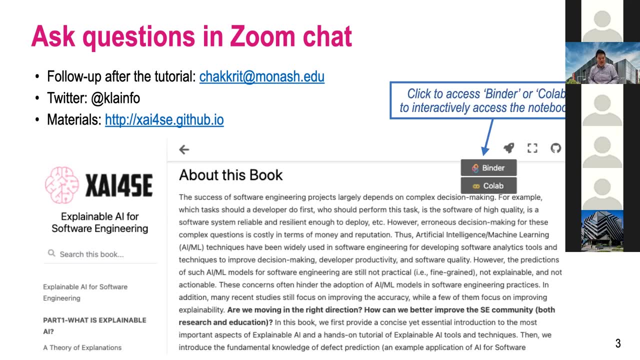 memories and comments are there and i will be happy to answer them tonight. so, uh, i really很好 brief interview before we collaborate and the uh, uh, the allows that you can get uh. uh, you know, um, your first job in ios are pretty new. uh, i think you can run uh the course very clearly. 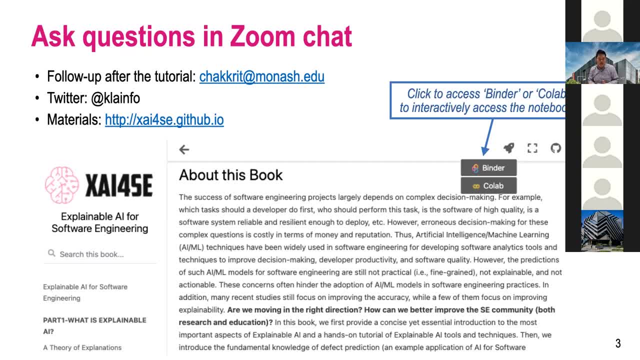 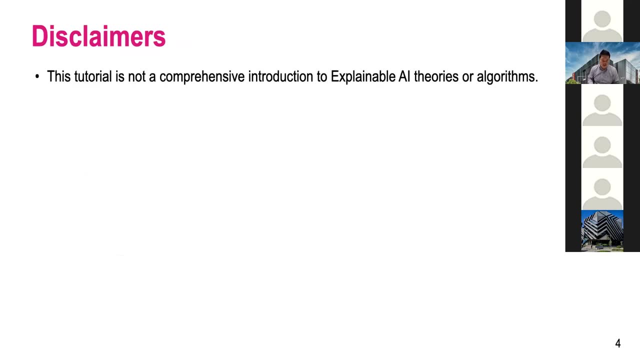 run the code on the web as well, without any installations or dependencies. so i think this is, uh this tutorial, uh this book is quite handy and accessible. yep, so, uh, before i start my talk, i just want to uh remind you that this tutorial is not a comprehensive introduction to 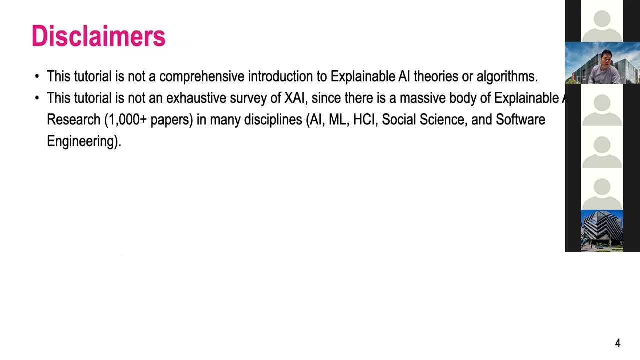 exit explainable ai theories or the algorithms- and this is not an exhaustive survey of the explainable ai as well, because there is a lot, of, lots of bodies of research about this area. i think, uh, it has been start uh like uh getting uh booming around 2016, so up uh like five years. 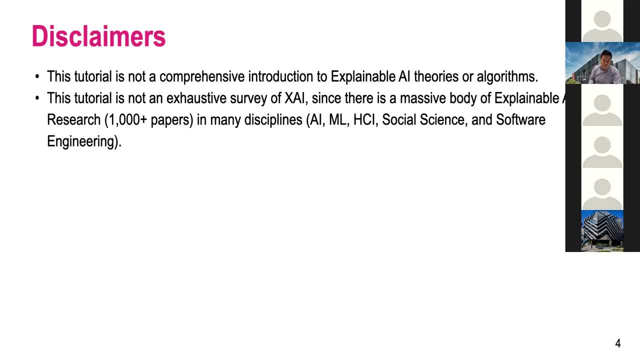 later i think it should have more than thousand papers, and those uh topics have been published in many disciplines as well, like ai, machines learning, HCI, social science and software engineering. So we cannot cover everything And we are software engineering researchers that try to make the AI for software engineering. 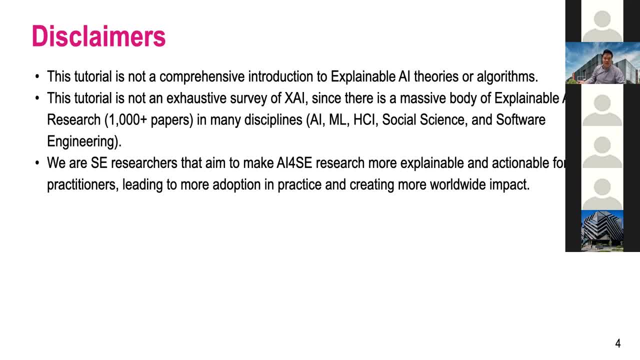 research more expandable and more actionable for practitioners So they can be widely adopted in practice or industry. So that means that this tutorial aims to motivate why the XAI is very important in software engineering and what is the concept behind. So I just want to 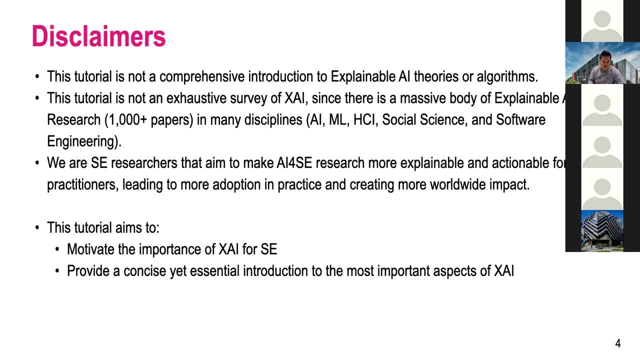 provide the key important aspect about the expandable AI. And finally, I just want to demonstrate some potential applications of the XAI for SE as well. Yep And finally, Kashumi, Hello, Can everyone please mute? Yep. Thank you. So, and finally, I just want to convince everyone. 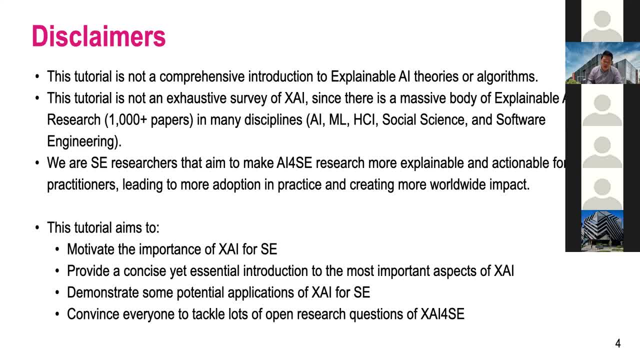 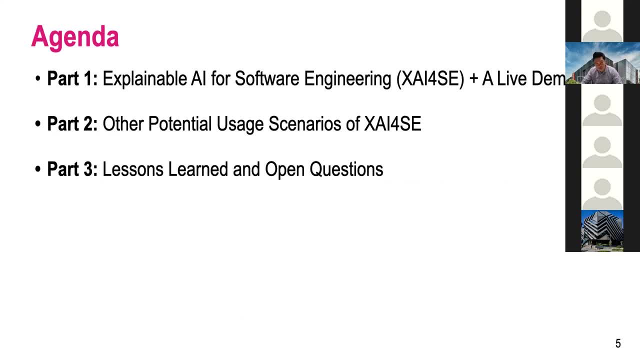 to tackle about this topic because there are lots of open research questions and challenges about the expandable AI for SE Yep. So the agenda of my talk today has three parts. First I will talk about what is the expandable AI for software engineering. 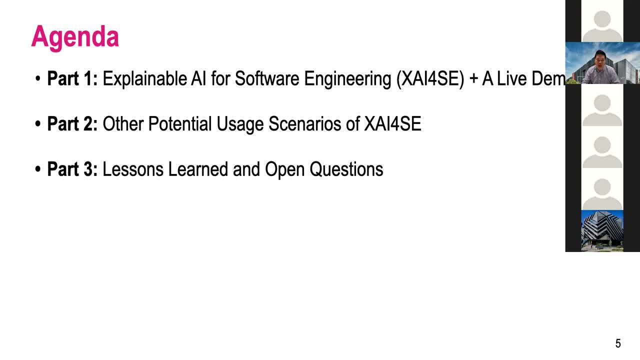 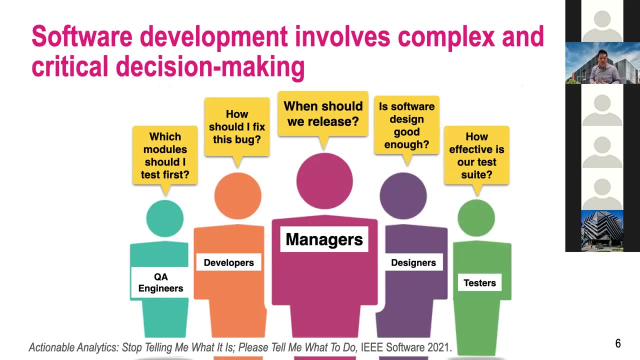 and then I will show some live demo as well, And then I will discuss about what are the potential usage scenarios And finally I will wrap up with the lessons learned and the open questions. So, in general, software development involves lots of complex and critical decision making. 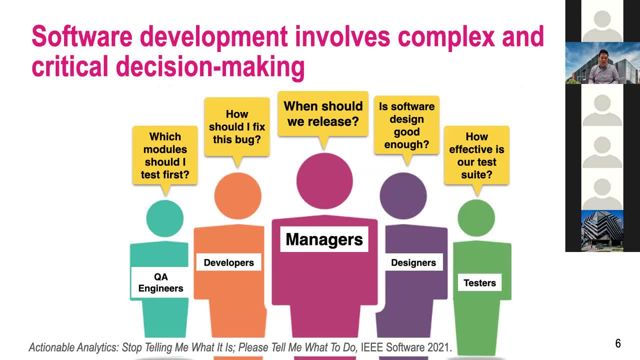 For example, as a manager, normally people should ask like: when should we release the software? as a developer during the program- Yeah, And then I will definitely cover some of them- I also want to uh during that development uh period. they also ask like: how should i fix this bug? and as a qa, 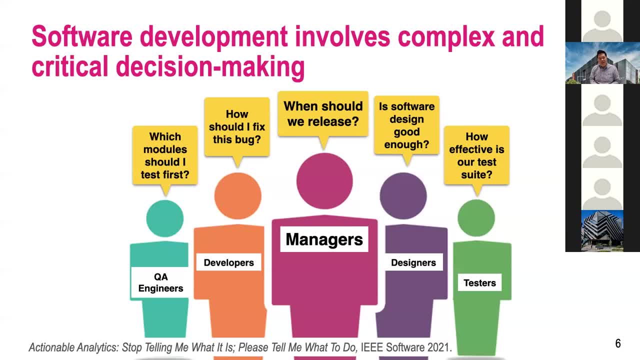 engineers. they also need to uh answer like uh. they also ask like: which modules should i test first? and as a designer, they also ask lots of questions like: is software decide good enough or not? as a tester, how effective is our test suite? so there are lots of questions behind, but 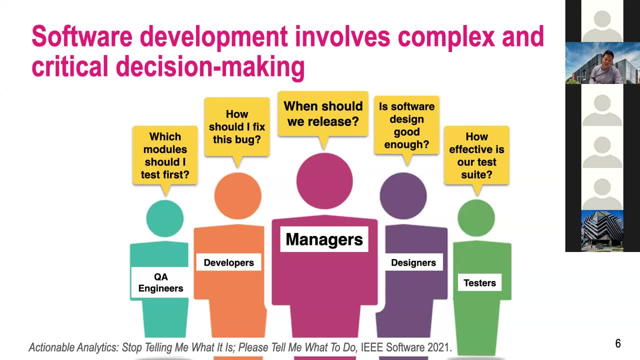 uh. at the moment there is no analytics. there's no like uh without analytics uh any uh erroneous in the decision making can goes wrong, go badly. you know, like uh. it will make the companies uh very costly. it will impact the reputations of the companies as well. so recently ai and machine 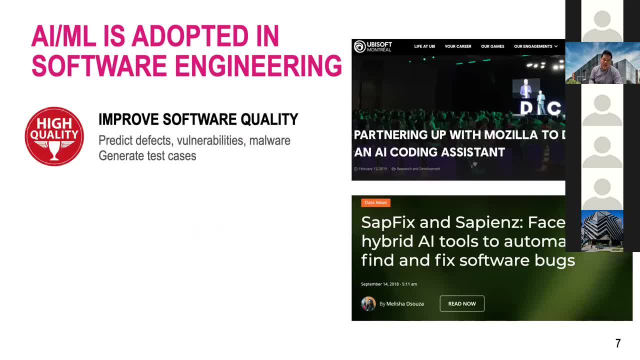 learning, uh, is widely adopted in software engineering and software companies, so in general they can use a, the ai and machine learning to improve the software quality. for example, they can use to predict where the defect is or to predict the vulnerabilities, the malware, or they can also use to generate the test cases as well, like uh and on the. the figure on the right side is some. 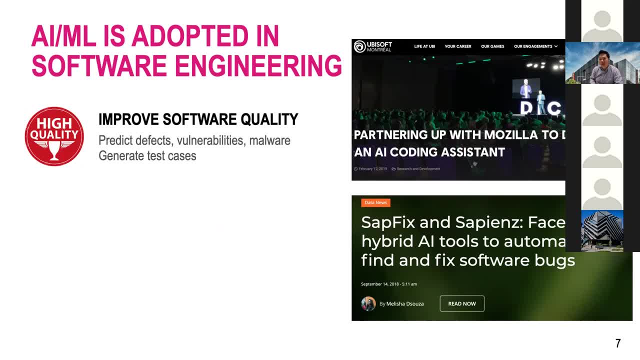 uh example uh successful example uh. for example, ubisoft, uh. integrate the defect predictions into the uh development life cycle to predict bars for every comments, and sapfix and sapiens also adopt the ai tools to find and fix software bugs as well, and the ai and machine learnings can also be used to improve. 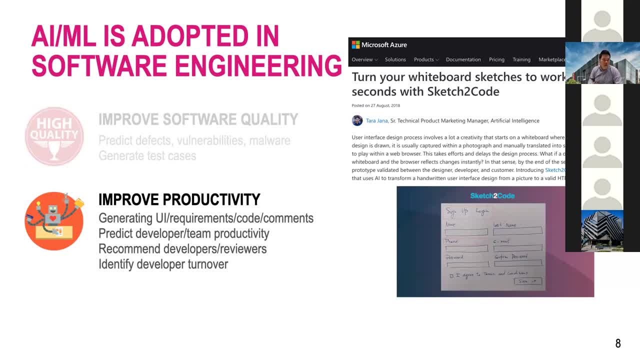 the development productivity, for example, uh. use the like a computer vision technique to generate the ui or generate your ui code requirements, code comments, predict the developer stream productivity. or or use the ai, machine learning, to recommend who should fix this bug, who should review the code, like developer recommendation tasks or the reviewer recommendation tasks. we can also use the ai and 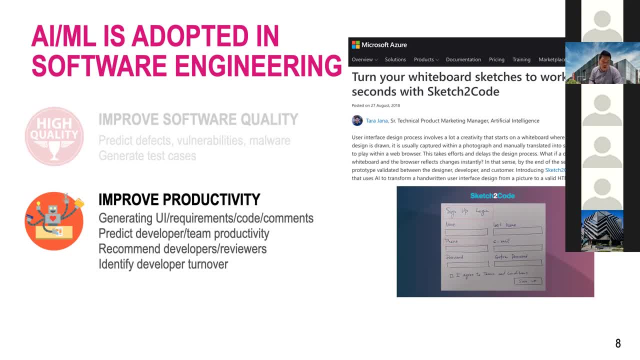 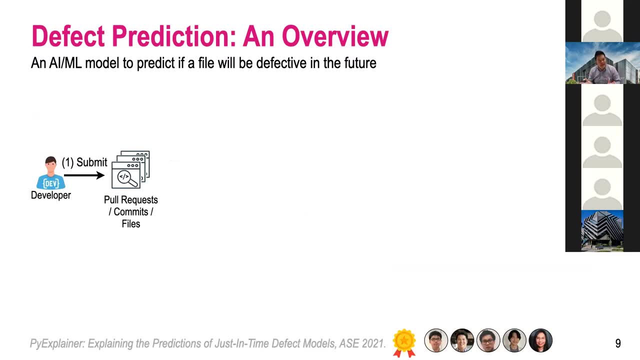 the machine learning to predict or identify who the the developer turnover as well. so there are lots of uh successful uh of the ai, uh, lots of success about the ai and the machine learning in software engineering. but i just want to show and talk a little bit about the. 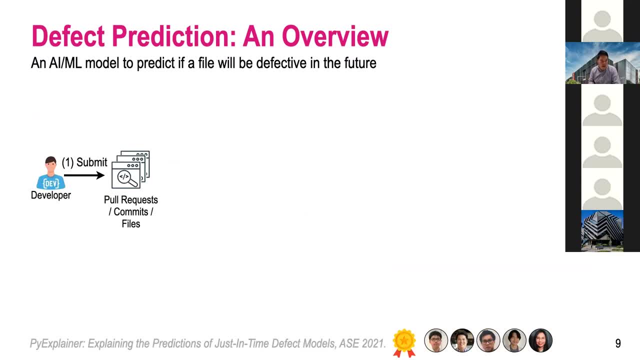 example of the defect prediction, like why it matters. so just to give an overview, what is the defect prediction? anomalies? developers, when you submit a code or pull request to the github repositories, reviewers have to review the code and at and ensure that the the code or the new 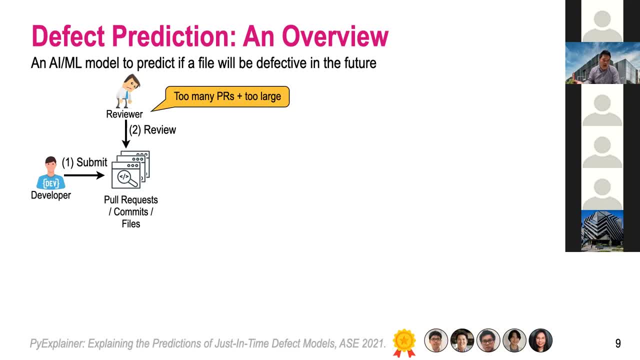 contributions in the pull request are of high quality, so it can be integrated into the software development branch, the master branch. however, the problem is that at the moment, in the large scale, complex software projects, there are too many pull requests, and there are too many and each pull requests are very large as well. then. so the first question for 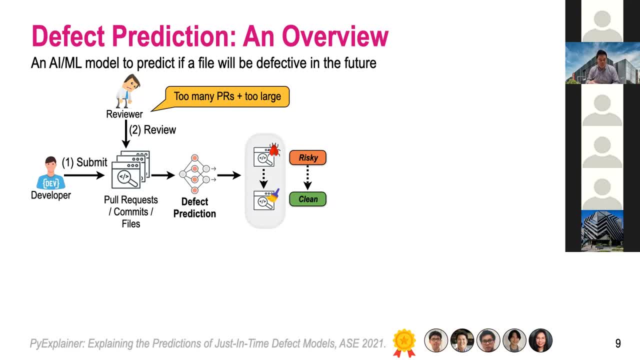 as a reviewer or a tester or QA, is that which pull request that they should look at it first. so that's why defect prediction models, which is an AI or ML model to predict which areas of the course are the most risky or the clean, so they can prioritize the limited QA resources or the most risky one, you know. 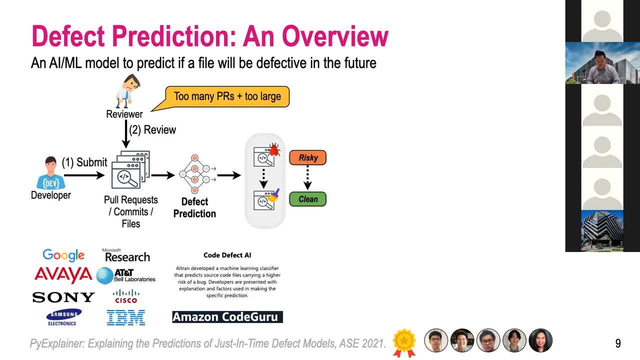 and so far, and the, the concepts of the defect prediction has been proposed for more than 10 or 20 years, and i can see lots of integrations of the different prediction models in many software companies, including google, microsoft, research and the. recently i also see the microsoft. 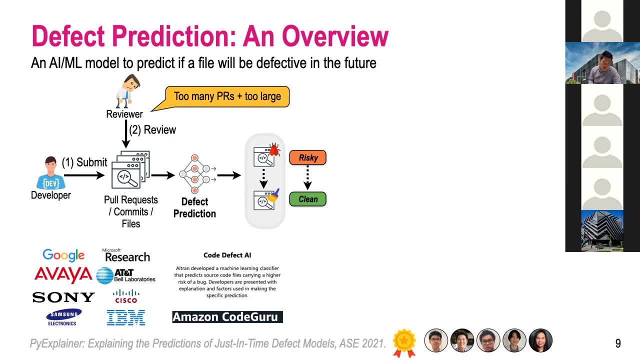 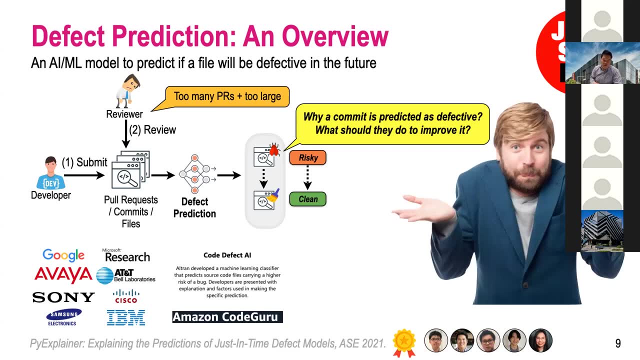 code defect ai, which is a new product from microsoft ai team as well, including the amazon code group. however, most of the time when we talk to practitioners, you know they often ask the questions why a comet is a defect prediction model? and i can see that most of the time when we talk to practitioners you know they often ask the questions: why a comet? 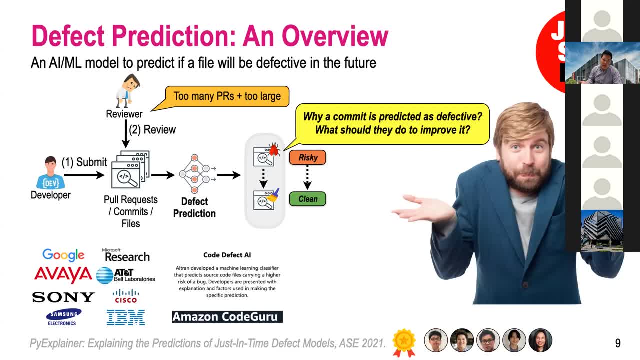 is predicted as defective and why like? why this file is predicted as bug, whether i should trust the, the, the AI or machine learning model or not. and given this file that is predicted as a bug, then they also ask the questions like then how, how should they, how should i improve the? 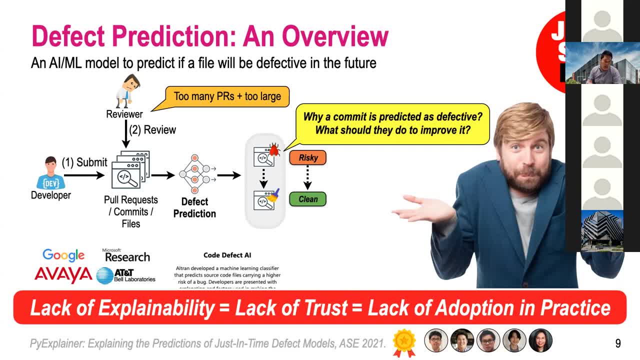 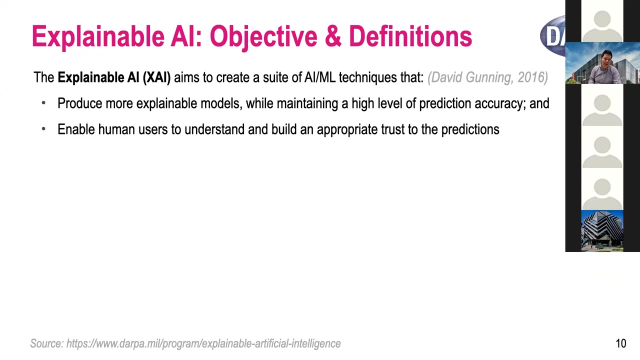 quality of this one right. so there are lots of questions, and a lack of explainability or actionability of the defect prediction models often lead to a lack of trust, which leads to the lack of adoption in practice as well. so that's why the concepts of the explainable AI is emerged recently, and the objective of the 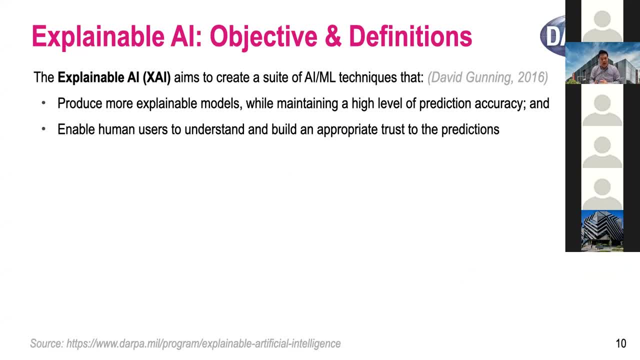 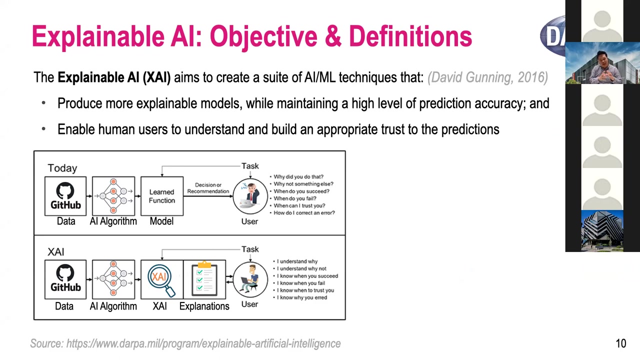 explainable AI is to create a suite of AI and machine learning techniques that produce a more explainable model while maintaining a high levels of prediction accuracy, and it also enables the human users to understand and build an appropriate task to the predictions as well. so i just want to show you an example. like in the past, we have lots of data, the big data from 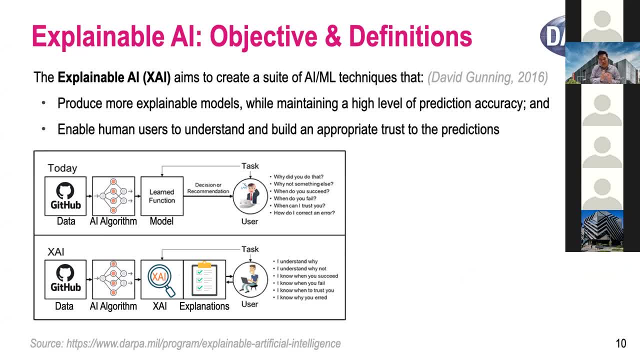 the github, we feed this kind of data into the AI algorithm, we produce the model and then this kind of models- yes, of course it is. it can produce lots of decisions or recommendations to the end users, but most of the time they often ask a question like: why did you do that? why not something else? 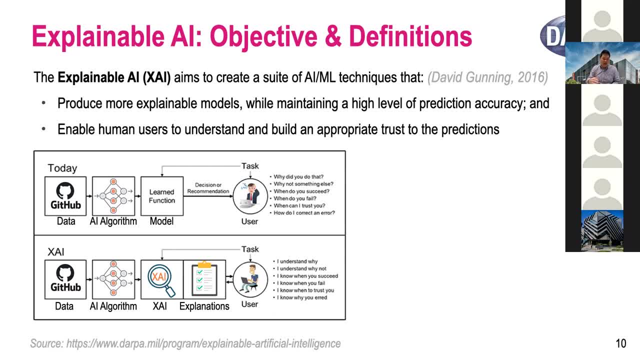 or what to do. right, but what if we can have another kind of technique that is more explainable and then the end users may understand more? like why the model of predictions? okay, so uh, there are lots of confusions in the uh- in the community as well, between the terms. 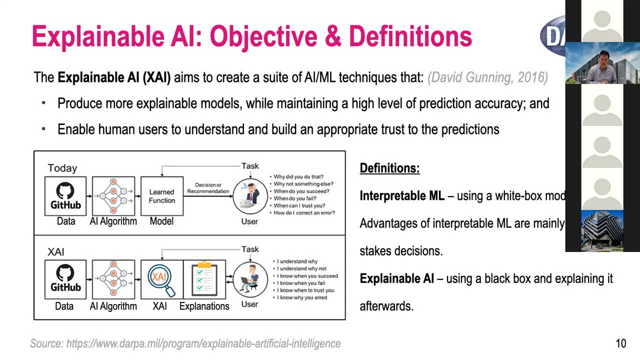 interpretable machine learning and the explainable AI from the common definition. uh, from what? uh, what i graph? uh, from literature survey. they define that the interpretable machine learning. it means that you use a white box model. uh, it's not complex at all, but they are very highly interpretable by. 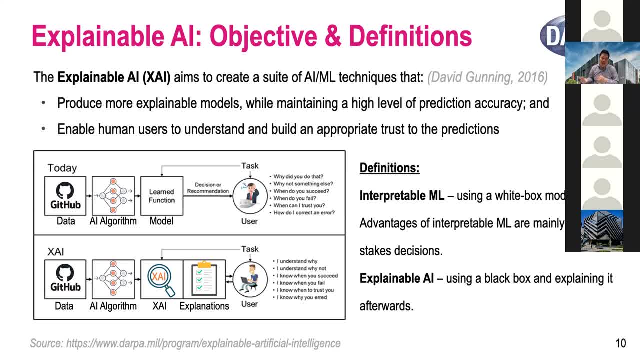 itself, so it should be used for, like a high-stake decision making. these kind of techniques include logistic regression, so they are just a simple mathematics, but they, but you, understand what, uh, what is inside the model and how each decision is derived from the mathematical models. however, uh, these kind of techniques are not that accurate, you know. 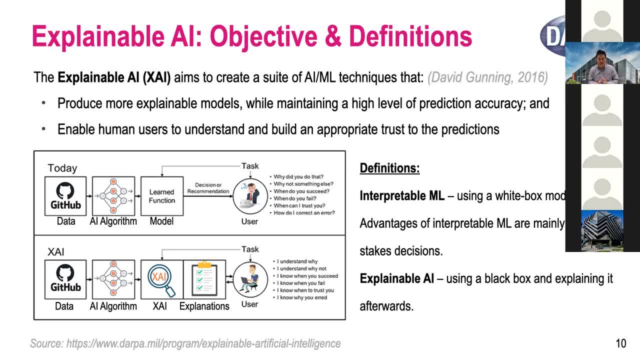 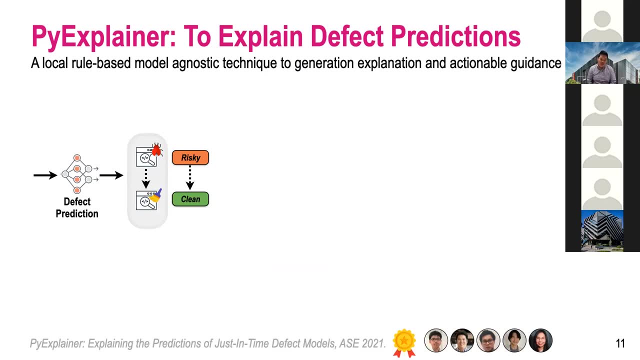 then that's why recently, lots of researchers often use the neural machine learning, deep learning. they are very, very accurate, but they are often treated as black box. then how can you do this? you know, how can we explain them? okay, so that's why we propose a new technique. uh, so it's called pi. 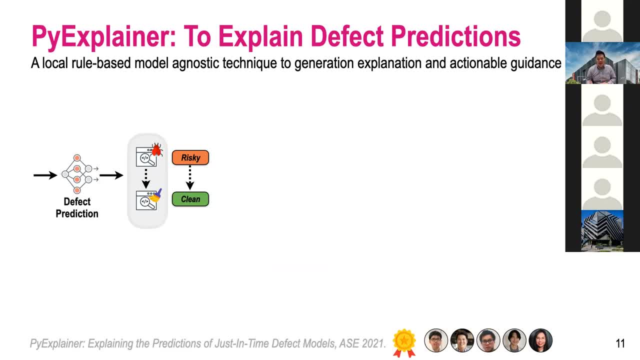 explainer. we uh this paper is published at the ase conference and also received the uh acm six of distinguished paper award as well. so this technique, uh, the, the definition of this work, uh of this technique is called, is a local rule-based model agnostic technique to generate. 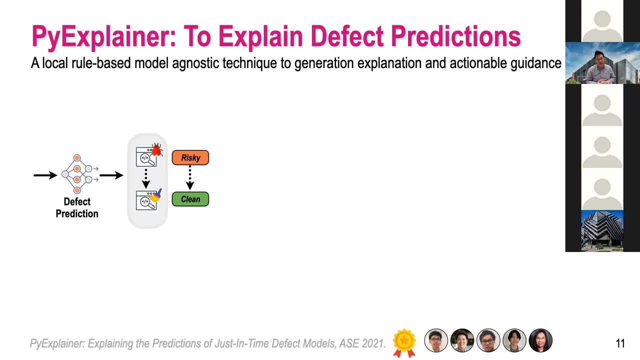 the explanation and the actionable guidance. that's the main goal. okay, in the past, in the field- uh, in the earlier slides we already mentioned that the defect prediction models are not expendable at all, and then i'm gonna show you how to make it more expendable and how can we generate the actionable guidance to the developers. okay, 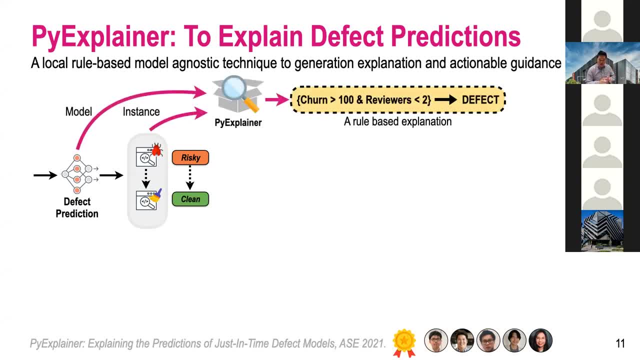 so, given the defect model, this, uh. so next i am going to show you how it works, given the defect prediction models normally, and the instance to be explained, or file, or commit. so basically we just take these two input into the pi explainer and the pi explainer will generate the rule-based explanation, for example. this is an example output. 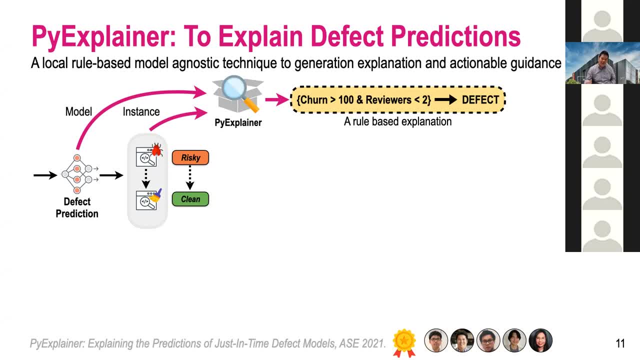 if churn. so like this one, churn is greater than 100 and reviewers less than 2 is associated with the defect. so it means that this kind of rule-based explanation is used to answer the question why a commit is, uh, predicted as defective. so this one is pretty as defect, pretty as defective because 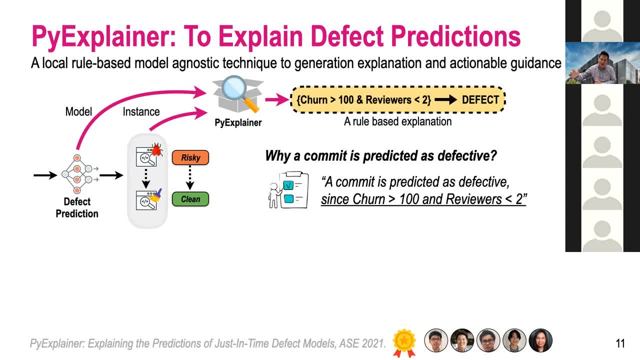 the churn of this comment is too large, it is greater than 100 and it has less than two reviewers review the code. we will disconnect right. then the developers know, okay, what's wrong, what is the most important aspect, okay. so this kind of knowledge is very important to help qa or developers. understand what, uh, what the progress of how we generate the UI, knowledge have developed this thing, uh, what is the most visual significance? and therefore, what сказать maher? to help uh qa or developers understanding what a vast um discussion, stop byDoor Page and help to fund güzel and help to understand what un unDI èto. 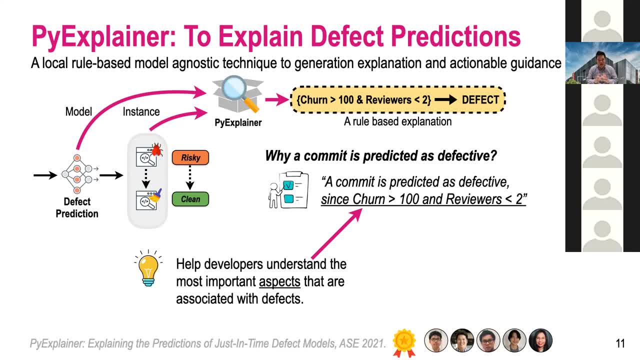 what went wrong with this comment so they can focus on the most important aspect instead of fixing something else? right, and and this kind of rule-based explanation actually goes beyond the traditional feature importance. it doesn't uh, the feature important. just show which feature is the most important, but it doesn't tell you what is the risk threshold, like, uh, how large is large? 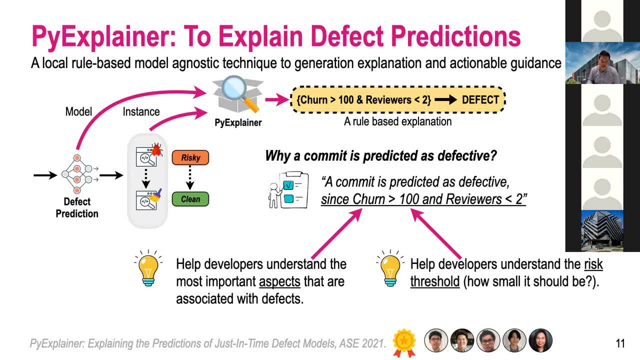 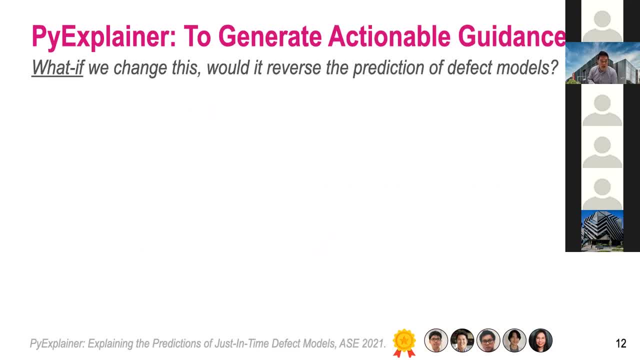 how small it should be, you know. so this kind of rule-based explanation is very useful in this context. okay, and once we know the explanation already, then we also think about, like uh, how can we make the uh explanation more actionable as well? okay, so once we have, uh, this kind of 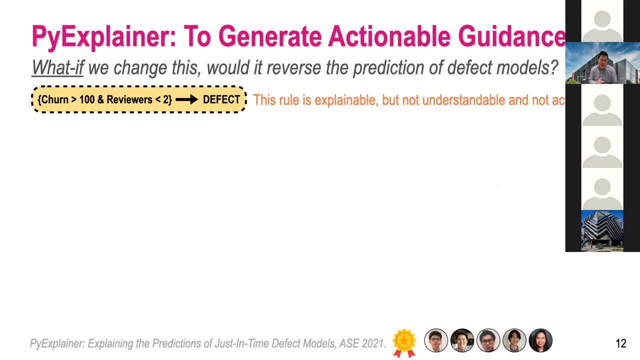 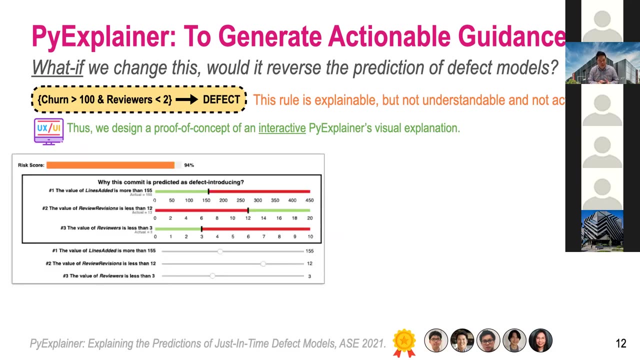 explanation: yes, it is explainable, but it's still not understandable and not actionable yet. so that's why we decide a proof of concepts of the interactive pi explainer, visual explanation, okay, and this is an example, uh, which is going to be in the jupiter notebook, okay, so, given a comet, 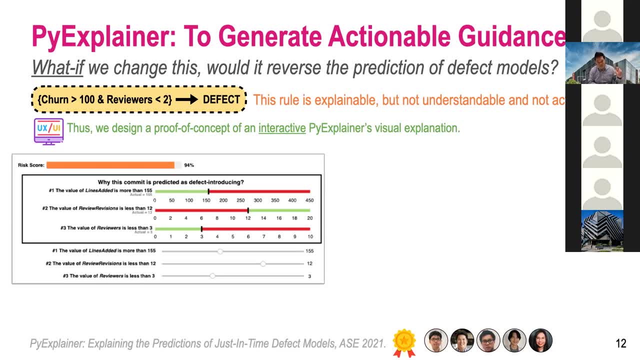 given a model. once we fit these two into the pi explainer, it will tell you what is the risk score, how risky it is, of this comet that will be defective in the future, and it will tell you the explanation. okay, so, uh, the the rules explanation will be translated. 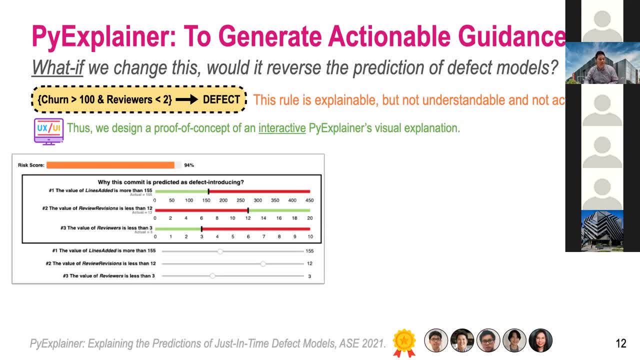 into the slide bar, into the this kind of visual, and it will tell you, yeah, what's wrong. okay, an example of this one is that, for example, the explanation is: the value of the light added is more than uh 155, so that means it should be. uh is too large, so it should be reduced something. 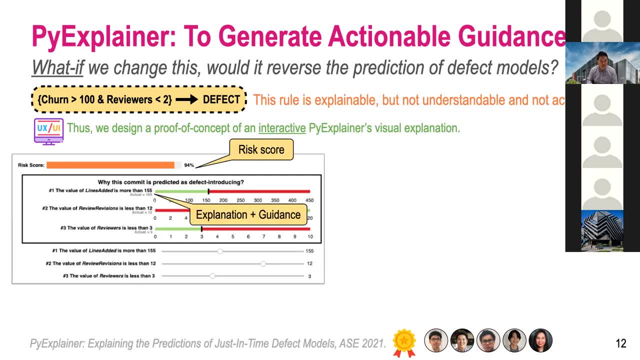 like that. so this is a risk score. this is the explanation and the guidance and the. the cool thing about the the pi explainer is that, uh, the question, um from the developers they often ask the question: what if we change this? would it reverse the prediction or not, right? 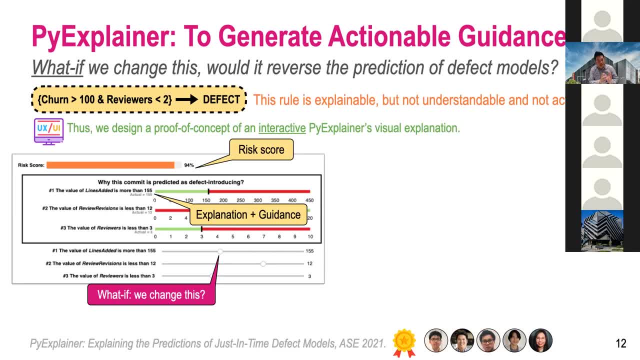 so let's say, if the, the, the, the explanation, the rule here shone- is greater than 100, and then the question: then how small it should be right? uh, what if we change to the 80, to the 70, to the 50? Would it reverse the prediction or not? 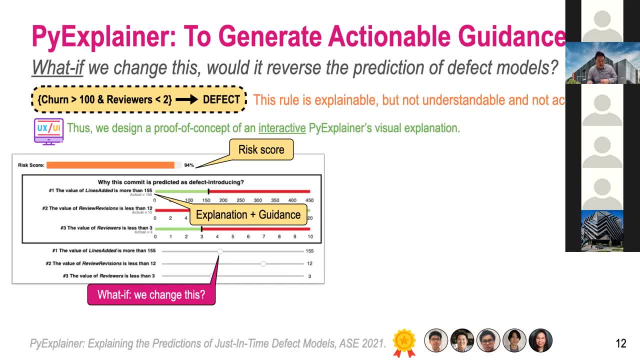 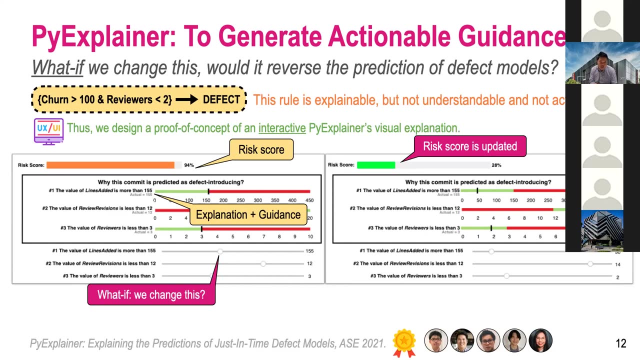 So this kind of interactive visualization. it will help developers make a better decision to identify the appropriate value of that factor. So this kind of tool. if we change the slide bar here, the score will be updated immediately as well from the model So far. anyone has questions? 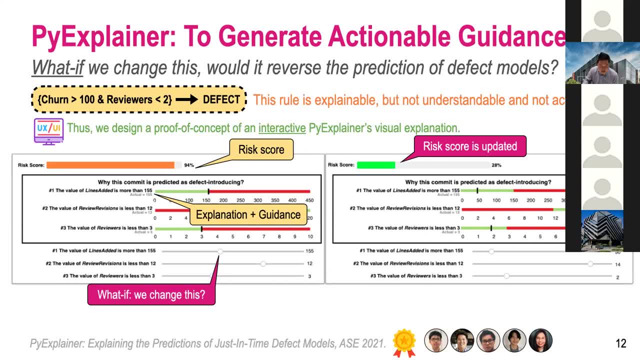 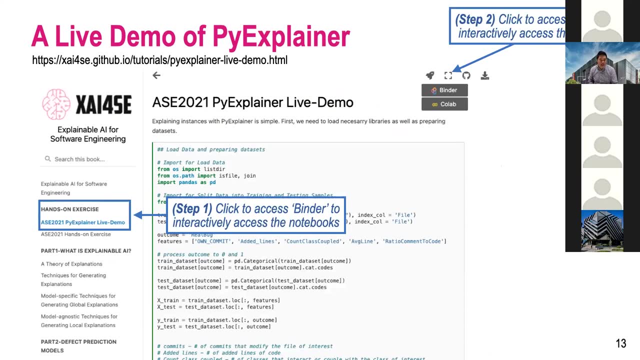 Let me just: Will the slide be available? Yes, it will be available. No more questions Then. next step: I am going to do a live demo of the PyExplainer. So basically, everyone can go to this URL: xai4segithubio slash tutorials, slash PyExplainer- dash live, dash demo dot HTML. 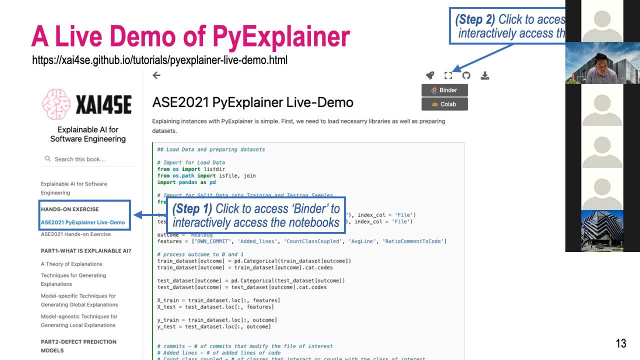 So, Jiraiyut, maybe can you put the link in the Zoom chat so everyone can access as well. Thank you, And so if you go to this one and go to the on the left side, there's a menu title: ASE. 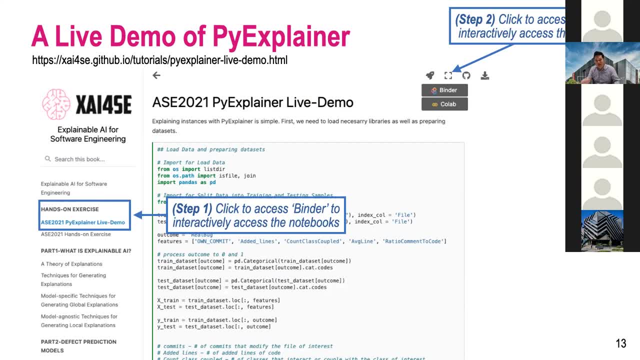 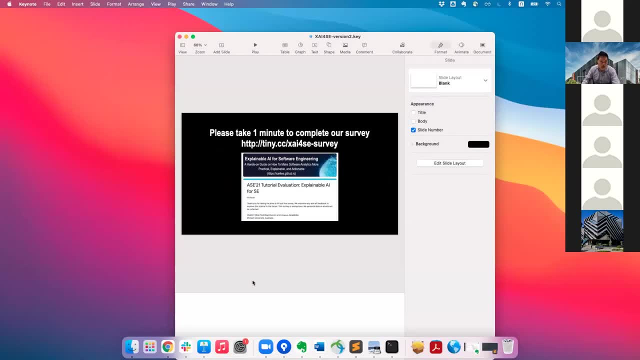 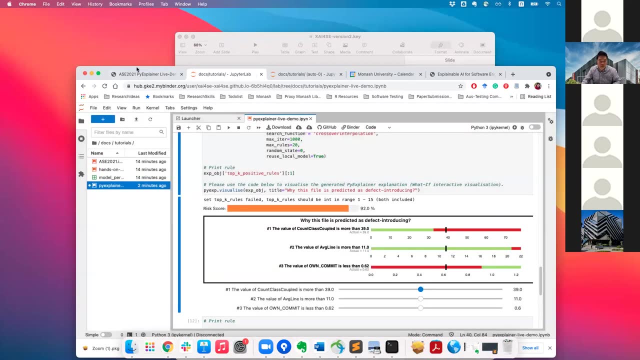 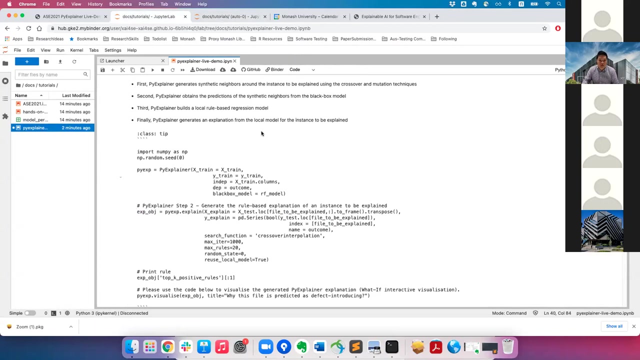 2021.. Okay So if you go to this one PyExplainer live demo, click that one and then you click the binder. Okay So I am going to show you the live demo, the code here. So this is an example. 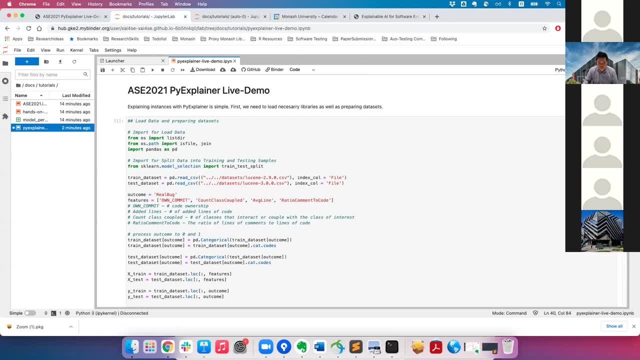 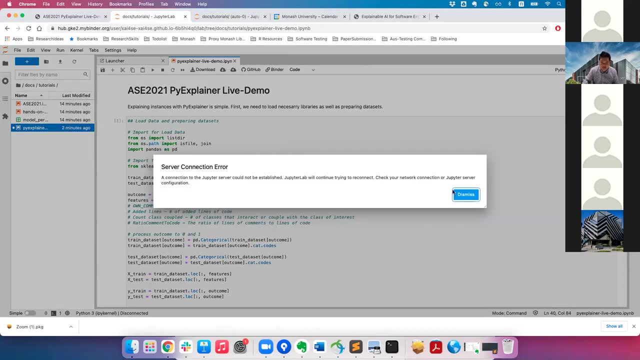 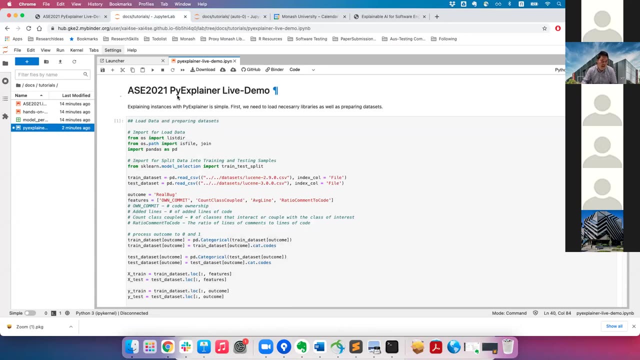 Does everyone see my screen? Yes, Okay, The the- I mean the Jupiter one- Okay, Yes, Okay, Yes, I can see. Yes, Okay, So this is a live demo. Okay, I'm going to explain the concept here. 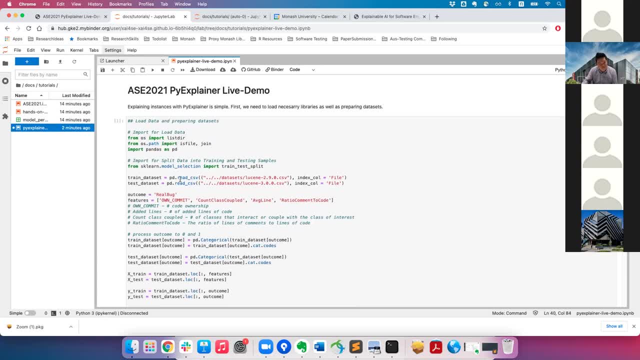 Let's say this is the context of the defect prediction. Let's say we input the trained dataset here, the Lucene 2.90 dot CSV and the test dataset- Okay, the test data here, uh. so that means uh, 2.9. we already know um. 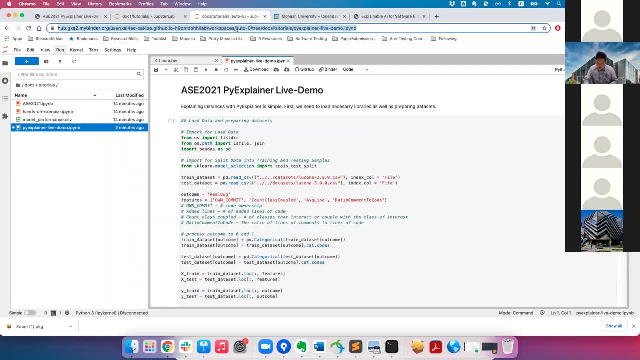 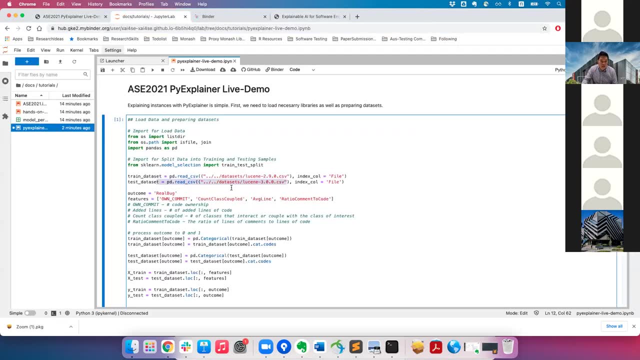 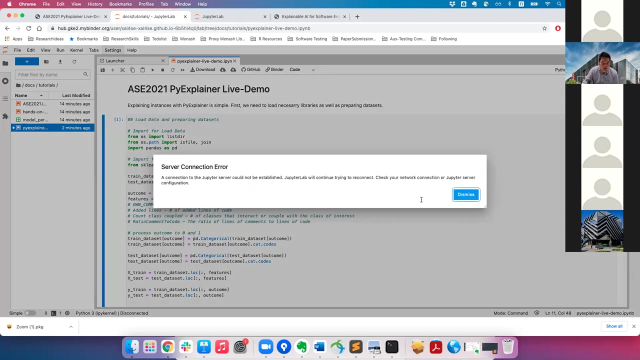 uh, oh, okay, one second. maybe i should run this one again. yep, yep. so we have the training data here, the lucene 2.9.0- uh, that release, and the test version, uh, the, the future one, okay, 3.0.0. and then we already have the, the, the. 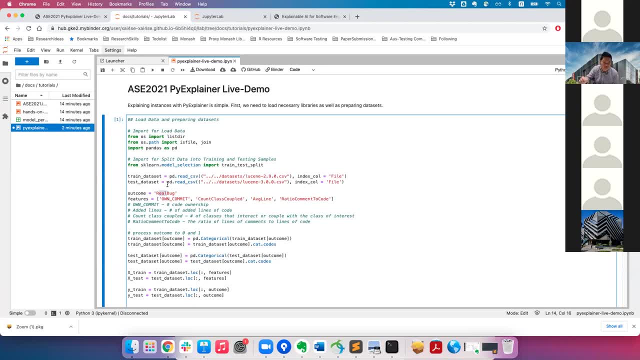 the, the feature that we want to predict whether uh five is a bug or not. uh, and then we also have the predicted feature here. so we use the code ownership, the numbers of class couple, the numbers of average lines and the ratio comment code. this is just an example. in reality you may 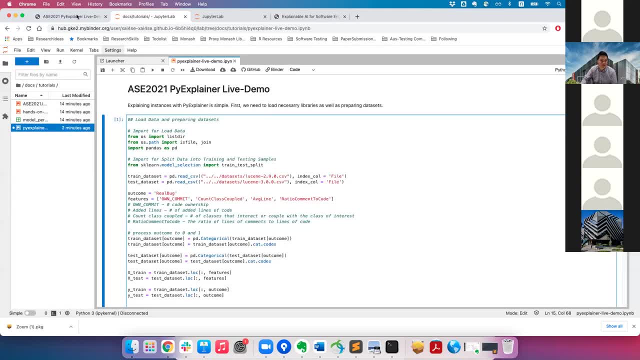 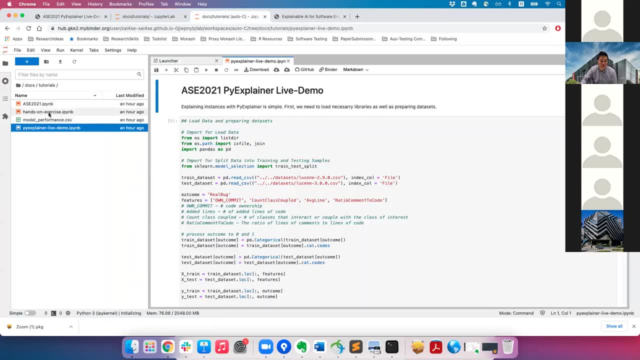 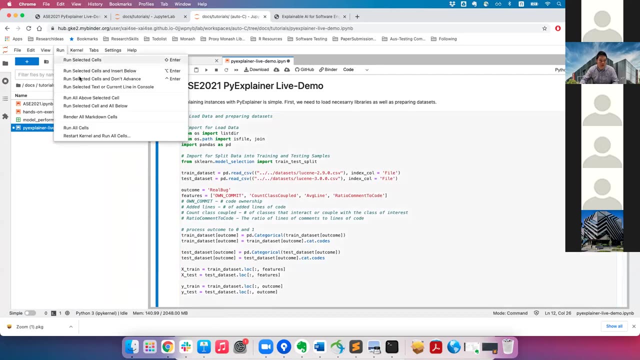 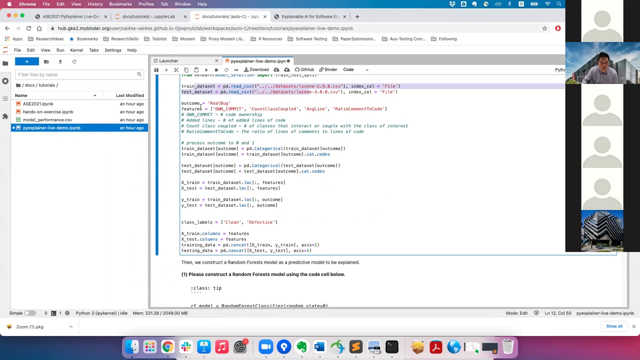 have lots of, lots of uh features. oh, geez, what's wrong? yep, okay, yep, okay, yep. so we already have the, the data set here. uh, we uh define the what, what, what, which columns are the outcome that we want to take and what are the features that we want to use? we pre-process something and let's say, if we are 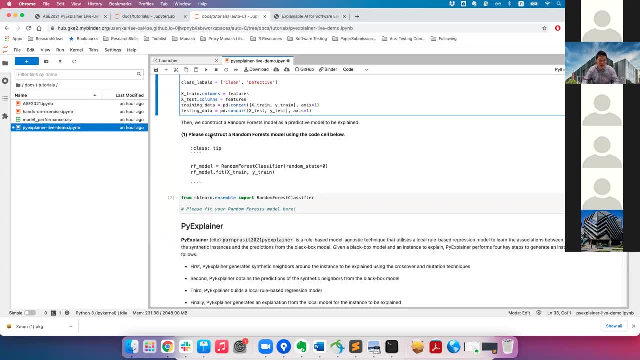 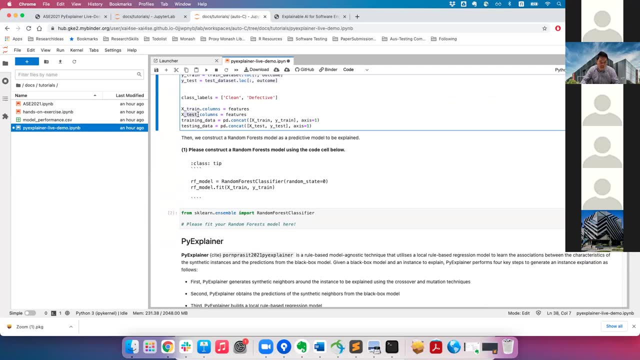 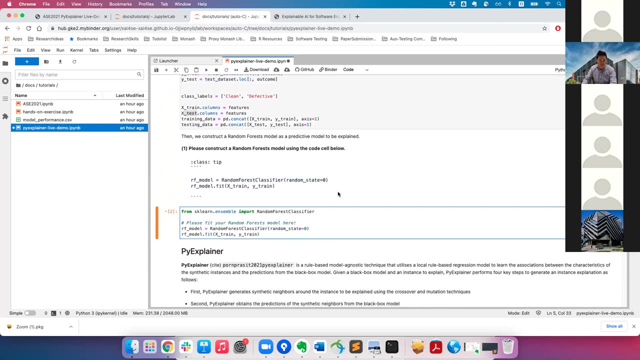 going to build the model. okay, first we are going to construct a random forest model using the code above. we already define what is the training data and the testing data here, so we can try to build the model. everyone, please try to support me if it is going to work or not. 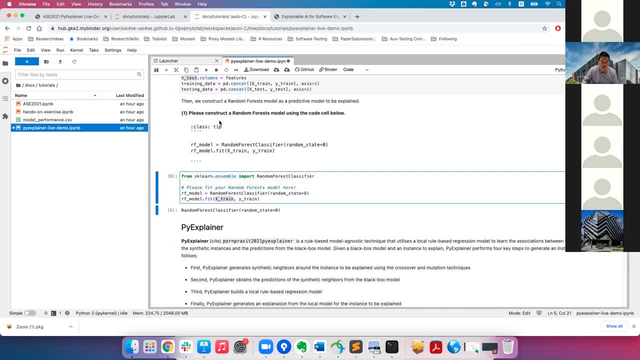 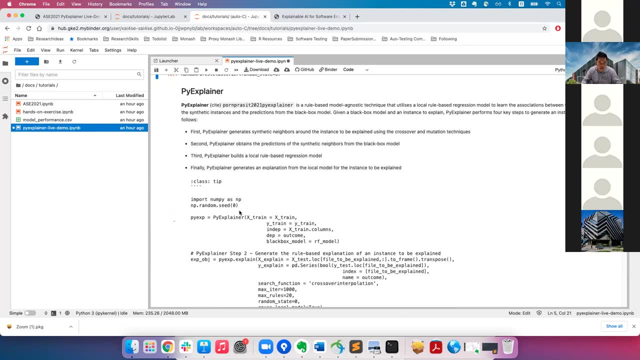 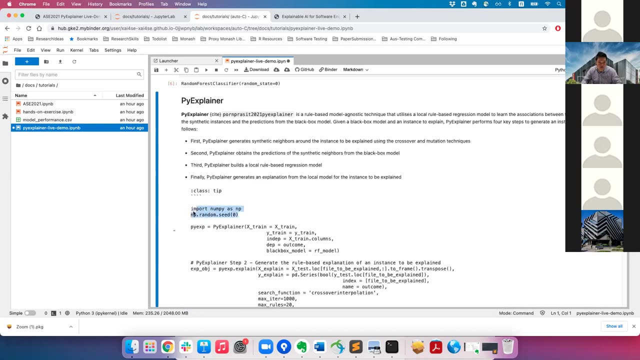 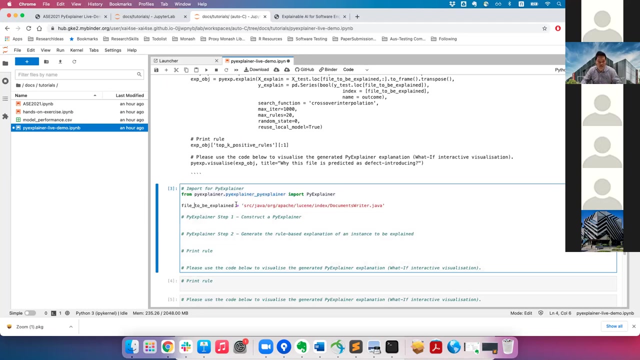 yep. so first we can build the random forex model based on the variables that we already defined, both okay and the concepts of the pi expander. it is very simple. it has only like one or two steps. okay, first we need to define the oh. first we need to import the library- that's very important- and then 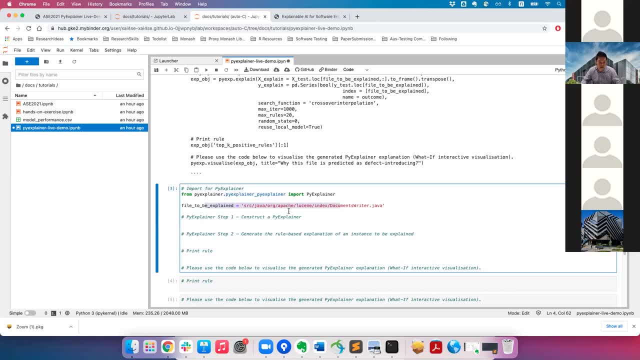 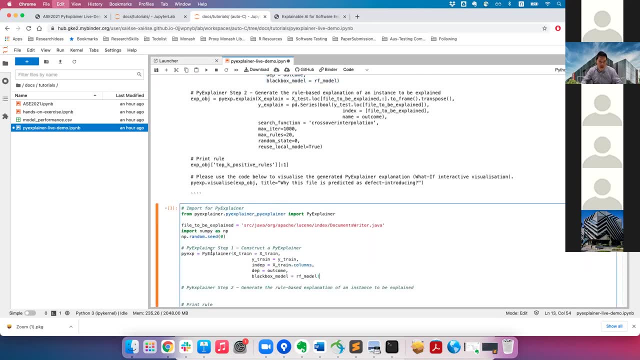 we select what which file that we want to explain. let's say this is an example one. First, we need to build a log-home model from the PyExpander package. The input here should be the training data and which feature the independent variables. 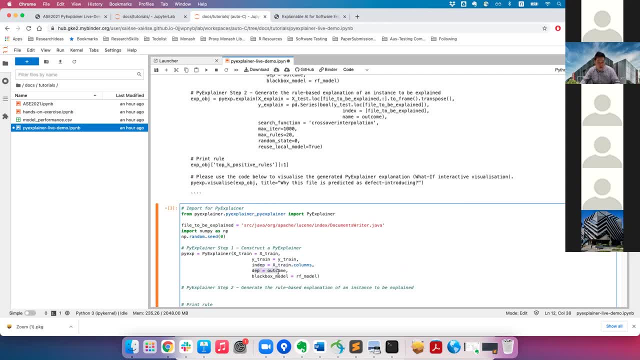 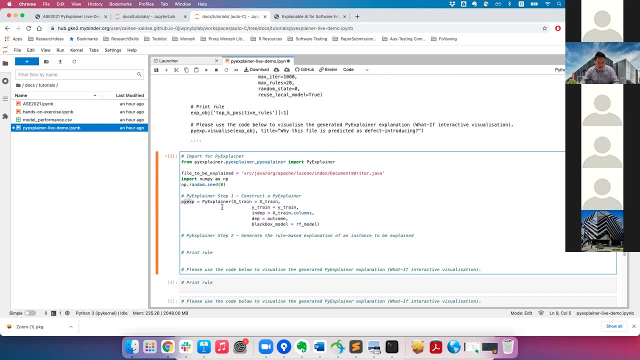 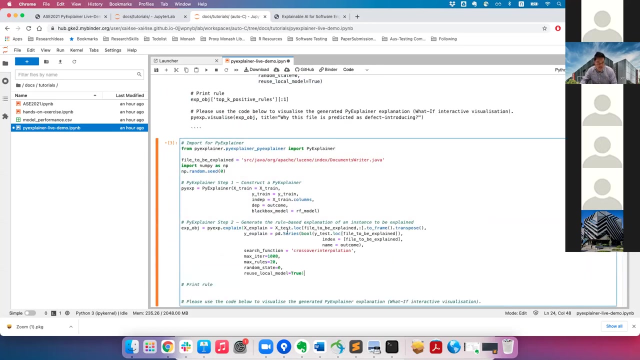 which columns that we want to use as a feature and which column that we are going to use as an outcome that we want to predict? and what is the random forest model? which model? First, we need to build the PyExpander object here, and then the next step is to generate the explanation. 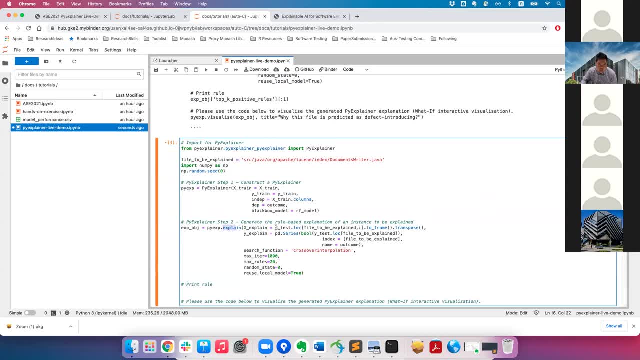 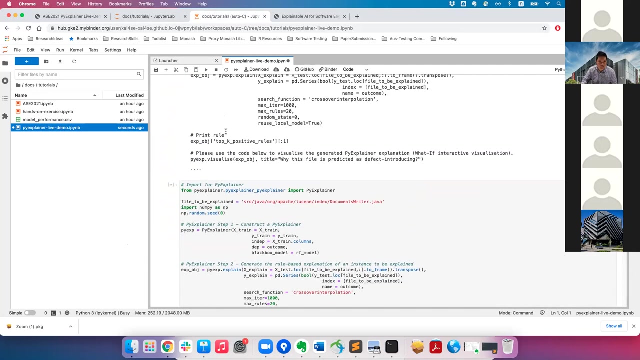 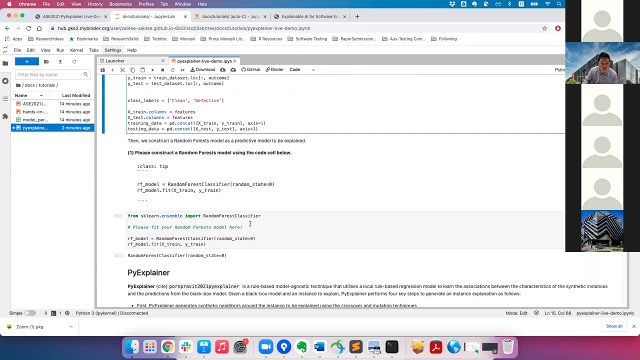 That means we just want to explain this instance, this file, the file to be explained, and we need to define what is the search function, which I am going to explain later, and, some price, All parameters here. So if you run this successfully, it will take some time. 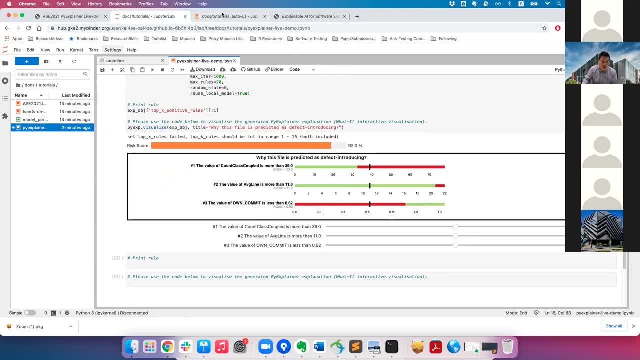 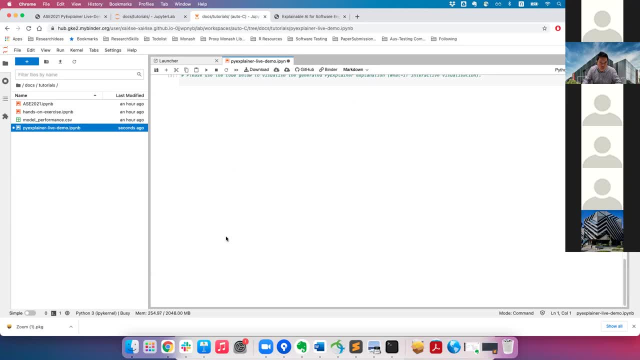 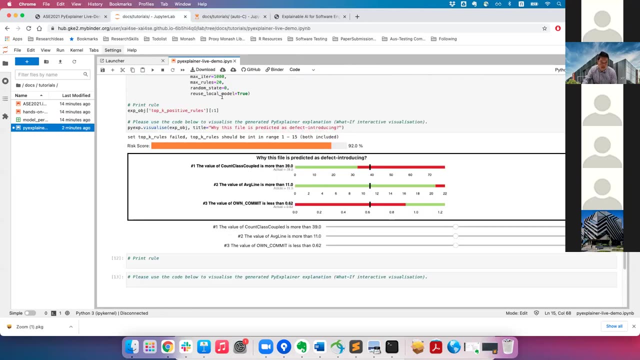 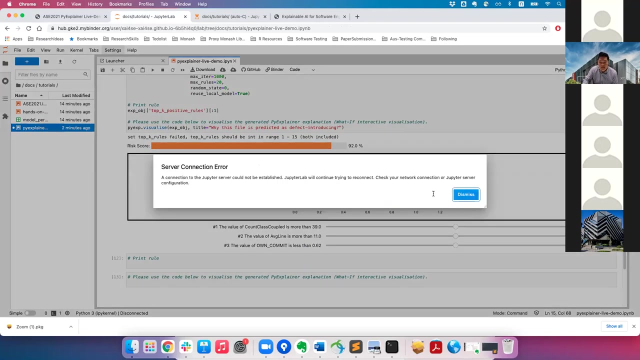 so if it is run successfully. and then the last step: if you run the PyExplainer visualize to visualize the rule here I will go back to this one later. once it is ready It will show you an interactive visualization like this. So that means this phi is predicted as buggy because the 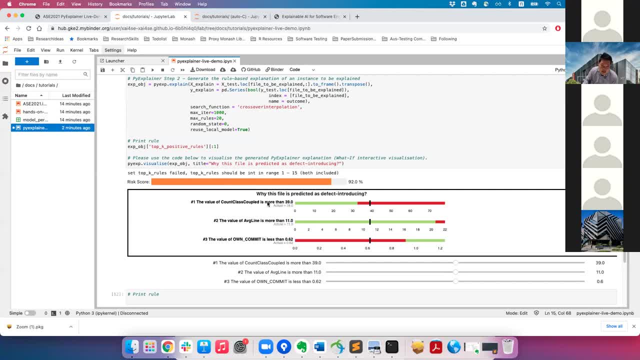 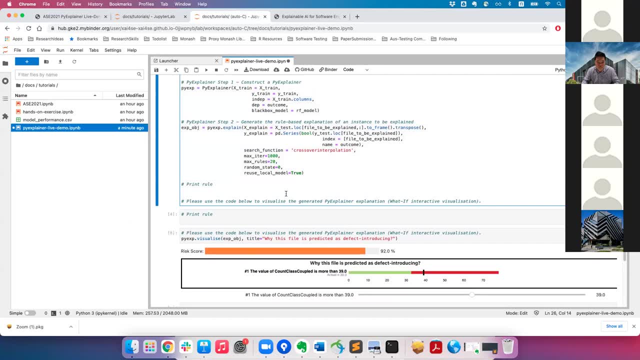 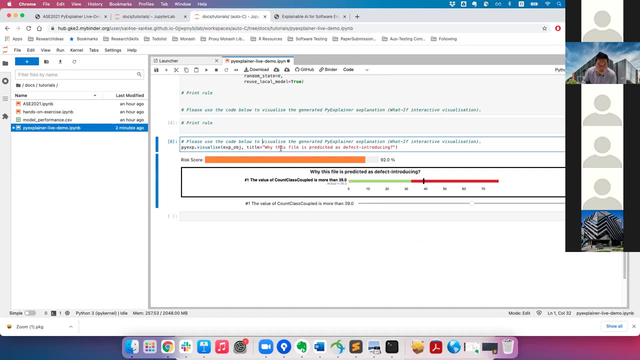 number of class couples is greater than 39.. It is too large, too much, right? Oh, okay, it is here now. That's very good. Let's take a look at this one. So this phi is predicted as buggy because it is greater than 39.. 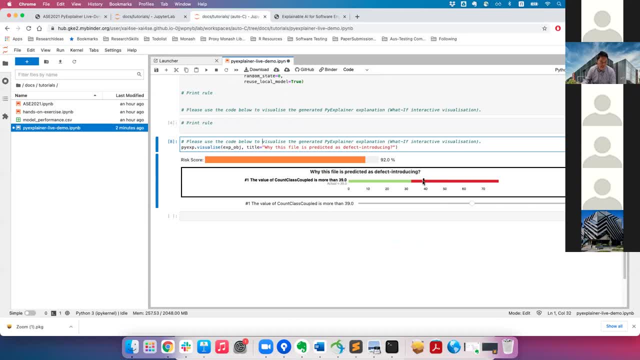 And the PyExplainer. it is a rule-based technique. It also suggests what is the, the value. The value is the risk threshold that it should be right. So I am going to try: what if we change the class couple here to something less than around 30 and see whether the risk score will be? 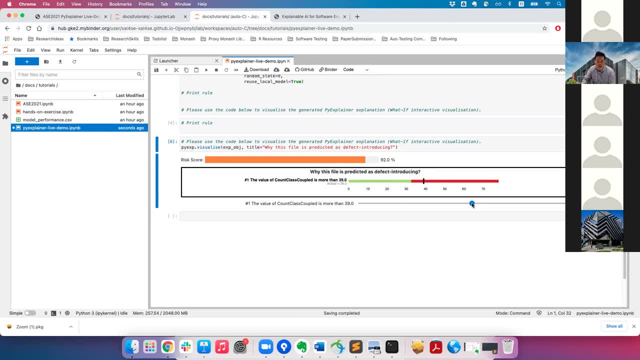 lower or not. right, Let's try. I'm very excited. Okay, Yep, so it works. That means, if we change the value of this, this feature, to the lower one, the model will be. the model will predict that this phi has a lower risk as well. So sometimes this kind of knowledge will guide developers. 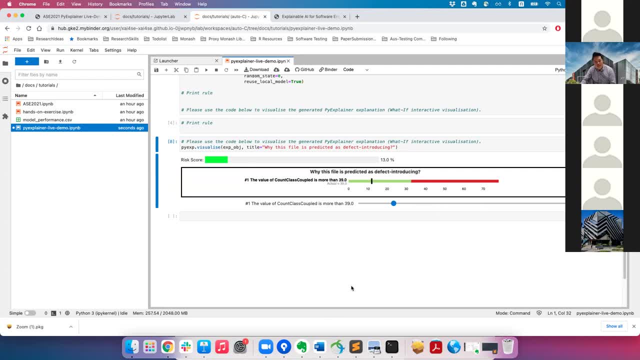 how small that they should change or how they should update the code. Yep, okay, Does the range in these features represent the potential values? The potential values that's taken from this. Yeah, there is a lot of information involved. It just recommend based on the calculation behind it. But at the moment, 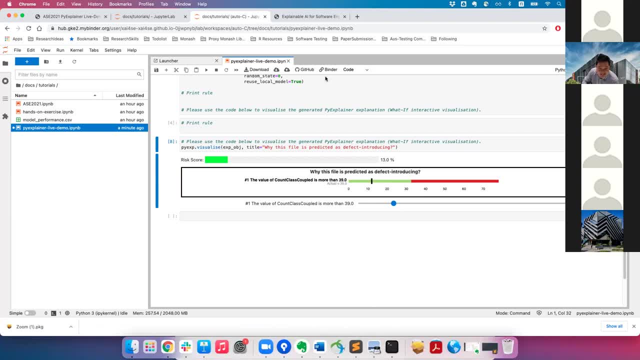 not too sure. Adida, do you want to ask some questions for here? Yes, Can you hear me? Yes, yes, the range in this visualization, you know, the zero to 70, for example, here taken from. can you hear me now? Alright, 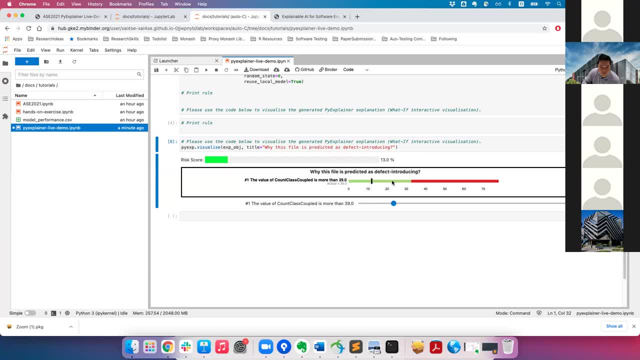 and um. are they specific to a project or general recommendations for where those metrics fall? okay, i see, yep, so you get the right point. uh, uh, thanks, uh for the question. yes, uh, this kind of range is very specific to the file, to the individual prediction, to the instance that we want to explain. 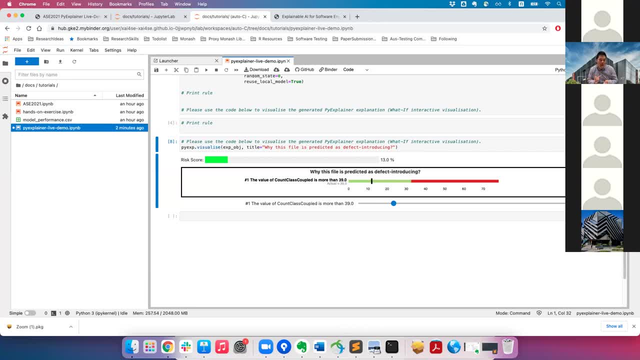 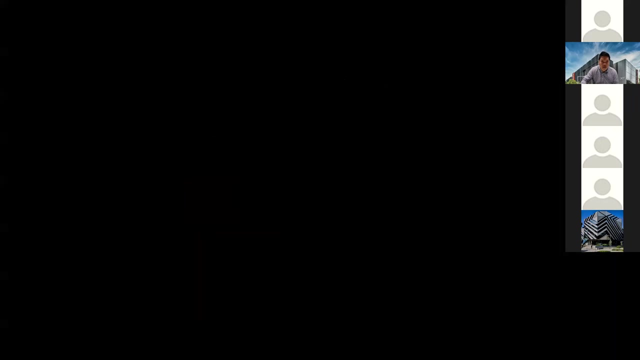 so it will not be a generic uh uh in the most important features like the global level or the model level, yep, so this is a very specific one. all right, uh. so let me go back, uh, to the slide. that's the the pi explainer demo here. yep, so i am going to take some break, let's say two or three minutes. 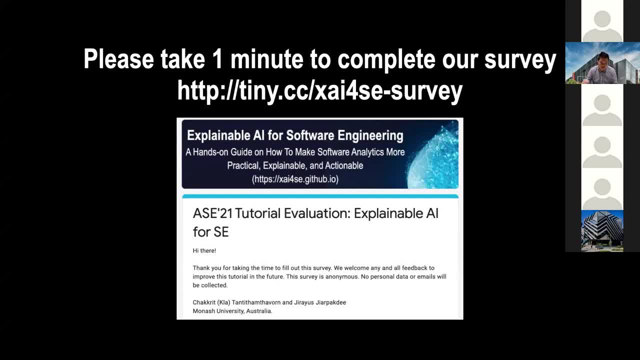 and in the meantime, can you please uh field out, uh the survey as well? uh, for today. and then uh, yep, and then after that i will continue the rest of the tutorial. thank you everyone. i will keep myself muted and in the meantime you can put the questions in. i will answer the next question. 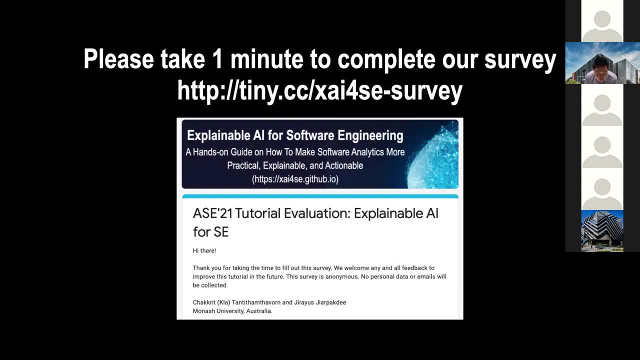 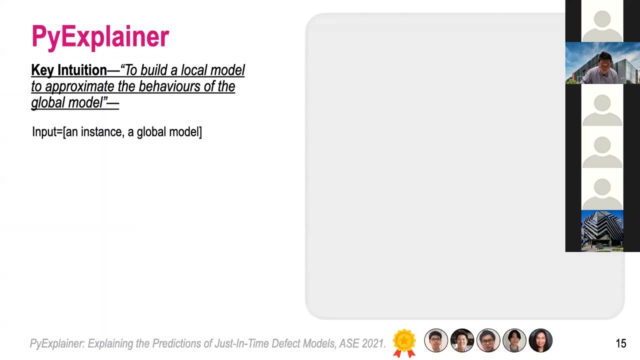 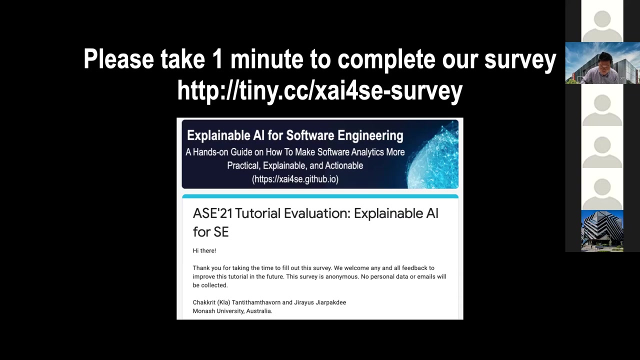 from john andrick. where did the threshold work? where you of 39 come from. so i'm going to explain in the next step. how does the pi explainer work? what is the algorithms inside? what is the key concept? thank you, you, you. Well, everyone, if you have already completed the survey, can you say, like a thumbs up to: 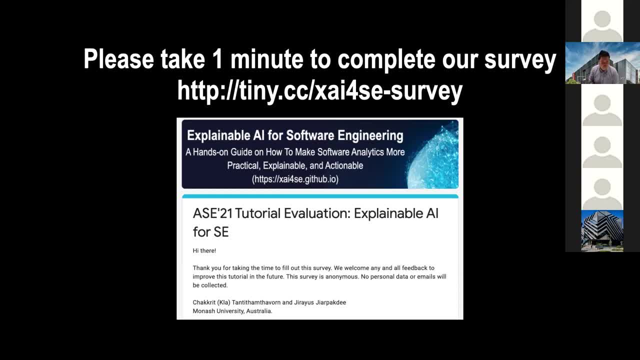 me, so I know that when we should move to the next slide. Hi, Cla, can you perhaps copy and paste the URL for the survey on the chat? Oh, yeah, sure, Jirayut, can you help me? Yep. 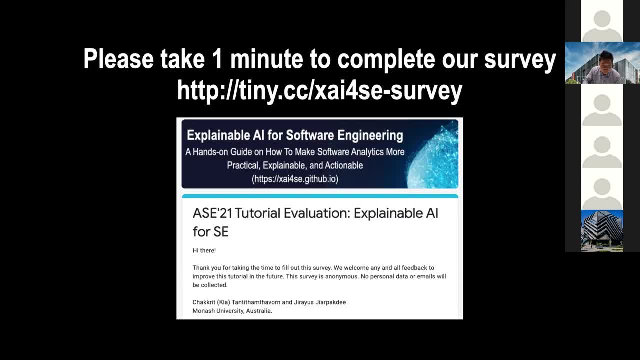 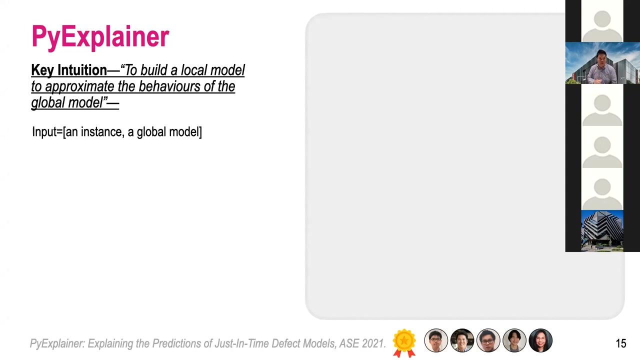 So the URL: tinycc slash AI for it's e dash survey. Okay, All right. Okay, 11.30. now, then I will continue to the next part. Okay, now the next step. I am going to explain what is the PyExplainer. how does it work? 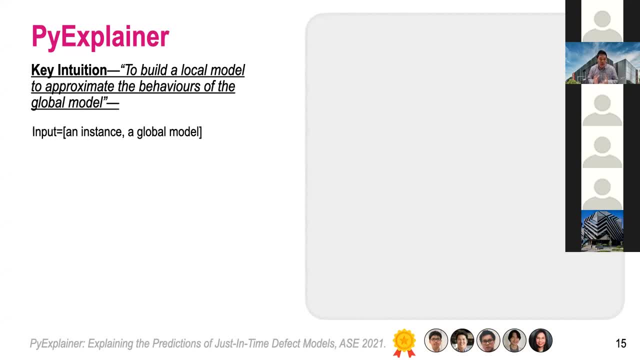 inside. So the key intuition of the PyExplainer is to build a local model to approximate the behaviors of the global model. So normally global model is treated as black box. we don't know how does it work and that's why we need to develop this kind of technique, which is called a model agnostic technique. 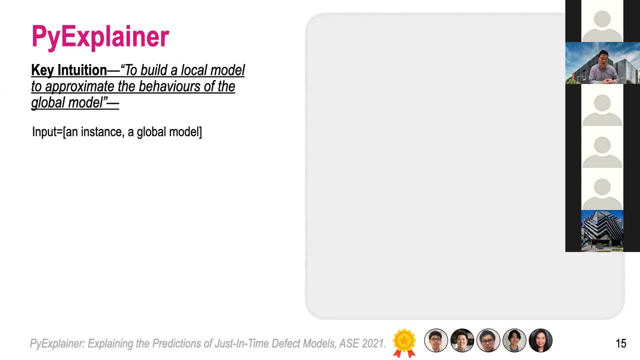 to actually explain the behavior of the global model. That means From the global model. we're going to take two inputs to the PyExplainer. First is the instance that we want to explain and the global model. So the first step, given an instance to be explained, we want to generate the synthetic. 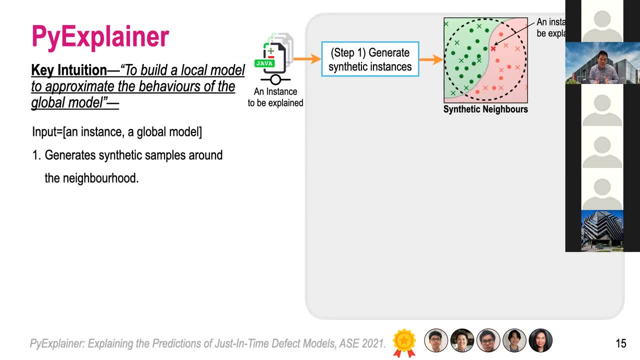 instance around the neighborhood. Let's assume that the X here is an instance to be explained around the decision curve of the model Here. So we're going to randomly generate the neighbors here, the synthetic neighbors, and then we can get the neighborhood here. 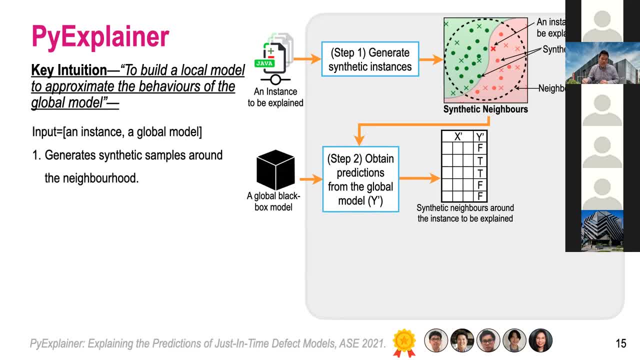 And based on the synthetic neighbors, we're going to input into the global black box model to obtain the prediction. So I'm going to call it YDAT. So that means right now we have the features, the X and the YDAT, the predictions from the 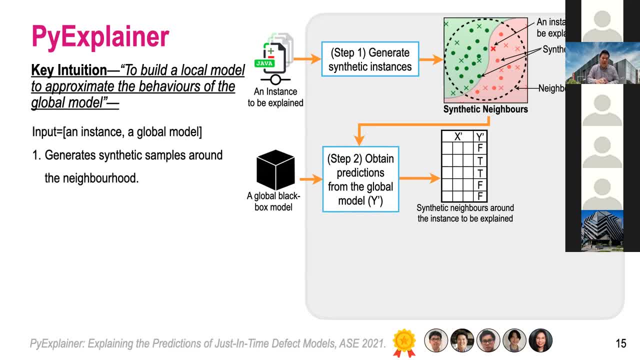 global model for the synthetic neighbors, Because then we already know how the behaviors of the global model. Then we're going to input this kind of data set into the rule fit model. So we choose the rule fit model because it will generate the rules instead of the most. 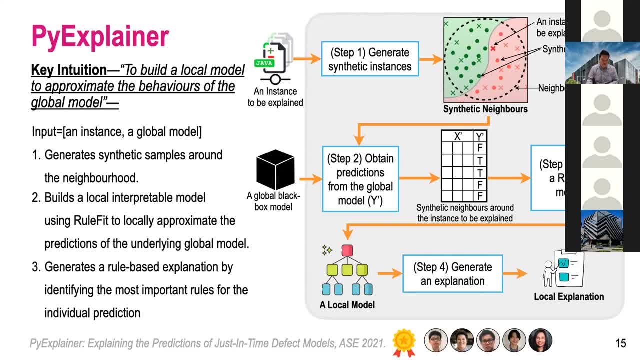 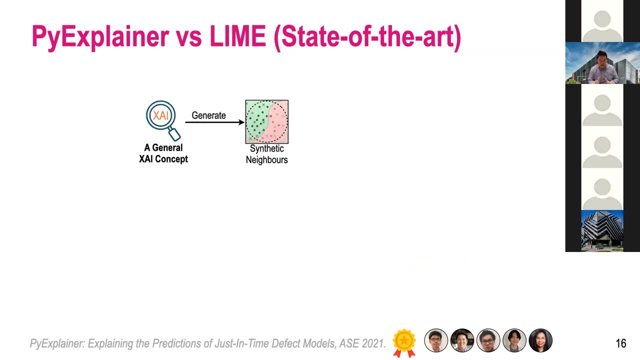 important features. Once we get the rule fit model, then we will extract the rule-based explanation from this model. So the next step I'm going to explain how does it compare with the LAMP approach. So, in general, the general explainable AI concept is to generate the synthetic neighbor. 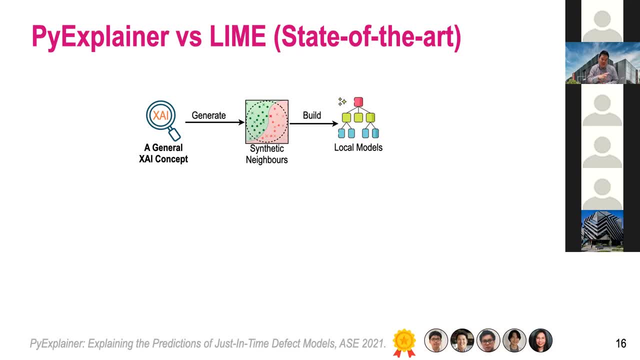 build a local model to approximate the behaviors of the global model And then it will generate the explanation. But the motivation of this work, the problem, is that the quality of the data set is not the best, Because the explanation often relies on the neighborhood that are generated and the local 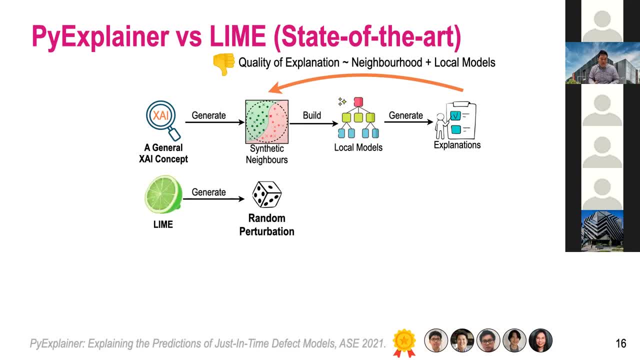 models that are built. OK, LAMP, which is a state of the art approach, And right now it has been cited more than 6,000 papers. They use just a random perturbation, which is not that smart at all. Given an instance to be explained, they just throw random instance. 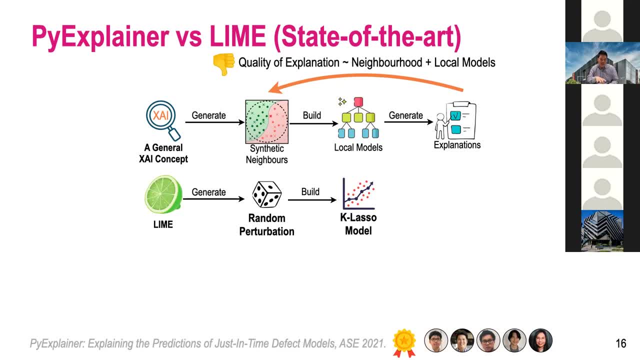 And then they just build a K lasso model based on the random perturbation. And then they just build a K lasso model based on the random perturbation, the random synthetic neighbors, And then they just generate the explanation from this one. But the problem is that when they use the random model, 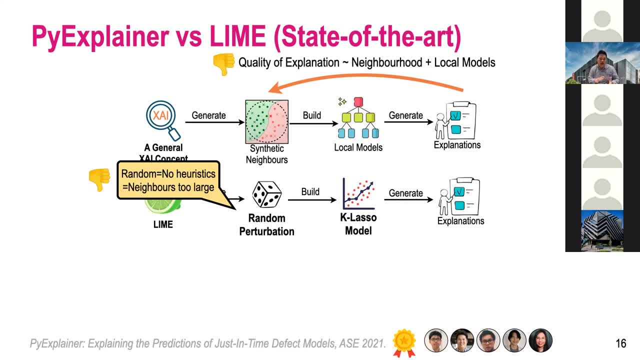 the random techniques. there's no heuristic at all And the neighbors are too large, They are not specific to instance to be explained. So that's why when the neighbors are not of high quality, it will produce an inaccurate model and it will produce the poor approximations. 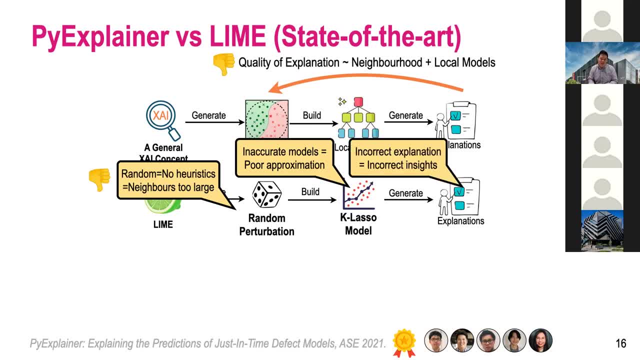 of the instance that we want to explain as well- That's why LAMP is not that effective at all- Then it will produce the incorrect explanation and the incorrect insight. That's the main limitations of the LAMP that we want to raise in this paper. 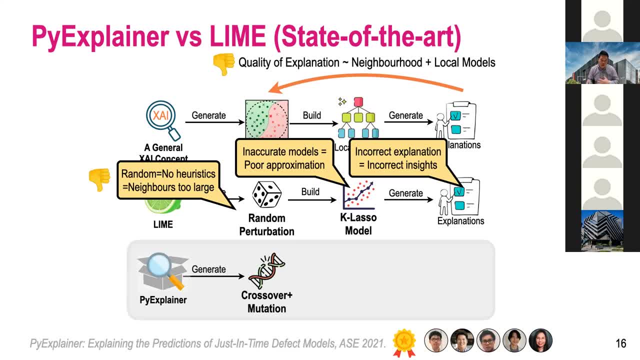 But when compared to our approach, we use the crossover and the mutation to generate the neighbors. That means given in an instance to be explained. we start from the initial random seed, random instance and then we do some crossover using the heuristic of the actual instance. 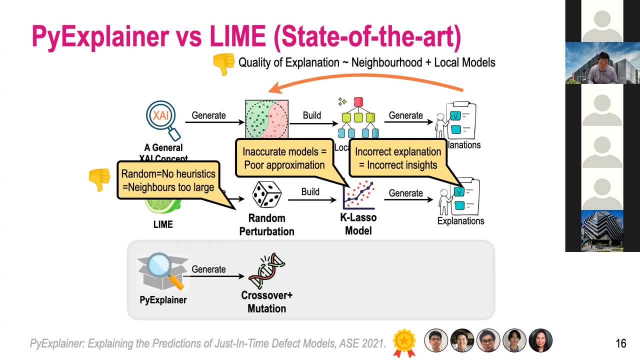 to be explained as well: actual data, And then, once we have a more effective neighbors, then we use the rule fit model to build the local model and then we generate the explanation. That's the key difference. But how can we ensure that the neighbors 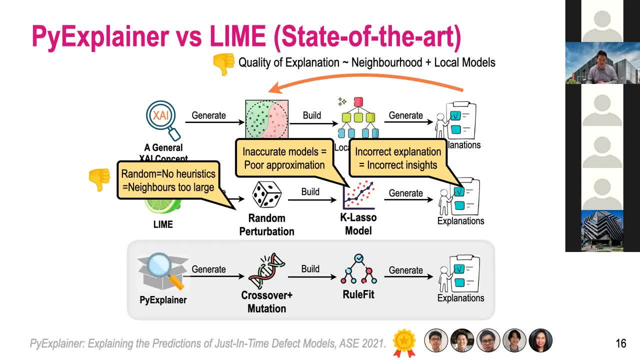 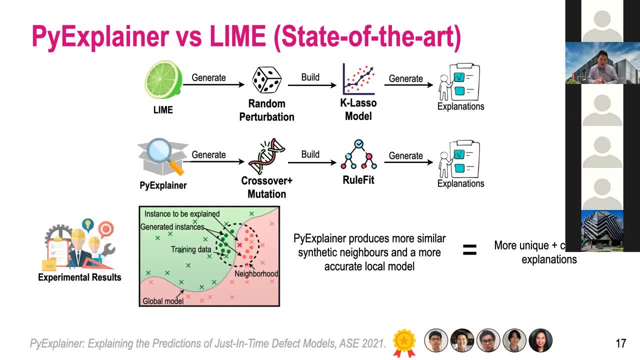 the neighbors that we have is better than LAMP, or the local model is better than LAMP or not. So we conduct an experiment to evaluate the quality of the neighborhood that are produced by PyExplainer when compared to LAMP and the local model. 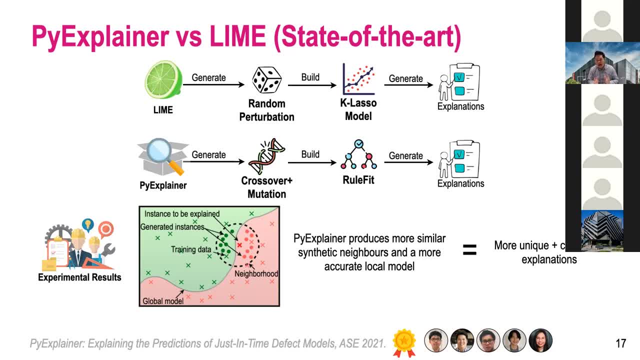 And finally, the results that we found is that PyExplainer produces more similar synthetic neighbors and a more accurate local models when compared to LAMP. So it means that we have a more accurate local model when compared to LAMP. So it means that our approach actually produces more unique. 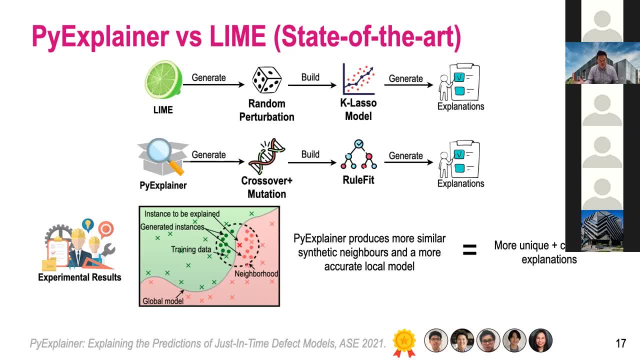 and more consistent explanation as well. So that's the key concepts of the PyExplainer. Okay, I'm gonna pause a little one or two minutes to answer some questions, if you have Yep Now. so Yi-cheng has a question. 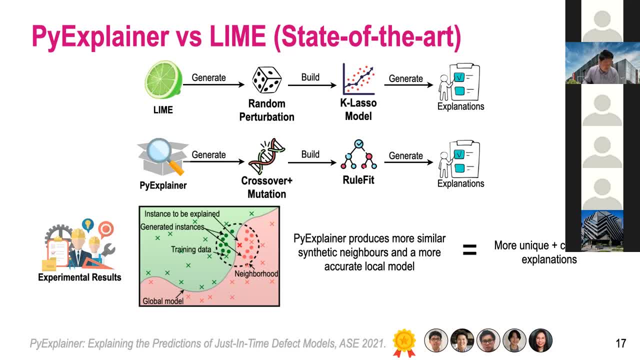 What is the difference of concepts of the local model and the global model? That's a good question. Okay, So the global model is the model that we train from the whole data set, and most of the global models are very complex. they are built from deep learning. they are not understandable. 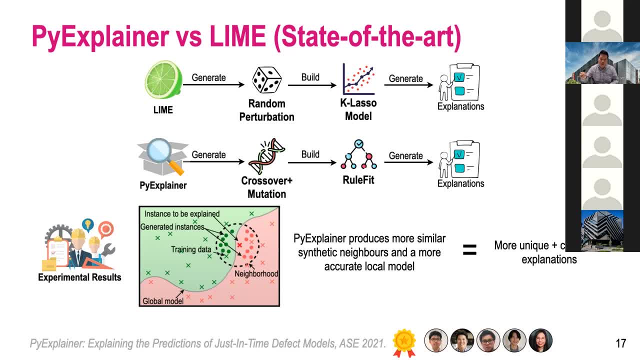 at all. So that's why we need to build a local model to approximate the behaviors of the global model, and the local model will be more interpretable than the global models. That's the concept. Am I answering your question? Yes, thank you. 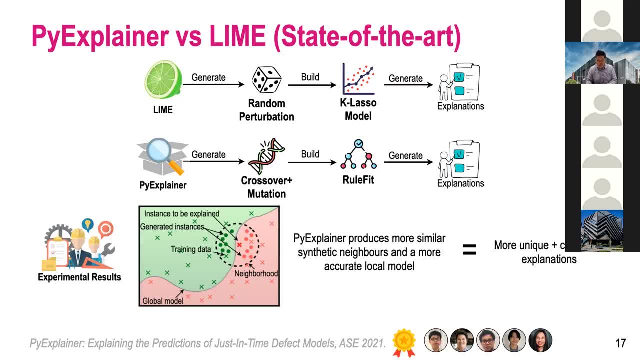 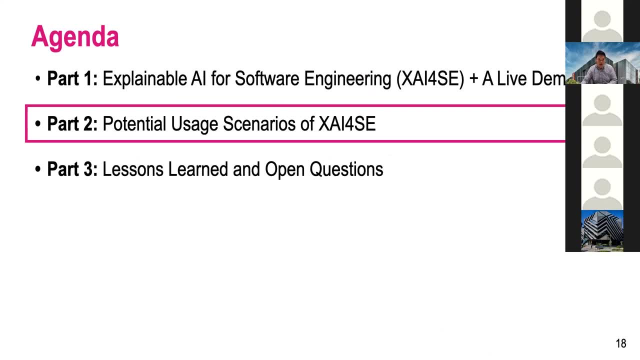 Okay, all right, then I am going to move to the next part of the tutorial. Okay, the next part I'm. I already saw In the part two, I'm going to show you how to build a global model. Okay, the next part I'm. I already saw. 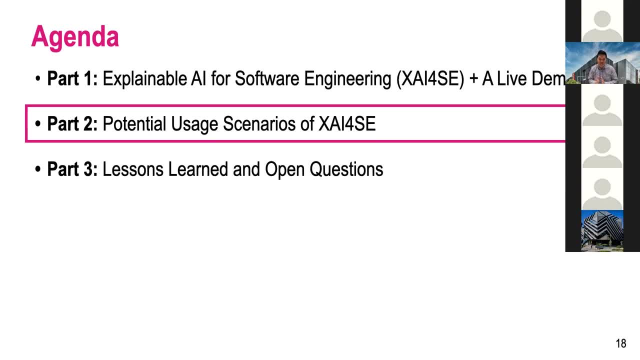 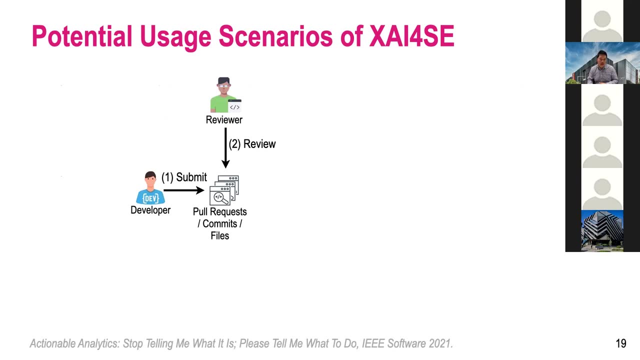 In the part one, I already talked about the concepts of the expandable AI for software engineering, and the next part I'm going to talk about what are the other potential usage scenarios of this area. okay, So, as I mentioned again, developers submit lots of pull requests and reviewers they 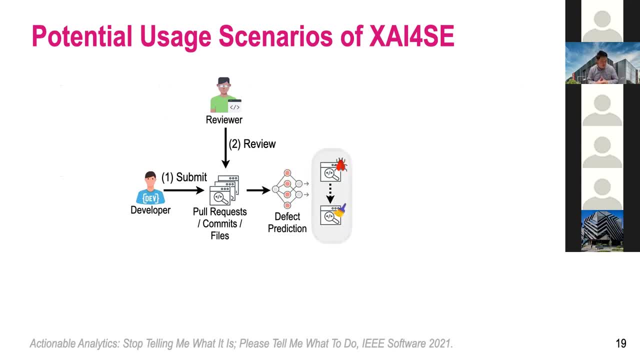 have to review the code, but they don't know. but there are too many pull requests, commits and files. how can we better allocate the limited resources? So different prediction models are built and what I am going to say is that expandable. 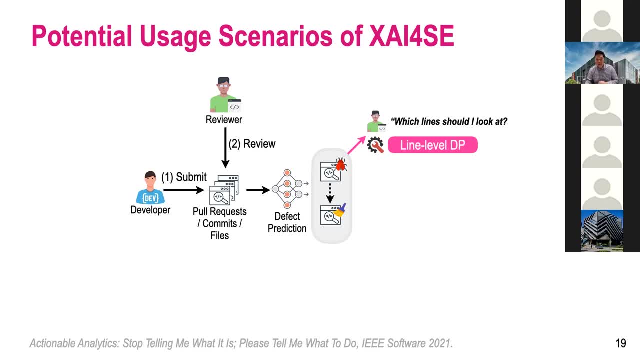 AI is not just only to generate the explanation, but it can be used to identify which lies that they should look for as well. So it's called lie-level defect prediction, And this is what I already mentioned- why it is predicted as risky- and to generate 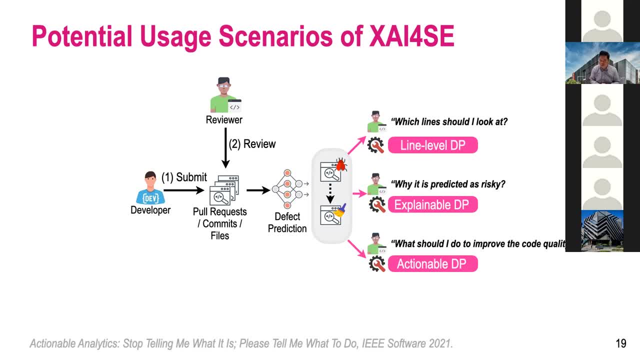 the actionable guidance. What should I do? What should I do to improve the code quality? So what I'm going to say is that in this presentation, I'm going to focus on the three aspects: How can we make the prediction models more practical, more expandable and more actionable? 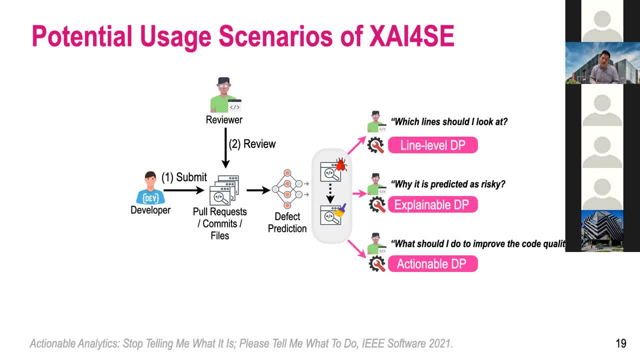 And, in terms of the explanation, we can focus. we can generate, like which features are the most important, but we can also generate which lies are the most important And, in terms of the explanation, we can also generate which lies are the most important. 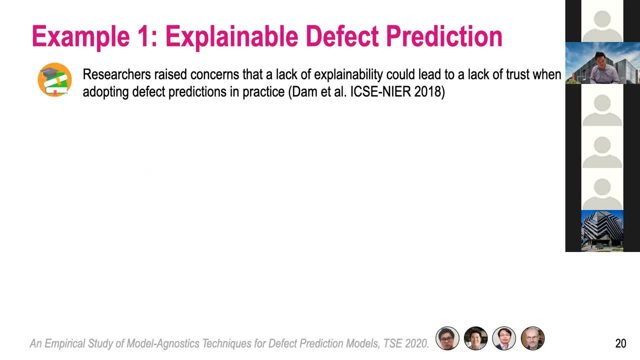 but we can also generate which lies are the most important. but we can also generate which lies are the most important. but we can also generate which lies are the most important or contribute to the predictions as buggy as well. Okay, In the earlier presentation I already talked about that. the applied explainer can be used. 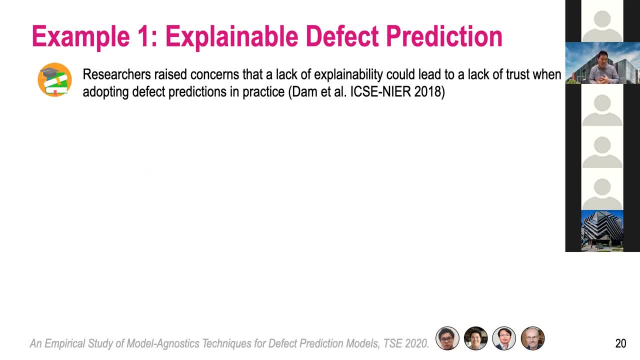 to explain the model, but there are lots of types of explanation as well. How can we maximize the benefits of the expandable defect prediction? Okay, So maybe I'll just talk about the motivation. Okay, So maybe I'll just talk about the motivation. 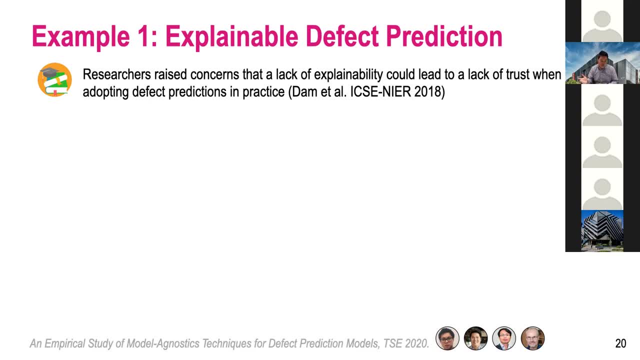 So maybe I'll just talk a little bit. Researcher, I mean in 2018, Hua Damatoff from Wulongong. he raised concerns that a lack of explainability could lead to a lack of trust when adopting defect predictions. 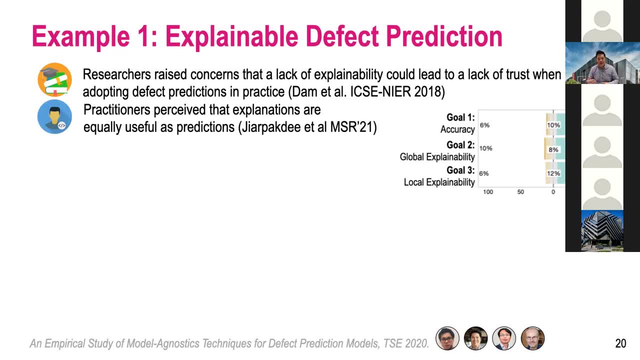 in practice And in our recent study we ran a survey with practitioners to identify what do they perceive about the goals of the defect prediction studies And we first do the literature review to identify what are the goals. and we found there are three common goals. First is to improve the accuracy, to generate the explanation And, surprisingly, 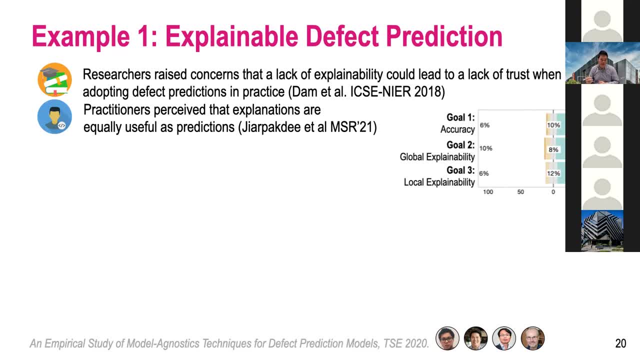 what we found is that practitioners often perceive that explanations are equally useful as improving the predictions. But the challenge is that most of the machine learning based defect models are globally explained, but they are not locally explainable yet. And then the global explanation is often derived from the historical data, but they may not be applicable to the unseen. 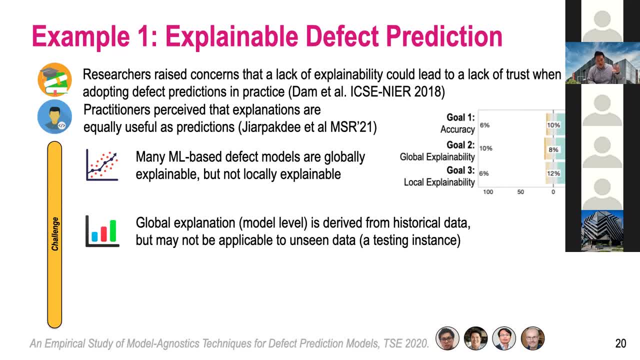 data. So just to illustrate again, you have a data set, you build a model, you accept the feature importance, that's, the knowledge or insight that is derived from the model, but not the unseen data. That's why we need a new technique, new concept to make the defect prediction models more explainable. 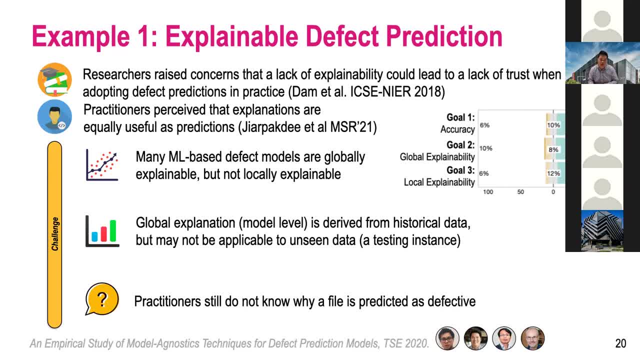 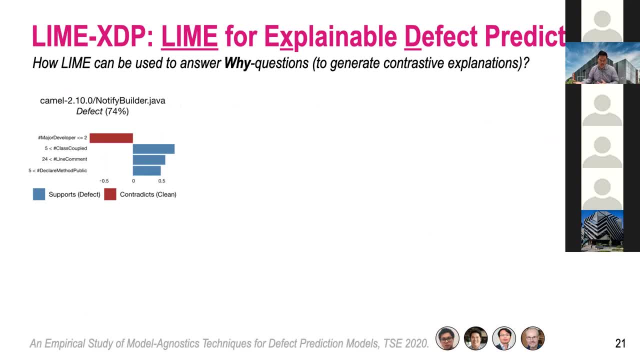 And, as I already mentioned, practitioners still do not know why a file is predicted as defective. So in this study, which is published at the IEEE Transaction on Software Engineering, we use LAM to answer four types of why questions. So the first one is that we want to answer. 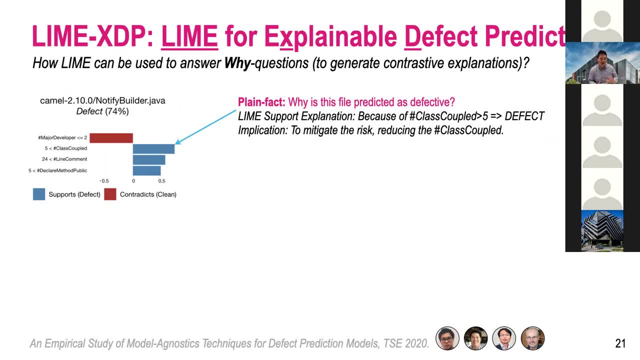 why is this file predicted as defective? This is an example visualization from LAM. Given this file, what are the features? There are two types: supporting explanation and the contradicting explanation. So we're going to look at the blue one. So in this figure it shows that 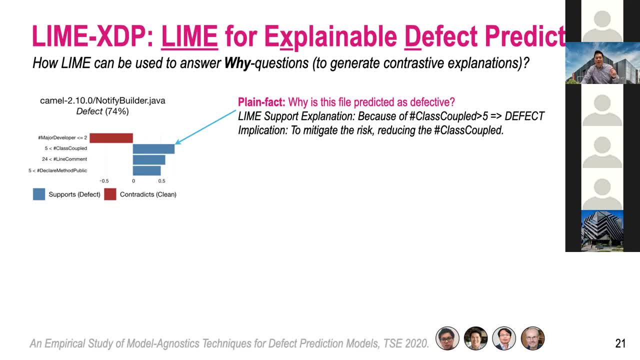 this file is predicted as defective because the number of class couples is greater than the number of comments, comment lines is more than 24, something like that. So it means that to mitigate the risk, we should consider reducing the class couple. This is an example And we can also use to 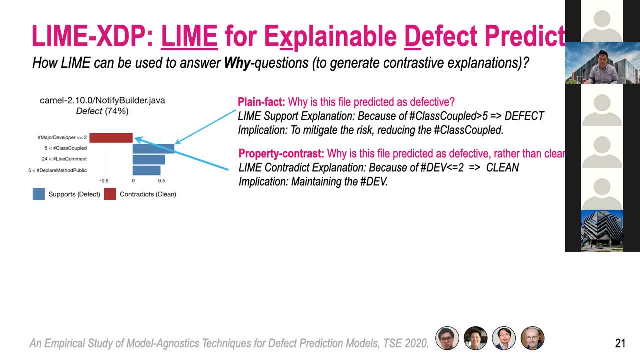 answer the property contrast as well. Why is this file predicted as defective rather than clean? So we, based on the LAM explanation, we know that the number of class couples is greater than 5.. We know the supporting explanation and the contradicting explanation, the red one as well. 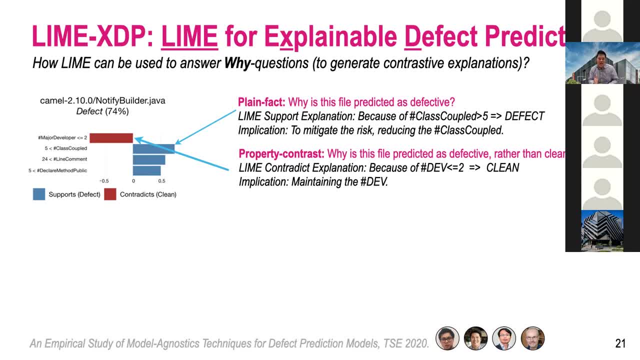 So, like in this one, we know that the LAM is predicted as defective rather than clean. because the number of deaf developers is less than two. It means that we should maintain the numbers of developers. We should not increase it at all. Does it make sense? everyone? 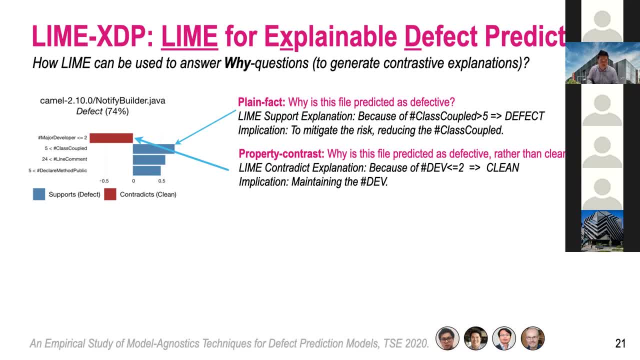 Yes, Okay, And then in Thank you, And then we can also use to answer the other two types of questions as well. Time contrast explanation. right, Let's say, if we build a defect prediction model at the release one and release two, One file given the same file in the release one is predicted as defective. but 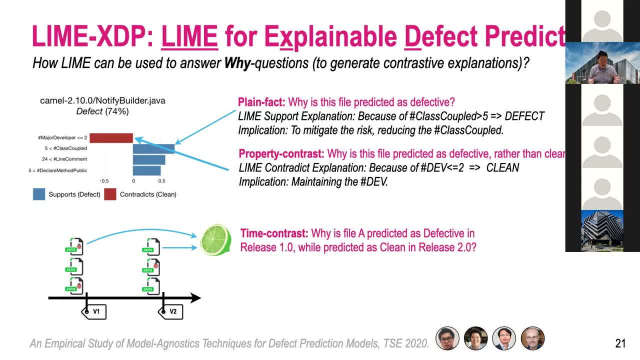 later on it is predicted as clean. Then the question is that: why is that right? So we can use LAM to explain the model in the release one and the release two as well, And within the same release we can also study what are the characteristics of the files. 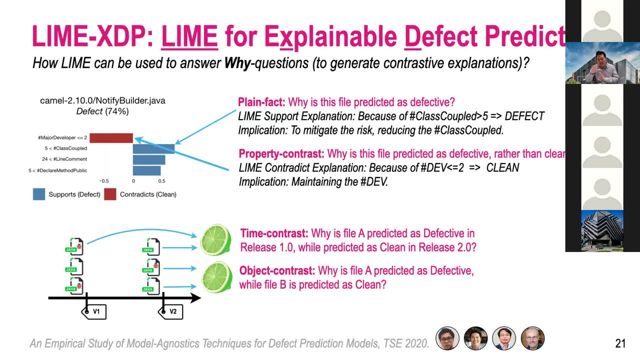 These kind of files are predicted as defective, while the other types of files are predicted as clean as well. So what I'm going to say here is that the model agnostic technique can be used to explain the defect predictions in many scenarios, to many questions. 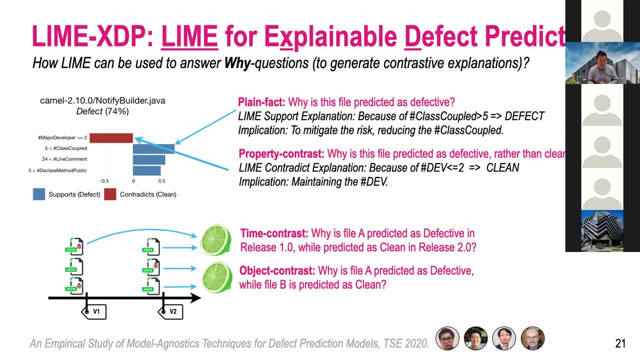 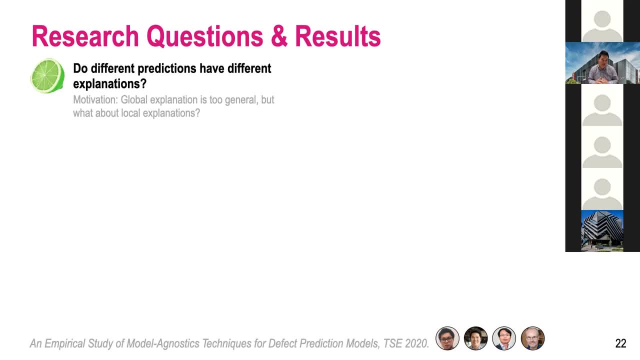 as well, And this kind of knowledge is very useful to practitioners. So in this study we conduct an empirical study to better understand the LAM for the defect prediction models. So the first question that we ask is: do different predictions have different explanations or not? 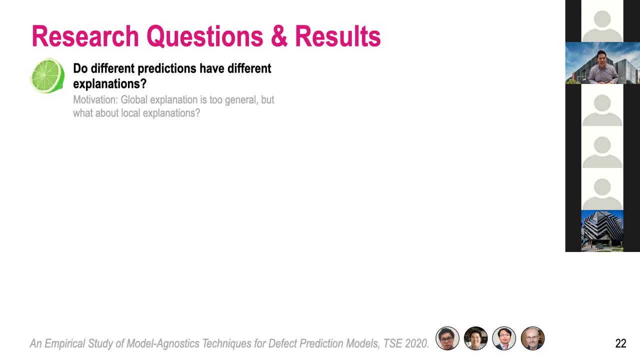 So the motivation here is that normally global explanation is too general. but what about the local explanation? Are they different? If they are different, it means that the global explanation may not be applicable to all of the local explanations at all. So what we find is that, given the same defect models, different predictions actually produce. 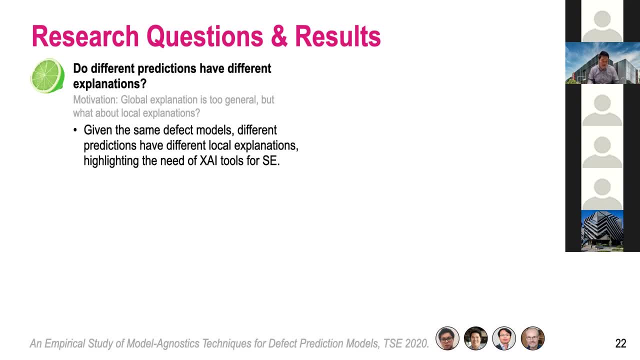 different local explanations. So it highlights the need of the expandable AI tools for software engineers And we also ask whether the local explanation overlap with the global explanation or not. And the motivation is that, ideally, local models should accurately mimic or approximate the behaviors of the global model. 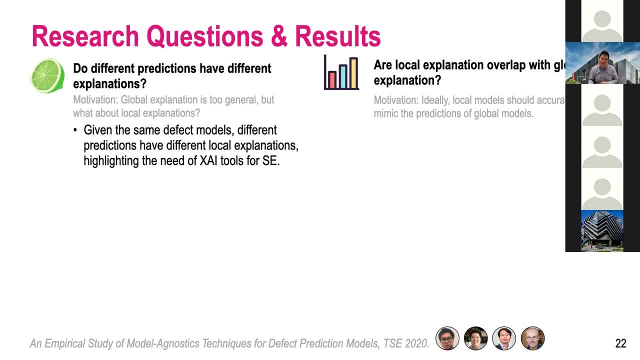 So we're going to look whether they are aligned with the global explanations or not. So what we find is that the top 10 features of the local explanations overlap with the global, but they are not the same at all. So that means, let's say, given the top 10 features of the local one, 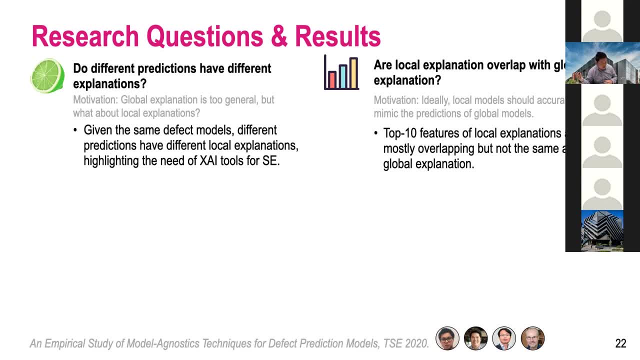 these top 10, they are the same as the global one, but the ranking they are different. And the next question is that: are model agnostic techniques rely on the random seed or not? Because this kind of technique is called, how can I say? 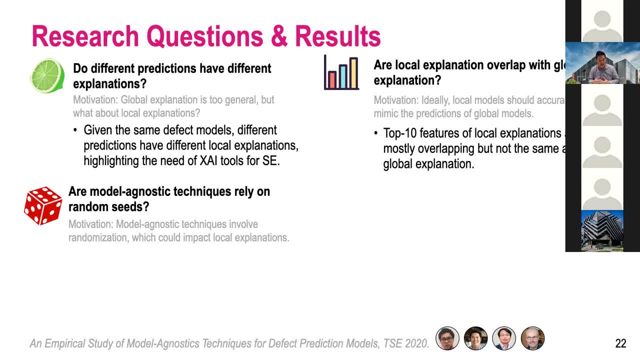 like perturbation-based modeling. It relies on the model agnostic techniques. It relies on the randomization. It relies on the random perturbation. So the different random seed may have may produce different explanation as well. So we also evaluate LAM for the different prediction models. 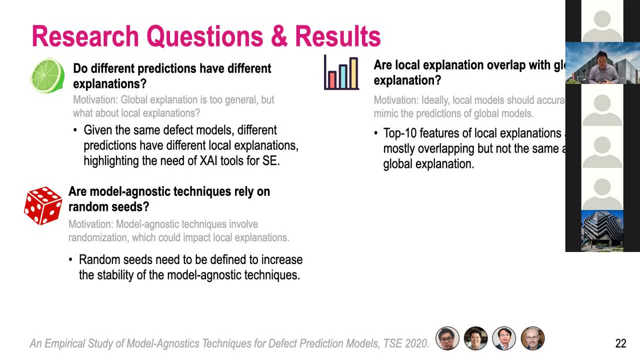 And what we found is that, yes, different random seed produce different types of explanation. So that means, to ensure the stability of the model, agnostic techniques, the random seed should be defined earlier And finally, once we generate different types of explanation, 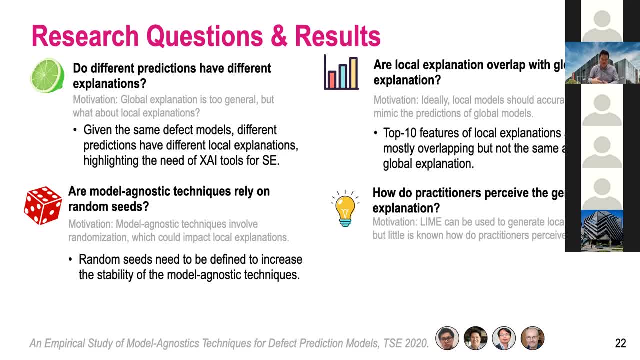 we send this back to practitioners and we run a survey. How do they feel? What do they think? How do they perceive about the explanation? And what we found is that 65% perceive that the time contrast explanations are the most useful. That means the time contrast explanations are the most useful. 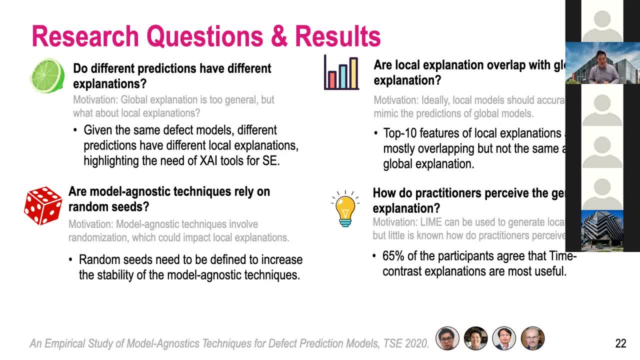 That means the time contrast. It means that when a file, the same file, in version one is predicted as bug, but they are predicted as clean in the version two, Why is that? So? I think they perceive that this kind of explanation is the most useful. 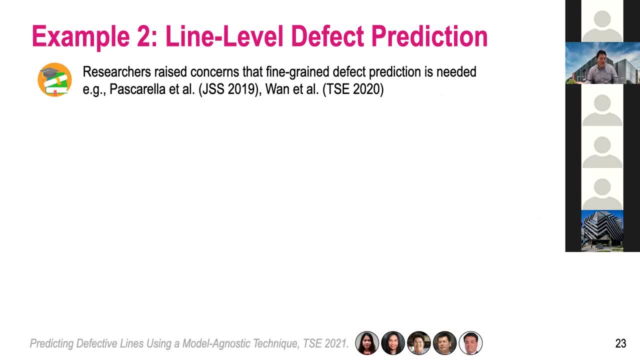 And next I'm going to show you the next example About how can we use the explainable AI techniques to make the predictions of the defect models more fine-grained. So the motivation is that lots of researchers already raised concerns that fine-grained defect prediction is needed. 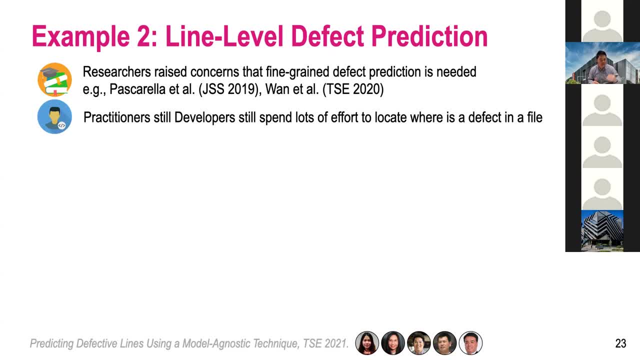 Because most of the models, at the moment they are predicted at the file level, the class level, the component level, But at the same time, developers still need to spend lots of effort to locate where it is, where the bug is in the file. 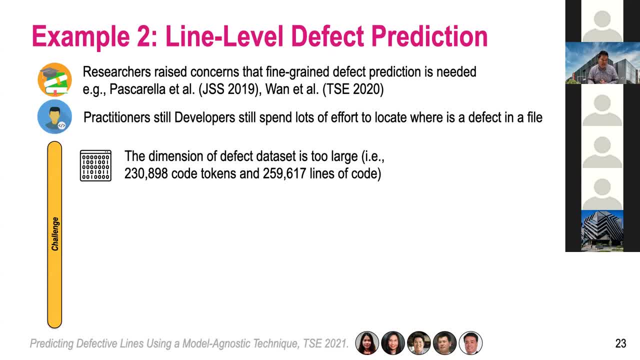 So there are lots of challenges in this study to build the line-level defect prediction. So let's take an example. We just take one software system. We found that, let's say, if we are going to build the backward models To predict at the line level, what we found is that the data set is too large. 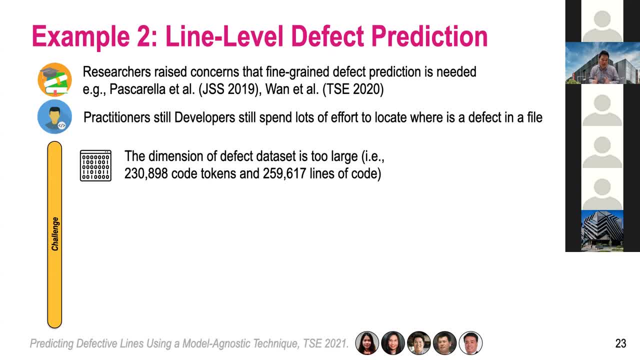 The dimension is too large. We have like over 200,000 code tokens, the features and more than 200,000 lines of code. So to build like a machine learning model it is still not easy, And we also found that the ratios of the defective line is still low as well. 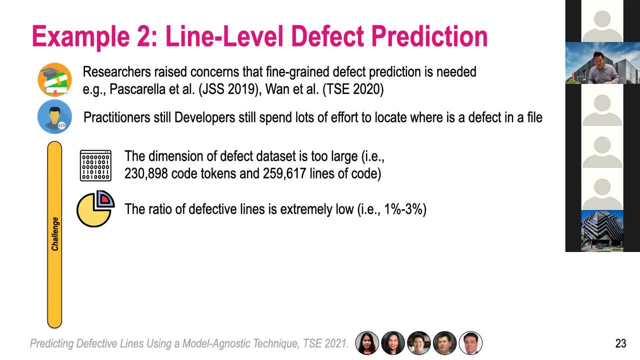 That means we have 200,000 lines of code. Only 1% to 3% of them are actually considered as defective lines. This is like finding needles in a haystack. How can we effectively build machine learning models or AI models to accurately predict which lines are the most risky? 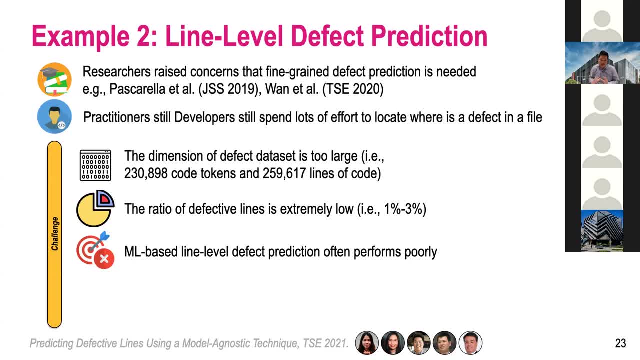 And when we try to build a machine learning model, it doesn't work at all. It doesn't work Because the data set is too large, The class is too imbalanced And at the moment I still have never seen any deep neural network to predict at the defective lines as well. 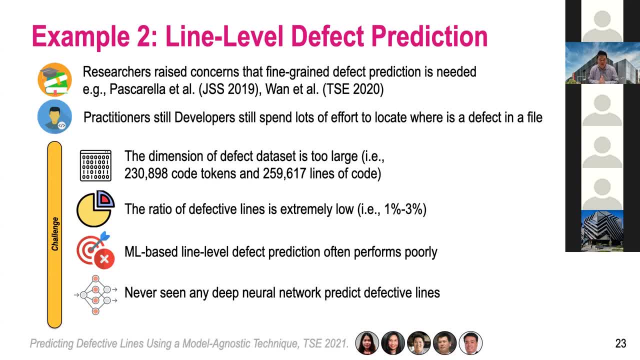 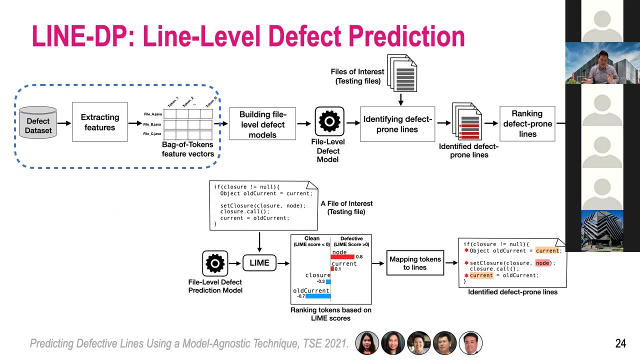 So this problem is very, very hard, very difficult, very challenging, And I am going to demonstrate present. next, how can we leverage the explainable AI technique to predict defects at the line level. Okay, So the key concept of the line level defect prediction is to build two-step model. 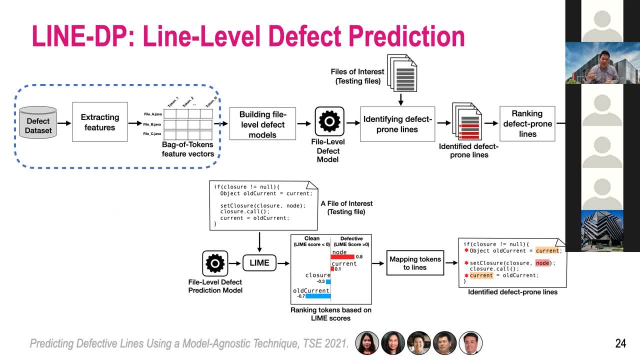 We're going to build the model at the file level and use the explainable AI to localize the tokens at the line level. Okay, So in the first step, given a defect data set, we extract the features. We just use a simple idea. 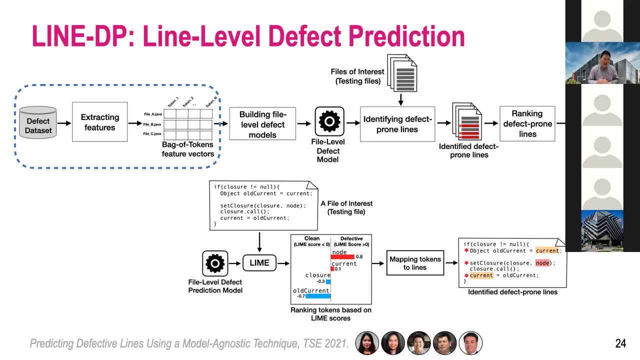 The backup was the backup tokens. That means how many tokens that appear in that file. Okay, So once we have this kind of data set, we're going to build the model at the file level And then we're going to build a prediction. 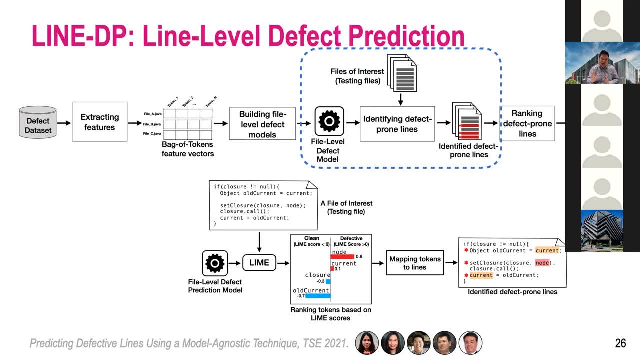 Okay, Just prediction, Whether this file is buggy or not. And then, given this file and instance to be explained and the model agnostic technique, In this paper we use LARM. We're going to take these two inputs into the LARM in order to understand which tokens are the most valuable. 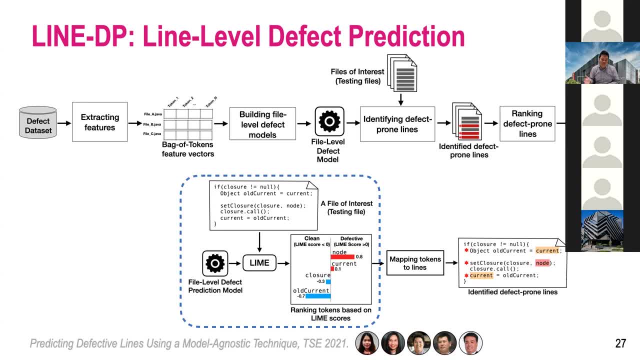 Okay, Which are the most important for this particular prediction? Okay, Once we know the tokens, we're going to map the tokens into the lines And then we can identify which lines are the most defect prone. Okay, So we can prioritize: the most risky one to the top and the least risky one to the bottom. 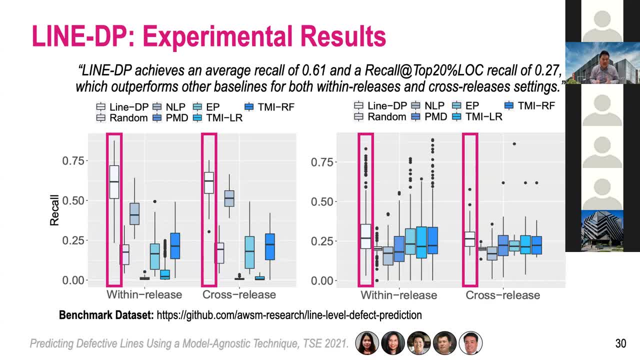 And the results are pretty fantastic. You know, We achieved the highest recall. That means we achieved around 61% recall, And the models also produce the ranking of the defective lines very well as well. And we also evaluate with the state-of-the-art approach using multiple techniques, including N-gram and the static analysis. 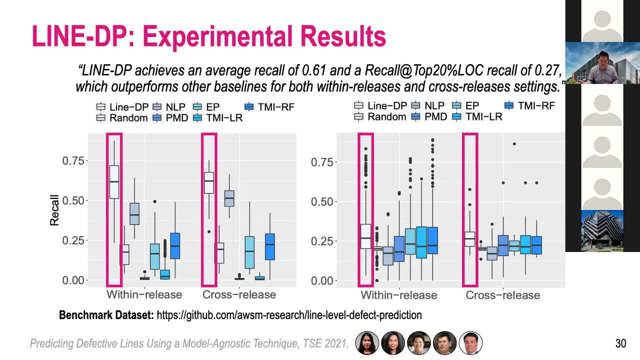 We found that our approach outperforms all of the baseline For both. Okay, So we can see the difference between release and the cross-release settings. Okay, And because this topic is very challenging, it's not easy at all- So we produced the benchmark data set. 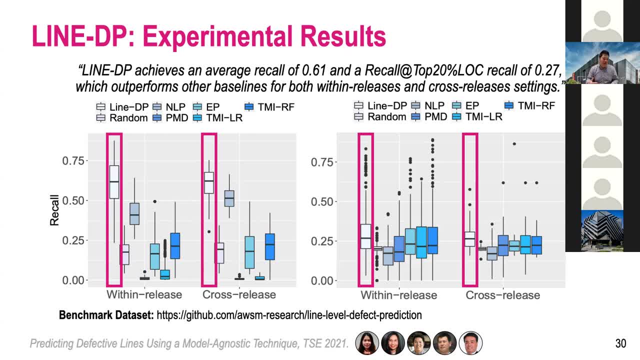 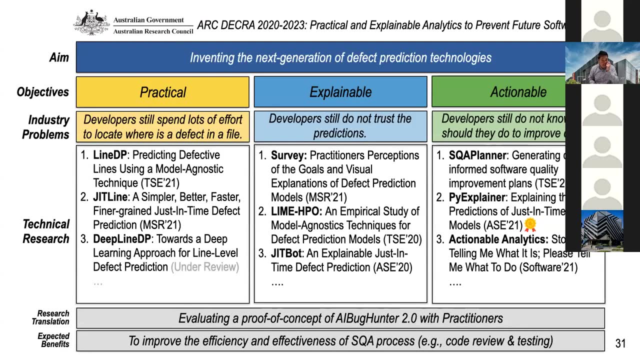 So if someone has a better idea, who is an expert in the deep learning or AI, they can use this data set to improve the accuracy of this paper as well. Okay, So, in general, what I'm doing here is it is the resource from the research project, my own research project, which is funded by the Australian Research Council. 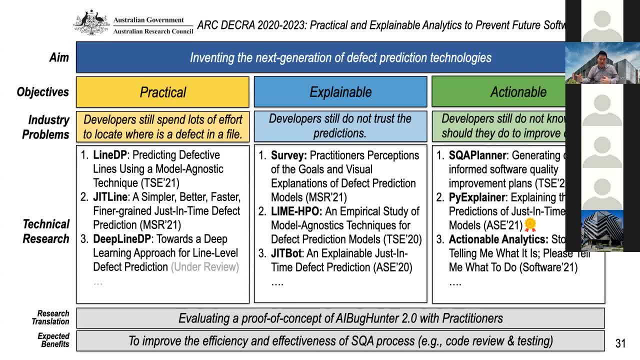 I think that the key aim is to invent the next generation defecation technologies. It has been proposed for a while, But how can we make it more practical and more expendable and more actionable as well? I tackle industry-related problems First. developers still spend lots of time to identify where the bugs are. 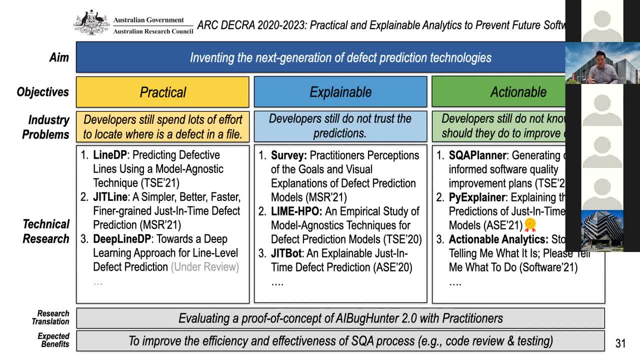 So we build the live-level defecation prediction. And when developers still do not trust, we conduct a survey, study, build, make the defecation models more expendable. And the last part is the actionable action abilities. Developers still do not know. 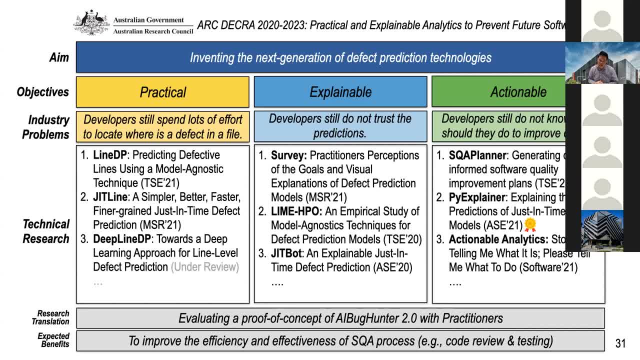 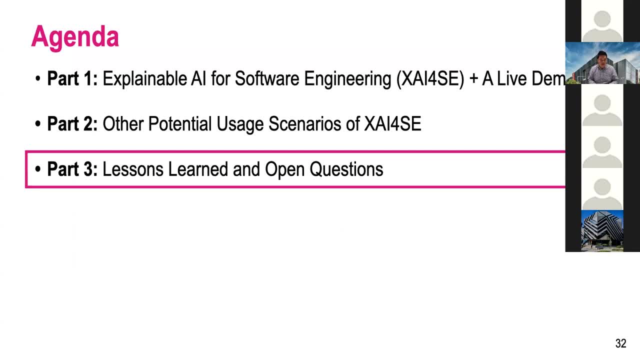 What should they do to improve the quality of the bugs, of the files, of the predictions? So we propose lots of approaches to make the defecation models more actionable as well. Yep, That's all. Before I am jumping to the next part, any questions that I should answer? 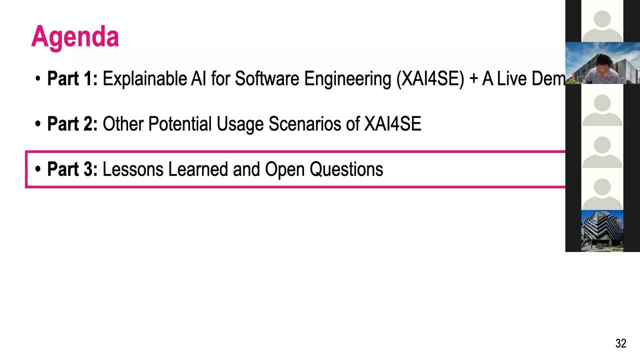 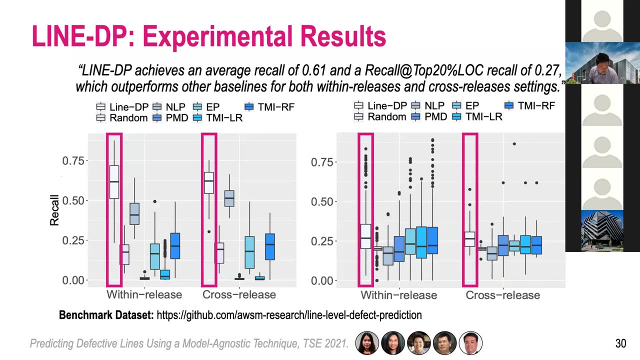 Let me look. Yep, I presume this is not cross-project, trained within project. Yep, No, So we have. we do both within and oh yeah, yeah, yeah, yeah, I see what you mean. Yes, Not, not cross and not within project and cross project. 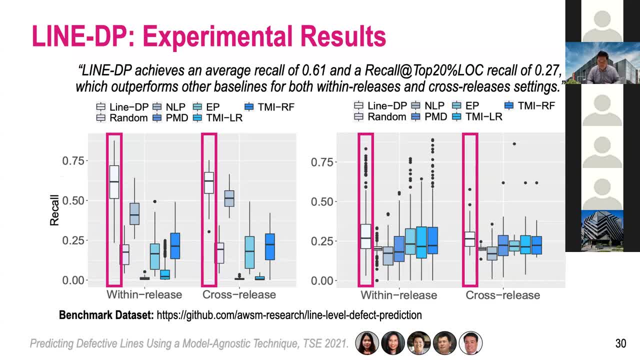 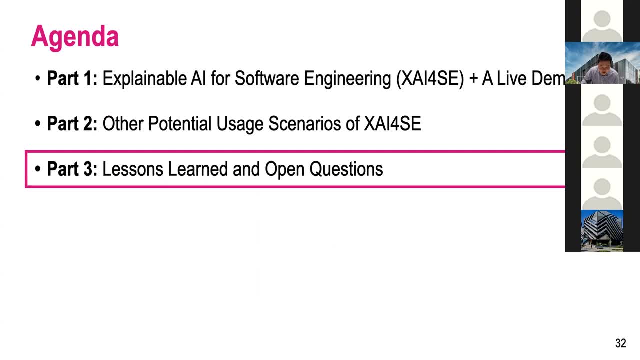 This is just only within release and across release. Yeah, Yep, Any questions? Any questions? If no question, then I will move to the next part, the lesson learned and the open questions. Okay, Okay, Okay, Thank you, Thank you. 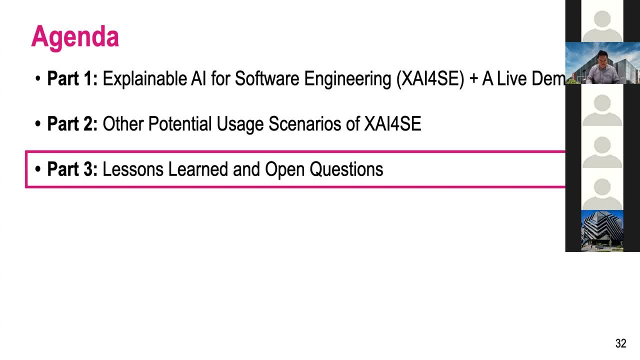 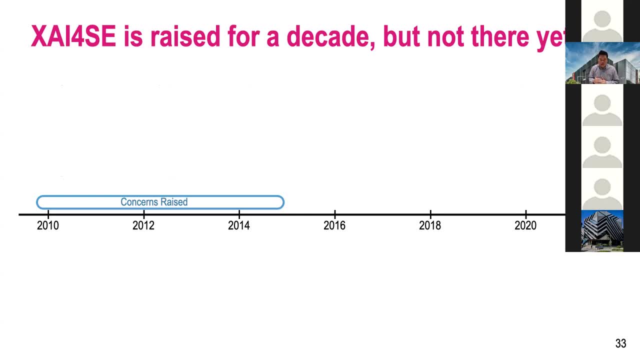 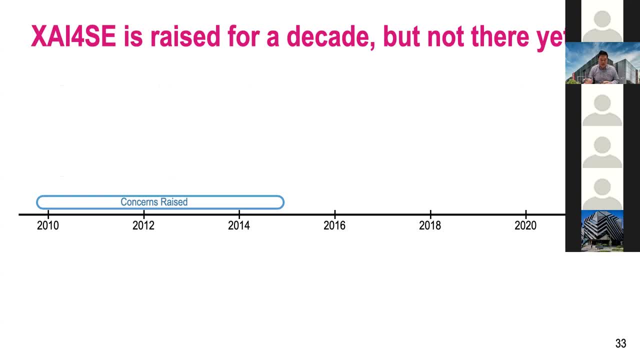 So in the first two part I already demonstrate lots of user scenarios of the expandable AI for SE, which is very modern. But I just want to say that the expandability is not something that new. okay, It has been based for a decade already, but it's not there yet. 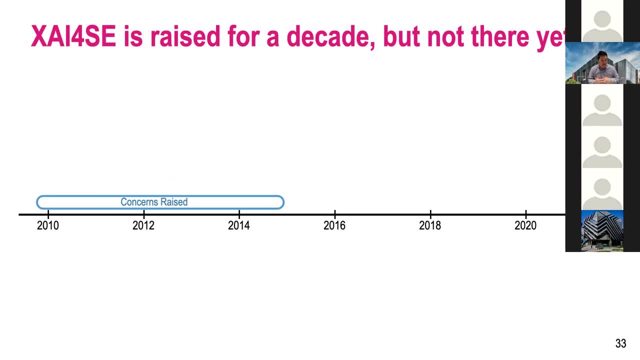 So let I So. in the past few days I just looked at the. I do some experiments. Okay, few days i just look at the. i do some literature review and try to do the, this kind of timeline mapping. okay, at the 2010, actually, singa, which is a game company very, very famous at that time, they 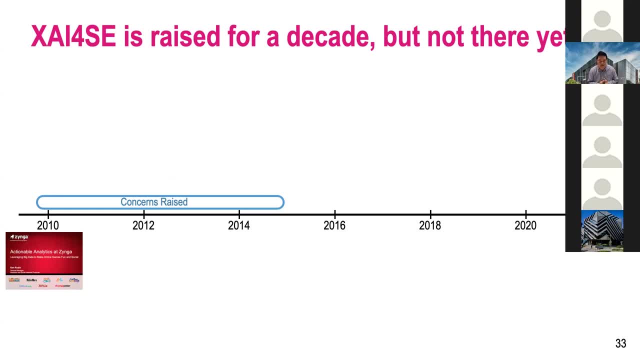 already start talking about actionable analytics. how can we make the software analytics more actionable? okay, and then in the xc uh 2012, tim menzies and thomas simmerman organized a fishbowl uh goldfish- goldfish bowl panel, talking about software development analytics. and at that time, 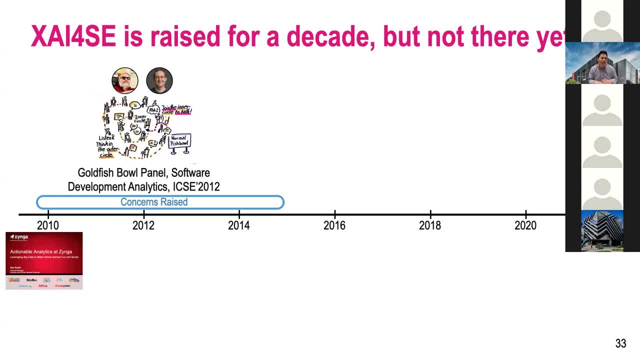 lots of practitioners and industry people. uh, they already raised concerns about the explainability. okay, and later on, uh, one year later, uh, tim and tom also organized a special issue, uh about software analytics as well, and they mentioned that, uh, software analytics must be real-time and more efficient. 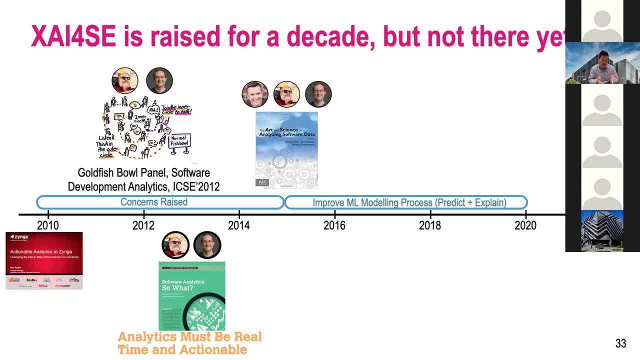 actionable right. So this is more like concerns that are rare. okay, But at that time, back to during 2010 to 2015,, we still do not see any research that tackled this area. okay, And in 2015, Kristen Bird, Tim and Tom also wrote a book about the art and science of analyzing software. 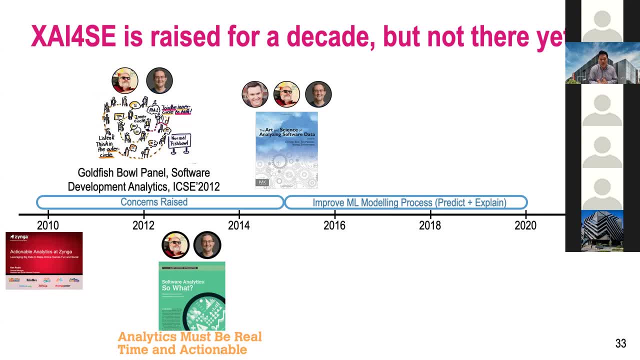 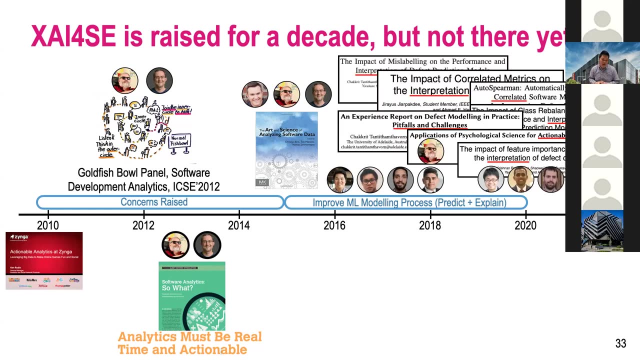 data. So basically, we just start the age of how can we improve the machine learning modeling process to make the models more accurate and more explainable. right And during my PhD study, I also published lots of papers and raised concerns about the mislabeling data, the correlation. 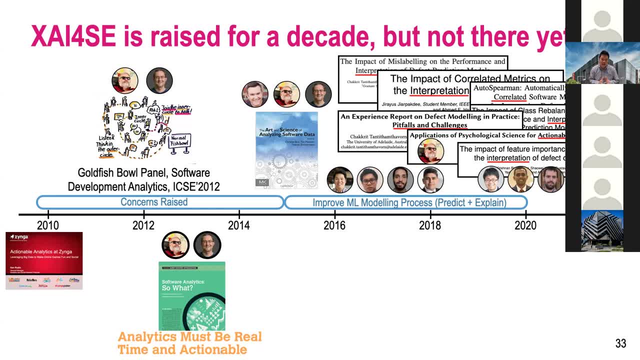 about the feature selection. lots of techniques or experimental choice actually have an impact on the model And later on, people also organized a special issue as well, who, in 2018, wrote a short paper at the ICSI near track about explainable software analytics. And recently I also raised concerns. 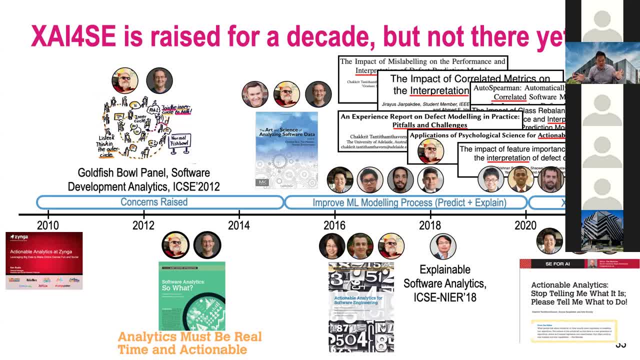 about actionability as well. So, as you can see, there are lots and lots of researchers, rare concerns, but we are not really there yet. Like, how can we make the deep learning more explainable, understandable to end users, build a better trust? this kind of 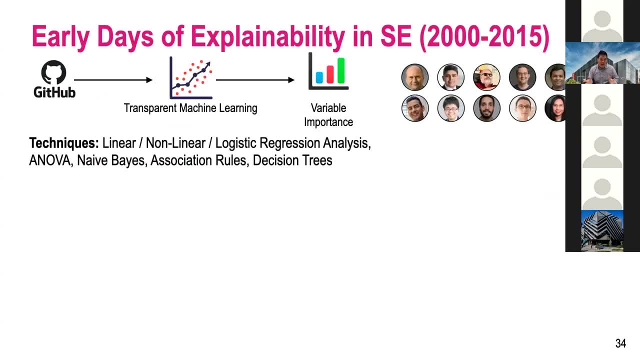 thing, right, Yep, And early days of the explainability in SE. let's say like this is like 20 years ago, 2000 to 2015,. right, There are lots of researchers often use like white box technique or transparent machine learning, like linear regression, nonlinear regression or using ANOVA, Naive Bayes Association, And there are a lot of researchers who are using this kind of thing. right, And early days of the explainability in SE, let's say like this is like 20 years ago, 2000 to 2015,. right, There are a lot of researchers who are using this. 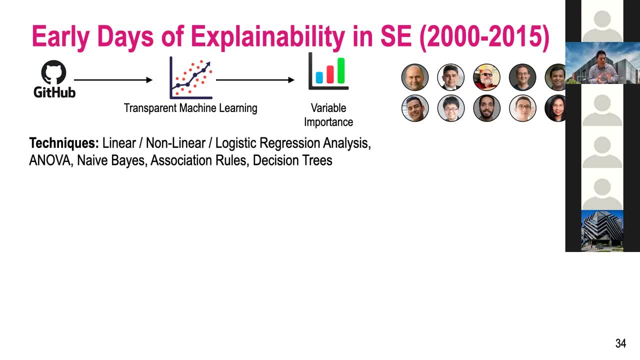 kind of thing right, And early days of the explainability in SE, let's say, like linear regression or using ANOVA, Naive Bayes Association, And there are a lot of researchers who are using this rules and decision trees to build a local- no, build a global- interpretable model. right? 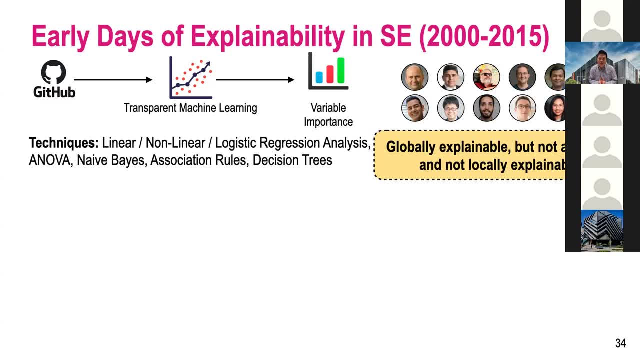 But this kind of technique, yes, they are understandable, but the problem is that they are not accurate and they are not locally explainable at all. They just build a dataset, build a. prepare a dataset, build a regression model, evaluate the R-square, And most of the time, 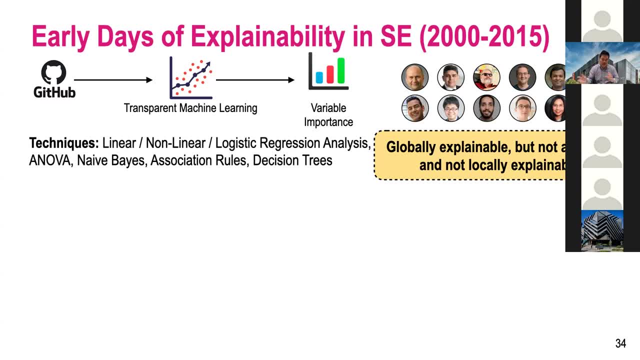 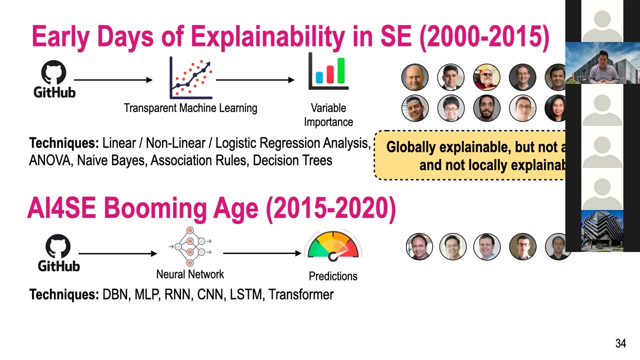 R-square is relatively low, let's say less than 0.2%, Right. So that's why, in the past five years, there are these kind of people like Prem, David Lowe, Dennis, Gravely, Barbota or Max. they tend to use, like an AI, a more complex model. 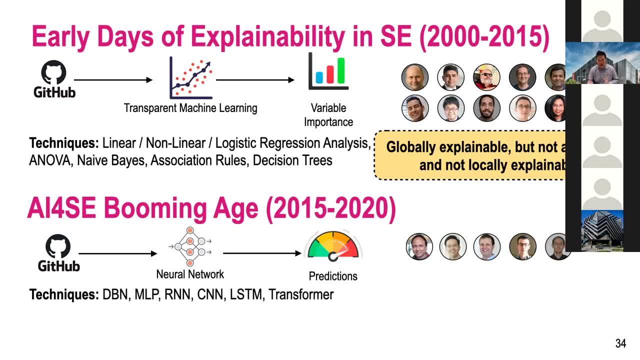 like deep belief, network, MLP and lots, of, lots of architecture to make the AI models more accurate. But these kinds of models are very accurate, yes, but they are not explainable at all. So how do you explain this? So how do you explain this? 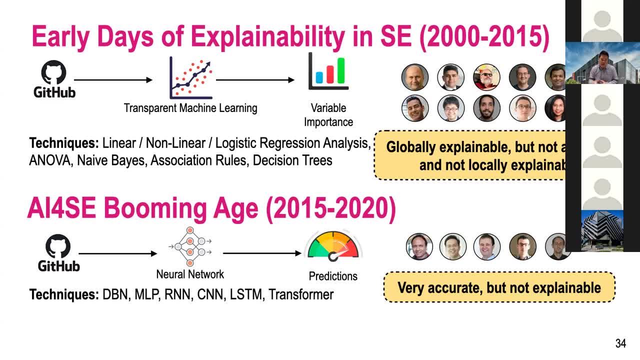 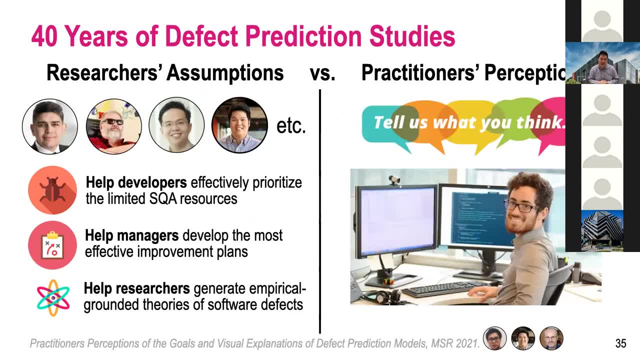 So how do you explain this? How can we bridge the gap right, Like, how can we make these kind of models more explainable? Yeah, And we also, yeah, talk about the. let's take a look at the defect prediction concept. 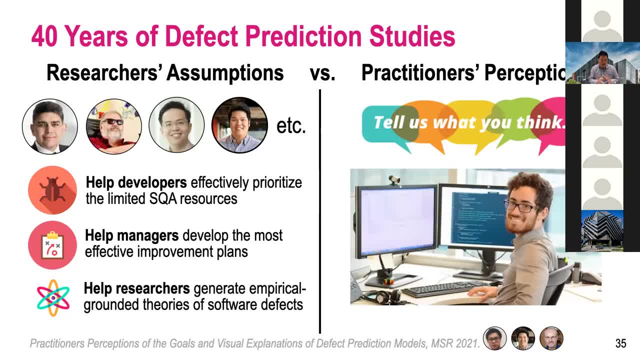 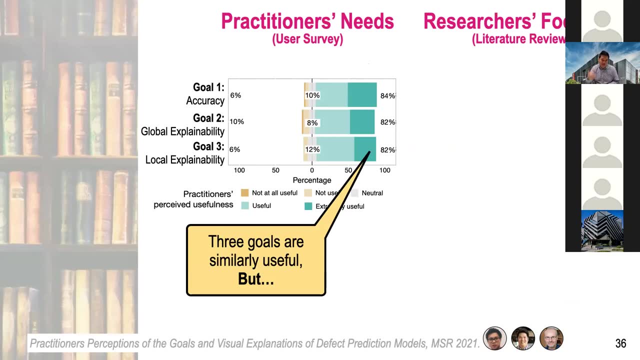 right People. there are lots of researchers propose lots of techniques. So in this study we want to investigate: what do practitioners think? What we found is that the practitioners perceive that the three goals are similarly useful. right, But when we look at the systematic literature review, look at the 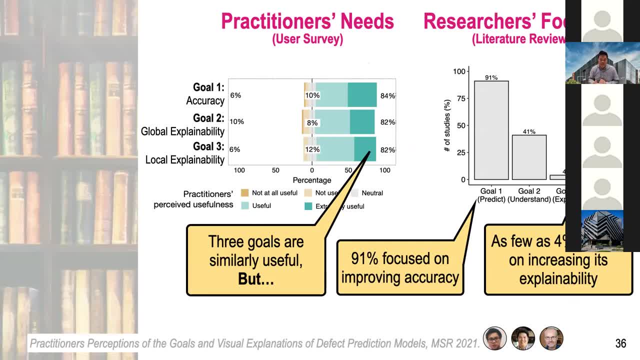 study at the literature so far, we found that 91% of the study only focus on improving accuracy- like too much incremental improvement already, But there are only 4% actually focus on the increasing the explainability. So how can we make the AI for SE models? 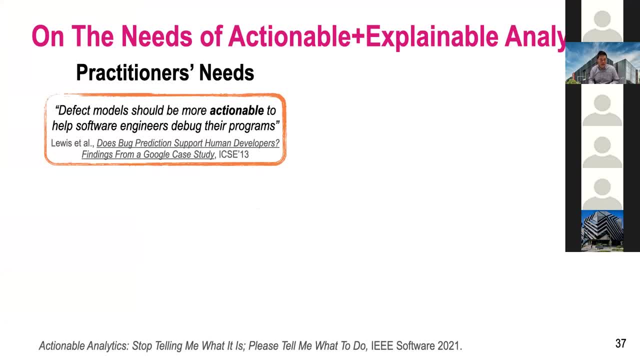 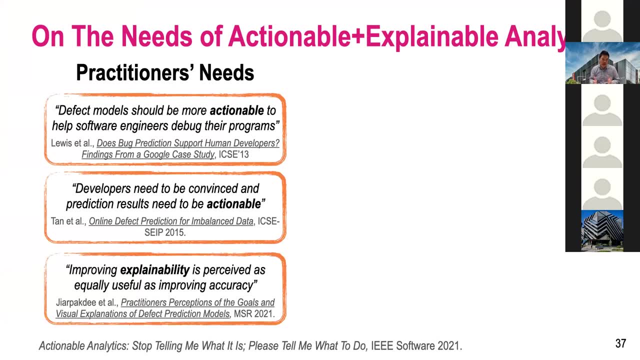 more explainable right, And this is not just only the practitioner survey but, as I already mentioned that there are lots of researchers talk about explainability and the actionability as well. like on the left hand side here, these are the case studies of the defecation model in practice when they are deployed. 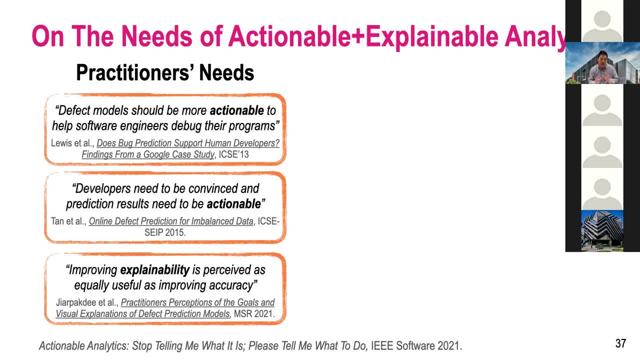 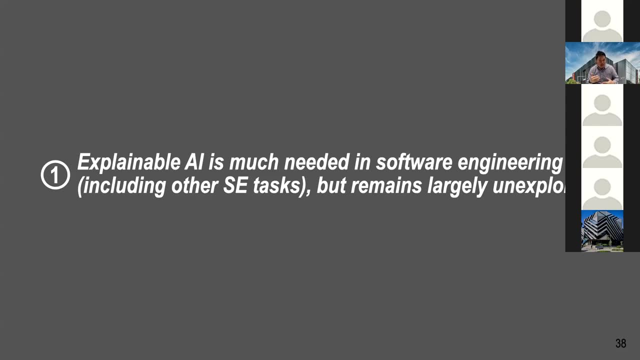 And what are the feedback that they get. And most of people, most of developers, just raised concern about how can we make the fabrication models more actionable, and, yet again, researchers as well. so the key takeaway here is that i just want to say that expandable ai is much needed in software. 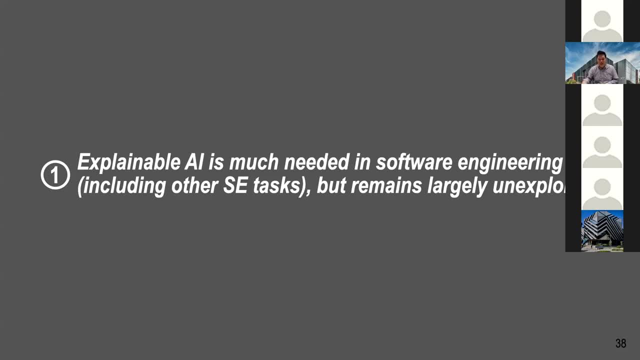 engineering, including other software engineering tasks as well, but at the moment, it remains uh largely unexplored. so how can we make the community, uh, how can we uh develop more research in this area? right, there are lots of things to do, and the next thing that i want to say here is that 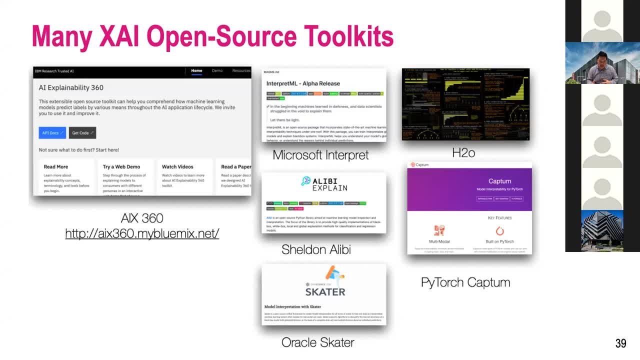 at the moment that, because of the field expandable, ai is quite mature. now there are lots of open source toolkits like a ai expandable uh, expandability 360, uh, the tool from microsoft interpret, uh, or python captain. there are lots of tools, okay, but uh, but when we look, 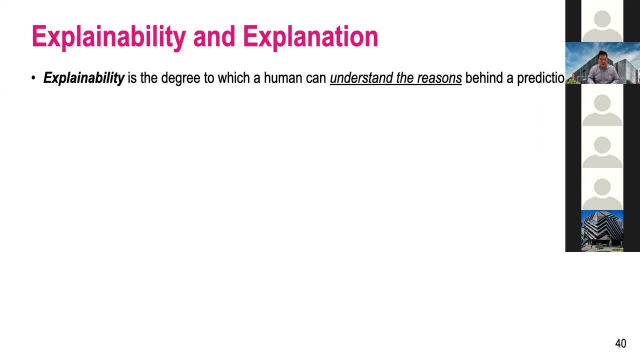 back to the theory of the expandable ai. it means that, uh, they want to. uh, it is the term. expandability is defined as the degree to which a human can understand the reasons behind the prediction right. so normally, explanation is used as an interface between the humans and the machines. so, uh, and then. 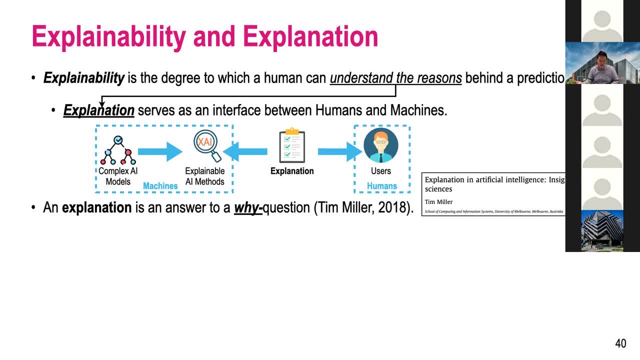 there are lots of research from the social science or psychology. they run a survey and they found an explanation is an answer to a y question and there are lots of types of y questions as well. there are lots of questions that need to be answered, so there are lots of challenges here. 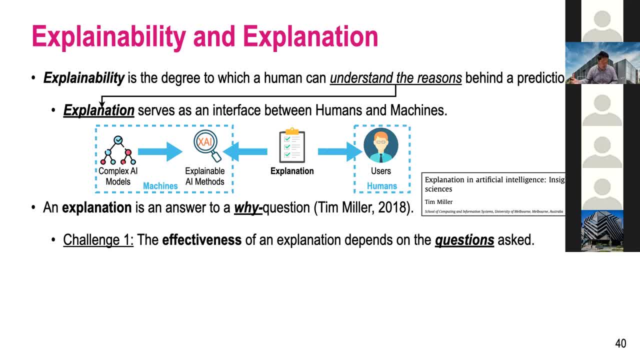 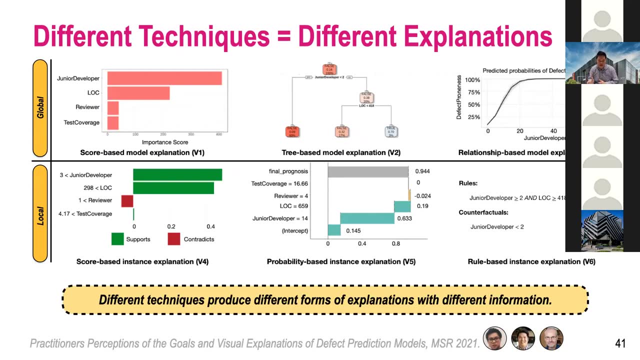 first, the effectiveness of the explanation depends on the questions, and the explanation can be presented in various scope and various form to serve a goal as well. right, and as i already mentioned, different techniques also produce different forms of explanation, with different types of information as well. then the next question is: 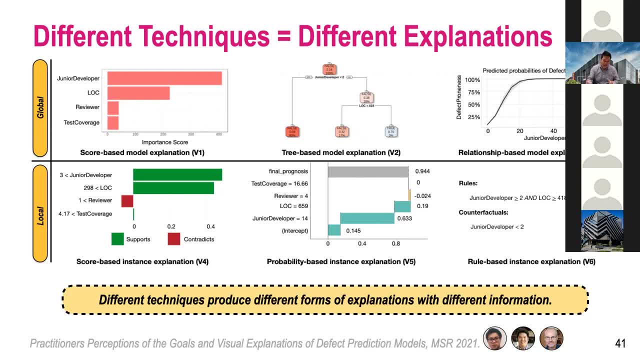 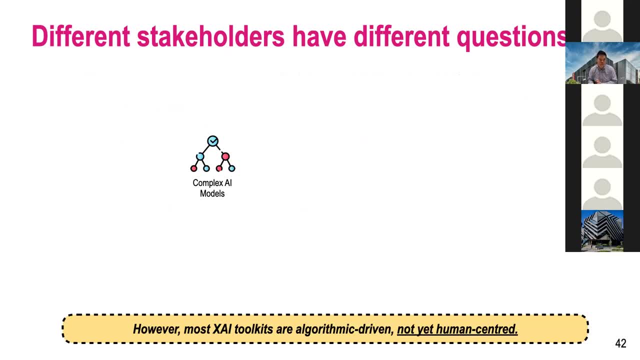 that, uh, no, this is a challenge, yeah, and the next, uh, and different stakeholders also have different questions as well. for example, given a complex ai models, they'll ask lots of questions: why am i getting this prediction? and because, uh, the, the end users, uh, who affected by the decisions. 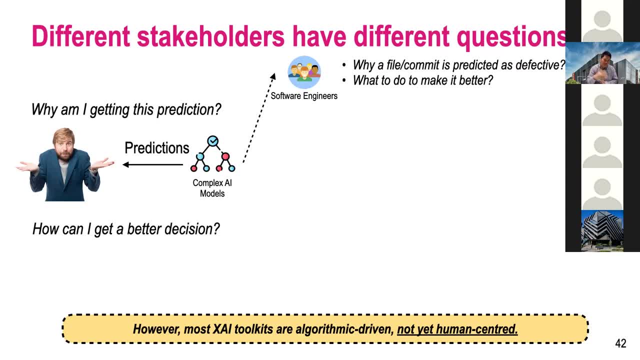 also have. we have many stakeholders. who? who is the end users of the complex ai models, right as a software engineers who take the different position. they also ask one set of questions: why if i is predicted as defective and how can we make it better? and ai expert also asked: like which ai? 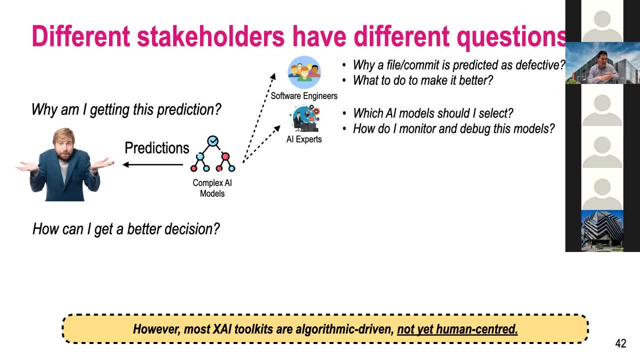 model should i select? right, let's say they build uh 10 highly accurate models, but how can they monitor or debug or select which four deals should be deployed in practice? right, uh, as a domain expert. they also ask uh like: uh, are the ai models learn correctly or not? is the ai model logic? uh, 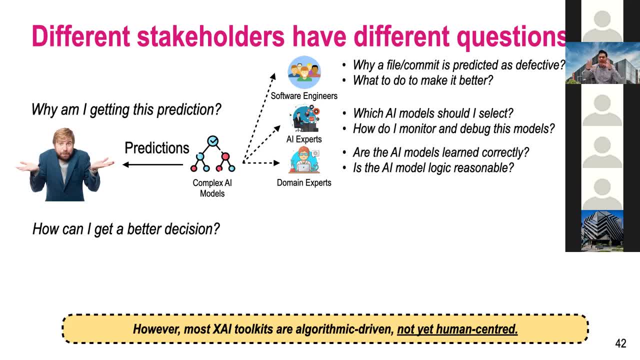 reasonable or not right, like for example in the image classification to classify a dog or cat. what if we explain the model and we found that they use background as a classification features? it doesn't make any sense at all, same to the defecation. what if the model use the blank lines as the feature right? so that means these kind of models are not. 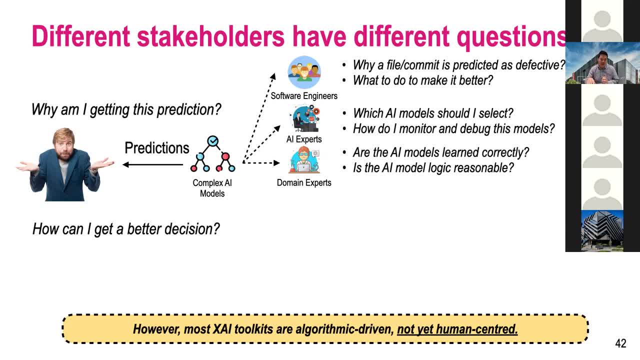 trustable. so how can we? so? the expandable ai can be used to develop appropriate trust and debug the model, help the software engineers understand as well. and the expandable ai can also be used to uh help like a business leader and policy maker, and the regulators as well. so what? 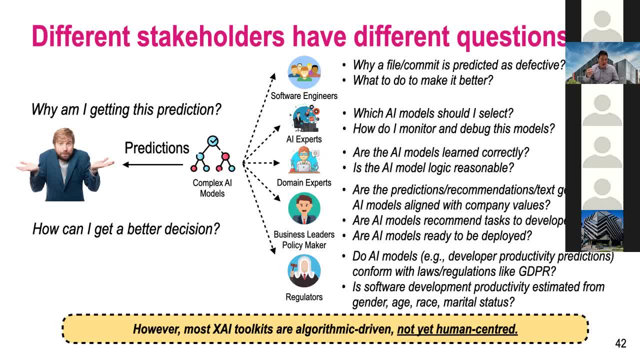 i'm going to say here is that, um, different stakeholders have different questions which require different types of explanation, and each explanation can be presented in many forms and many scope. but the challenge here is that most of the xai toolkits are algorithmic driven. they are built for researchers, but they are not yet human center yet, right. so 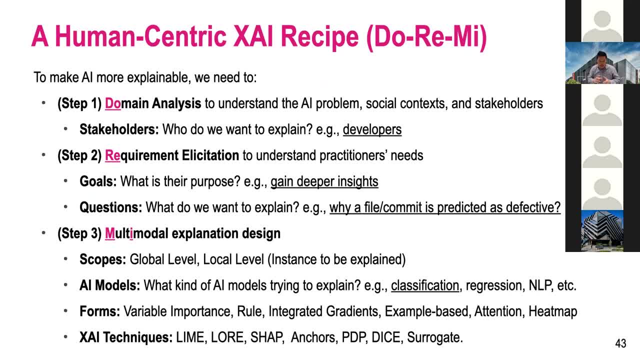 so in the future, i think that the explainable ai for software engineering should be human centric. how can we make the explainable ai tools, uh, that are designed by humans? also, how can we decide the explainable ai tools that generate explanation that most suit practitioner need? okay, one of the approach that we can do is called doremi. okay, this is a. 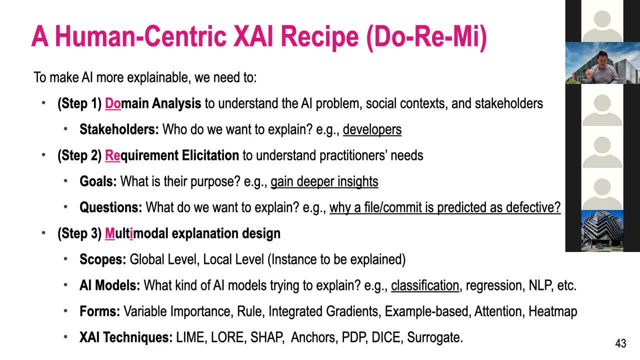 simple approach. the first step we need to study, we need to do the domain analysis to understand the ai problems, the social context and the stakeholders. who do we want to explain? we need to identify first whether we want to explain to the, explain the ai models to the developers or the. 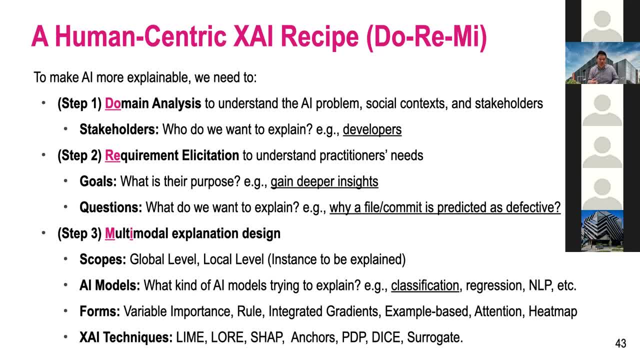 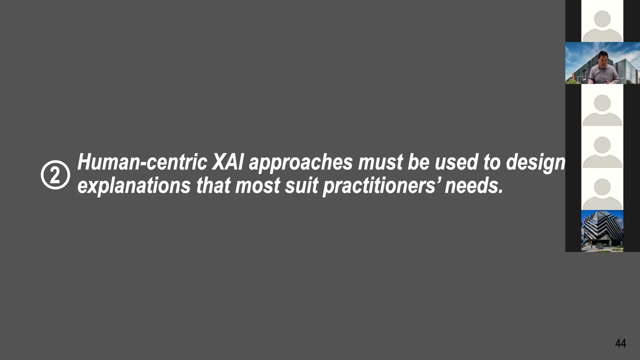 ai, expert, right. then we do the requirement, elicitation, to understand what are the practitioners need, what is their purpose, what do we want to explain? right, and then we can decide the explanation model, like what are the scope, the models and the forms and select the tools. so just to wrap up, uh, the the. the second key lesson learned is that human-centric. 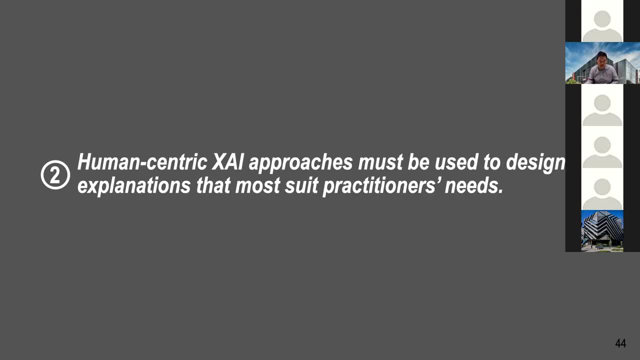 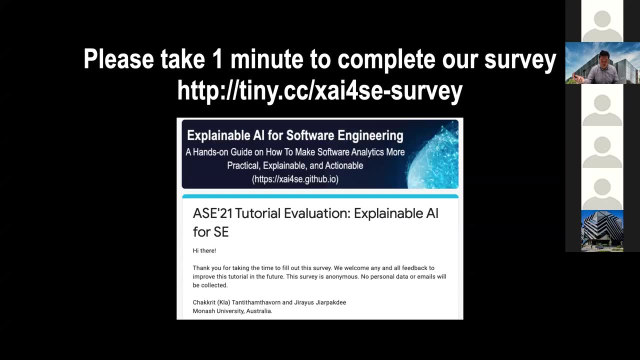 explainable ai approaches must be used to decide the explanation that most practitioners need, yep. so that's the oh. that's all for my tutorial today. now i think i will go back to the question again for within project: how so? i have the question from ali for within project: how do you split? 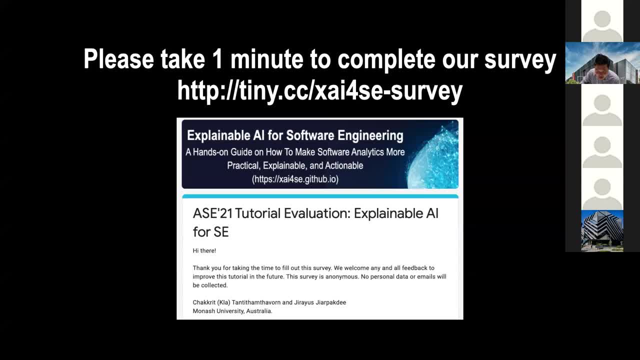 your training and testing data. is this a time order process? yes, uh, so for that paper we built the release space defect prediction models. um, uh, that means uh, the the earlier release. uh, we use uh for model training and the later release we will use uh for uh testing. yeah, but 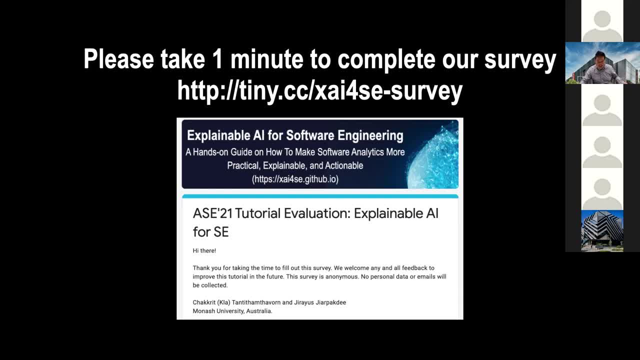 we also have another kind of another paper- it's called jit line uh- which is built based on the time order data and, yes, we sort the data set by the time and use the older commits for training and the later commits for testing. so they are not fixing, yeah. 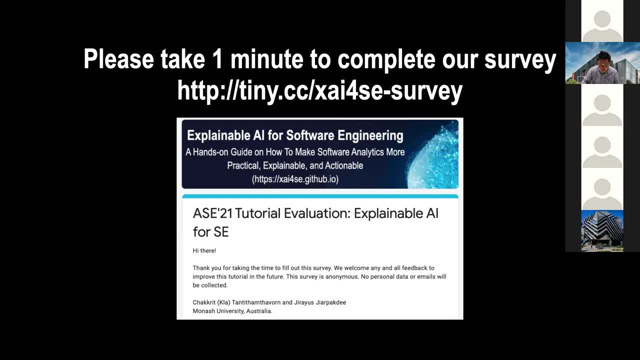 so these all come together? yes, a little bit of so. so that's all from my android. okay, steve question. happy to answer any question And again, if you have time, please take one minute to complete the survey as well. Thank you so much. 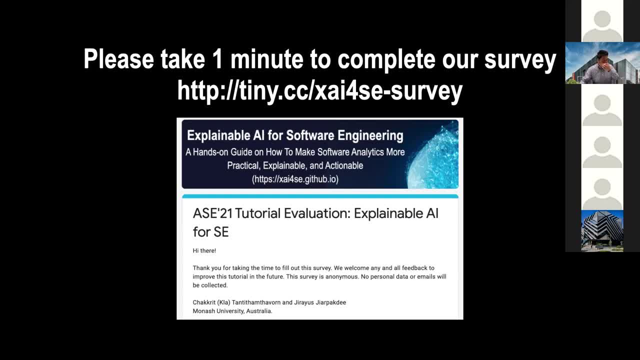 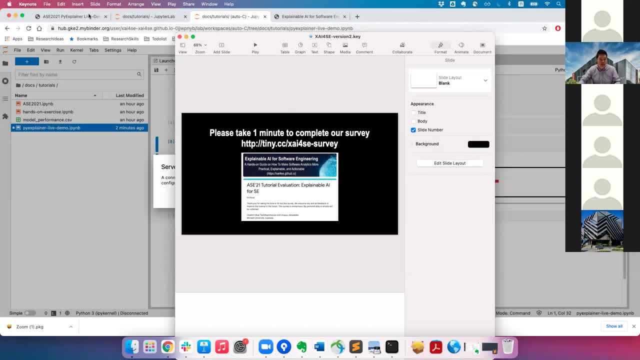 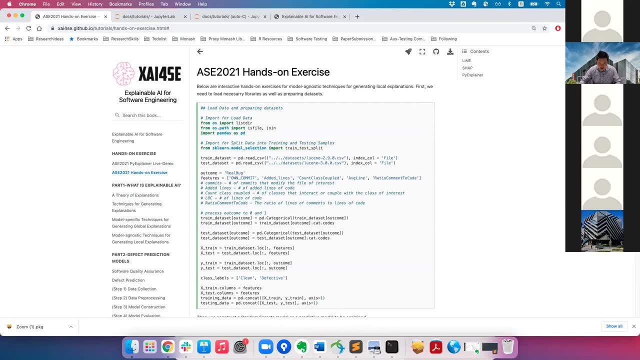 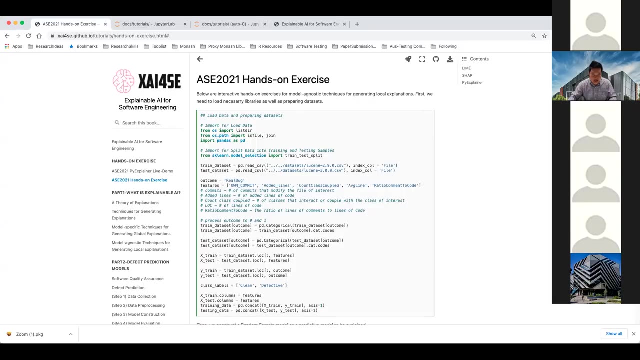 All right, So everyone next. I think the tutorial is already finished here, And the next step is going to be the hands-on exercise. Yeah, the hands-on exercise, So let me share my screen again. Yep, the hands-on exercise. 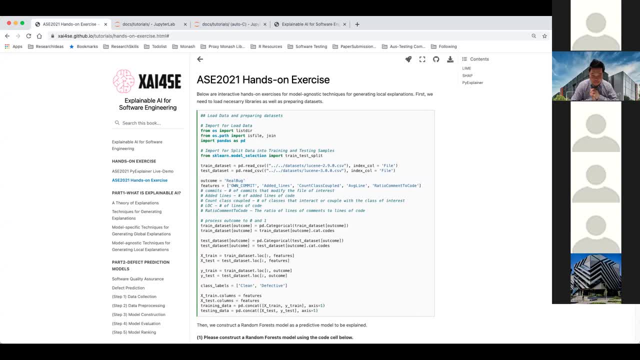 So, Jirayut, are you ready? Yes, Should I share my screen, or Yes, you can? OK, sure, Yep, you can Maybe just want to check again. Any questions? Any more questions? OK, no more questions. 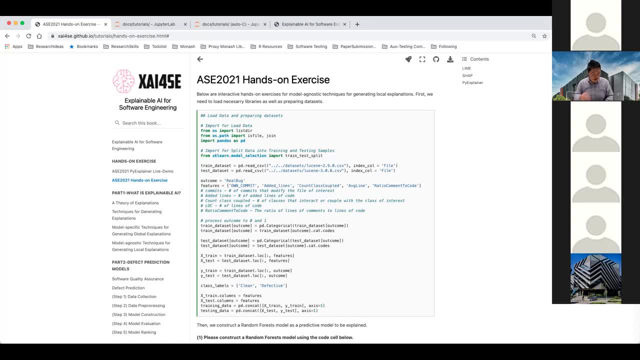 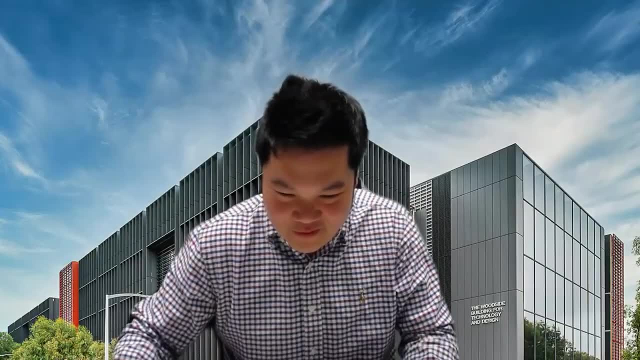 Then, yep, I think we can move to the next step. OK, The next part of the tutorial, which is the hands-on exercise. Yep, over to you, Jirayut. Yep, OK, Let me share this screen. 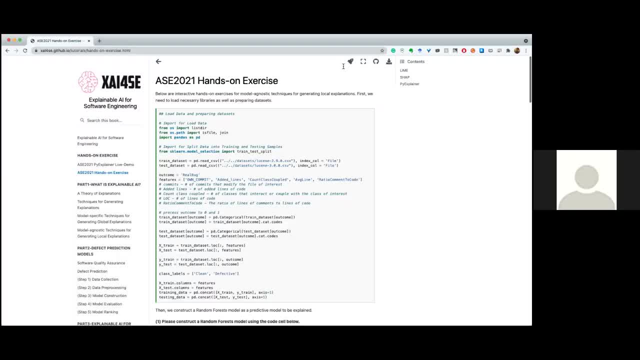 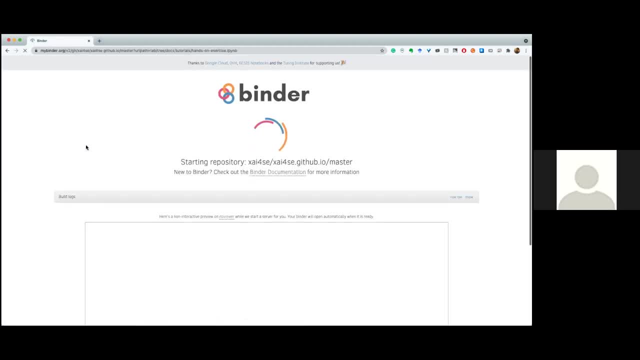 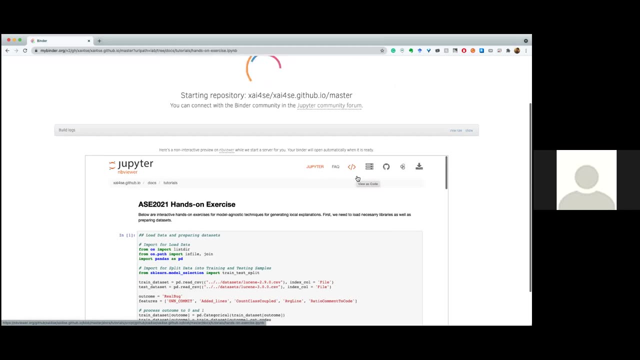 OK, so I'm going to use Binder to interact with this exercise, And this exercise has four main parts, but we are going to focus on three of them. first, because Cla has already covered the PI explainer And I'm going to show you how to use it. 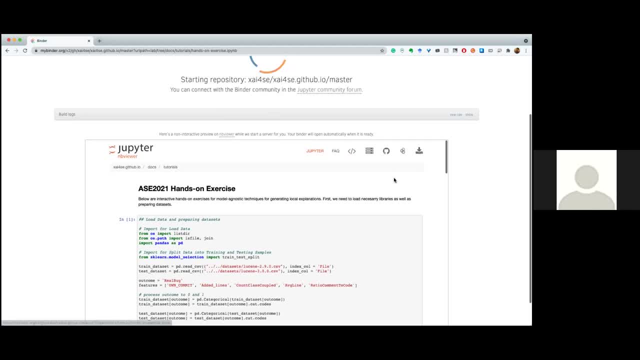 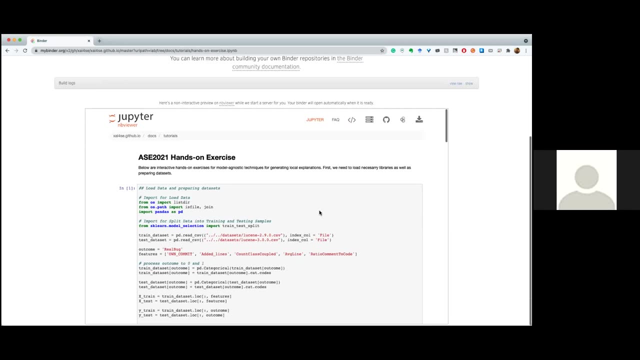 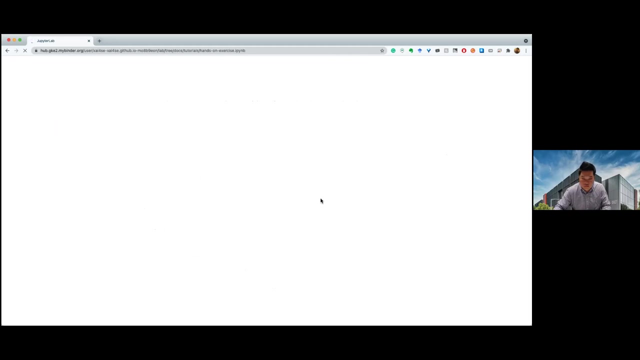 OK, So the PI explainer part. please wait a bit. OK, so everyone can follow the instructions And I'm going to show you how to use it. OK, so everyone can follow the instructions And I'm going to show you how to use it. 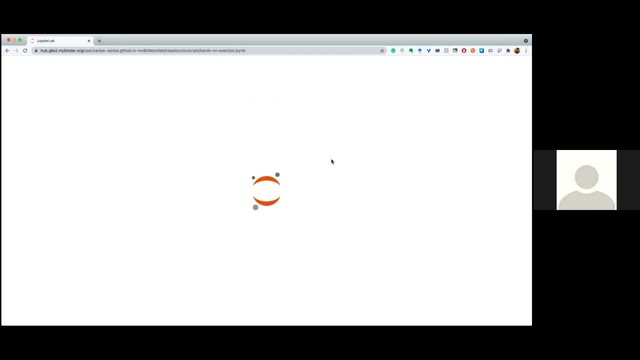 OK, so everyone can follow the instructions, And I'm going to show you how to use it, And I'm going to show you how to follow the exercise by using their own interactive notebook or just walk through with me. OK, so the first part here is to set up the environments. 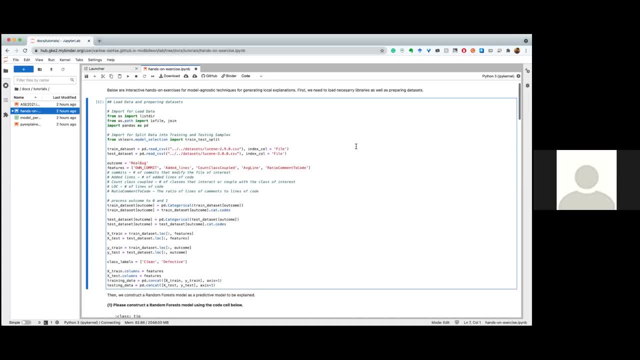 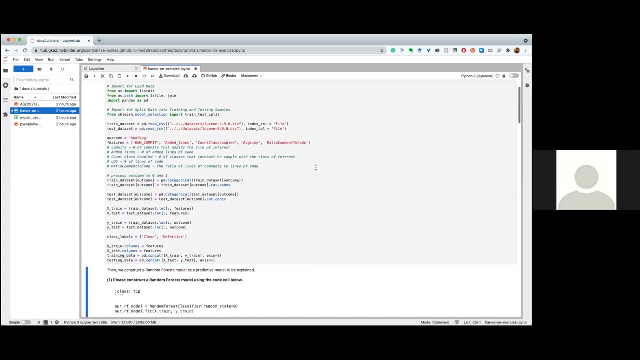 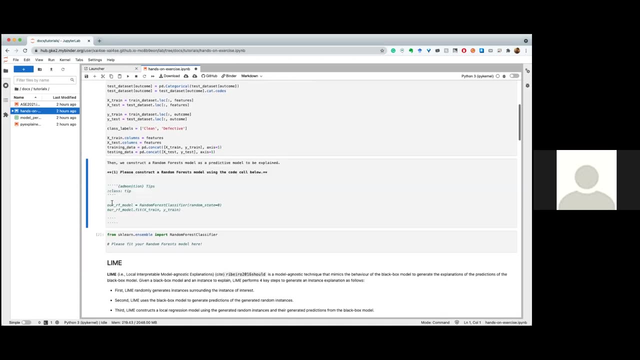 So when explaining any instance, first you need to prepare the data sets and the model. here We have already prepared some basic codes for you, So let's start with the first part. OK, first one. okay, constructing random forest- this one- uh, we can simply. 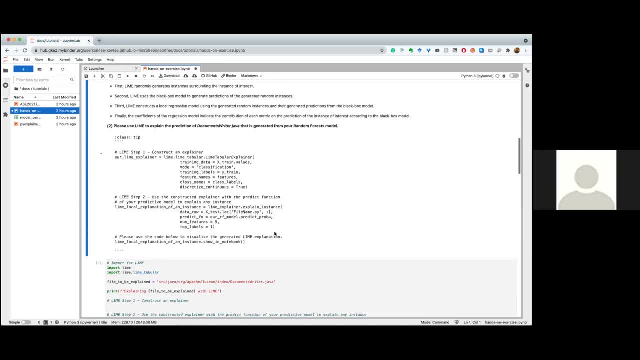 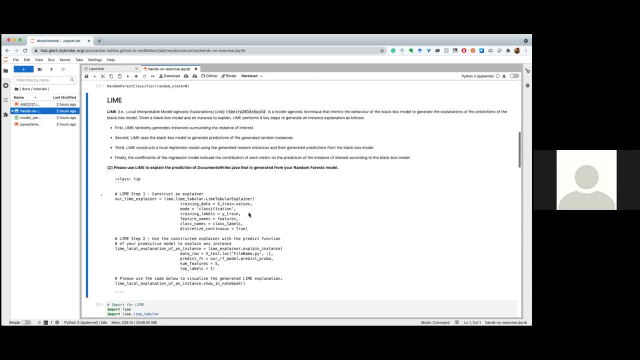 um. skip this one and here. so um first islam, and the second one is chap. i want to emphasize that these are very simple um. you can explain them using only three steps. so, basically, first you need to build the um explainer and then you can, you can use that explainer to to explain each. 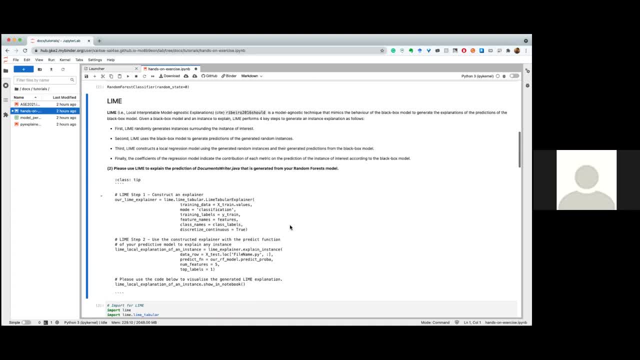 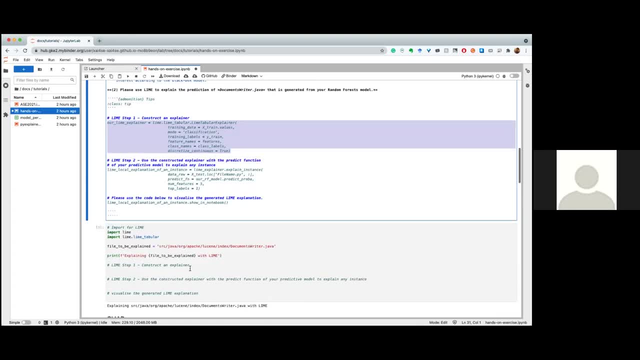 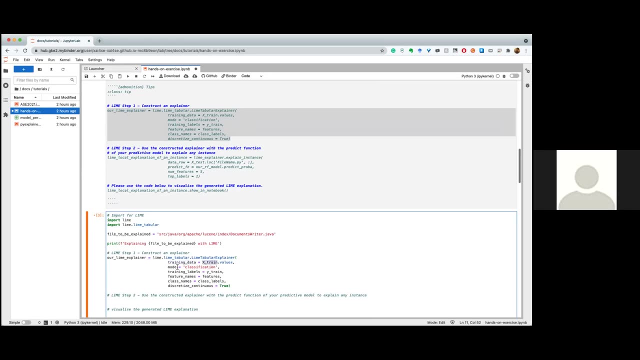 specific file or prediction. so let's start with the first step, okay, so, for example, lamb you, you can just simply input the training data, which are our extrins, and then you select the uh mode of the explanation can handle both classification, regression or other types of input, for example text, as well. 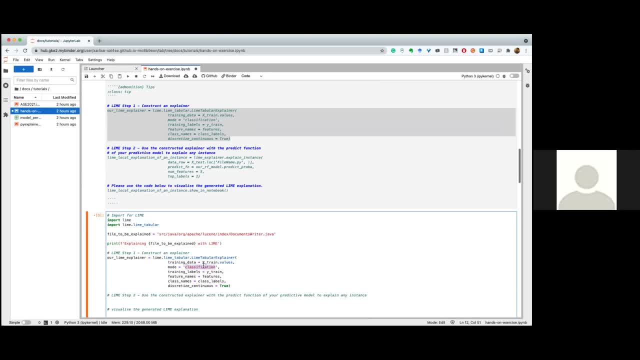 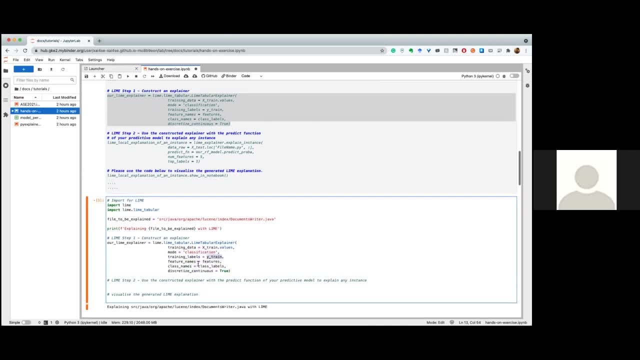 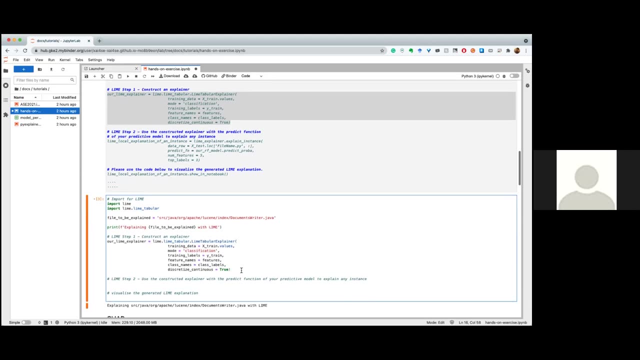 you can explore more in the document page of a lamb repository. and then we need the labels, and then the features, name and class labels and- and i mean in you can, if you are looking for example, a blank status, but you can see that there is an example, an example name. 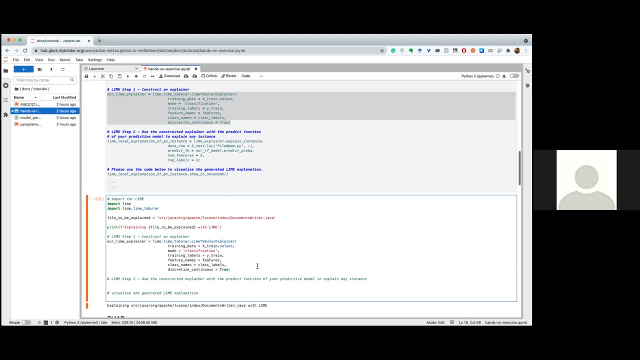 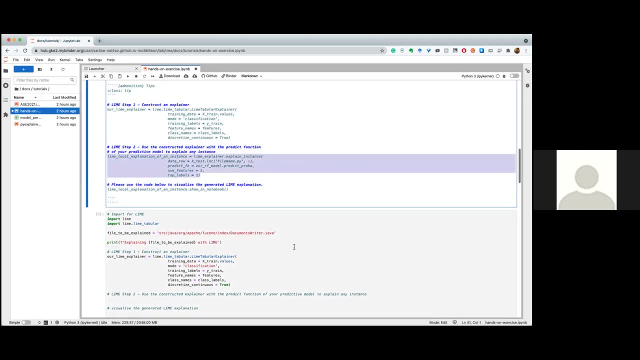 so here you can see the label names, and then the label name and the place where those labels are displayed. so that's basically the way to do it the other way around. so let's check the uh. so let's check one more time what kind of um expected input. you can print each of them in your 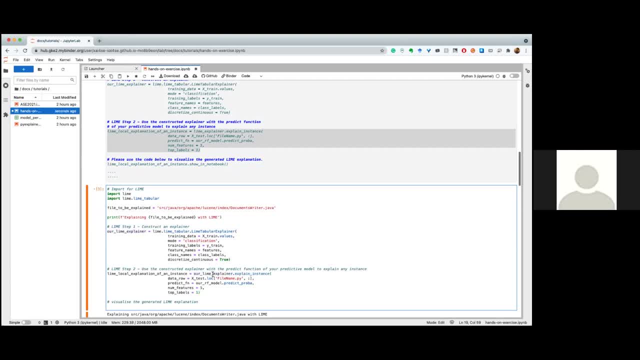 own um notebook now. so we have our lam explainer here, simple in one line. then we will use this um, this explainer, our explainer, oh, here. so we will use this, our lam explainer, to explain instance, and what we need for this function is the role that we want to explain to our familiar. 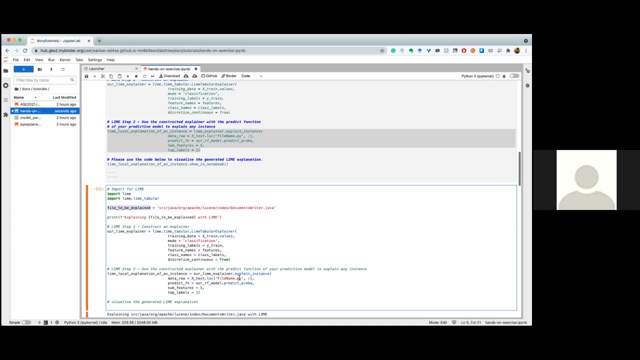 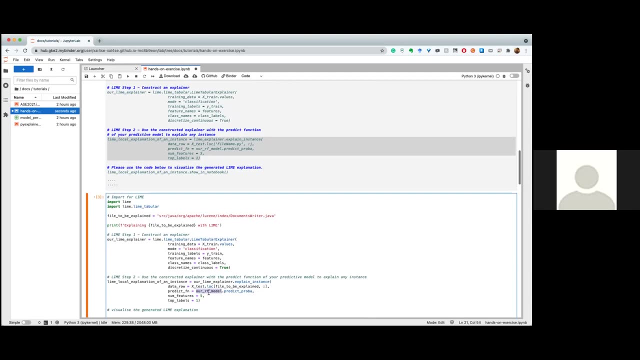 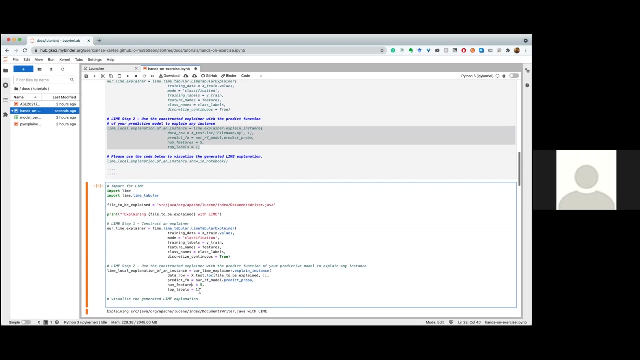 explain in this case, um. here we want to explain this: um document writer. right, so we need to replace this one. and then we need the predict function of our random for our black box model. in this case it's called: it is our if model. and then we need to specify how the um, how many. 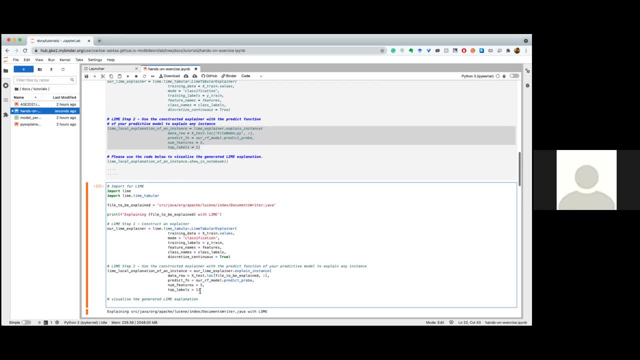 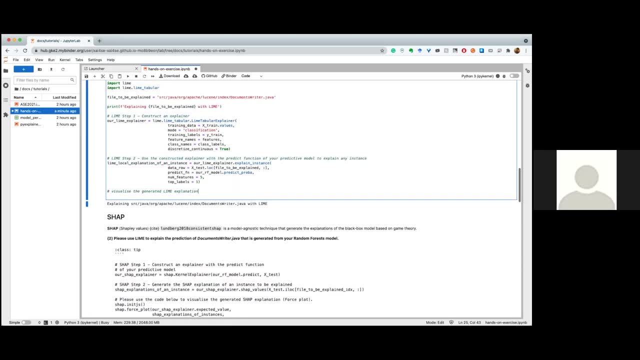 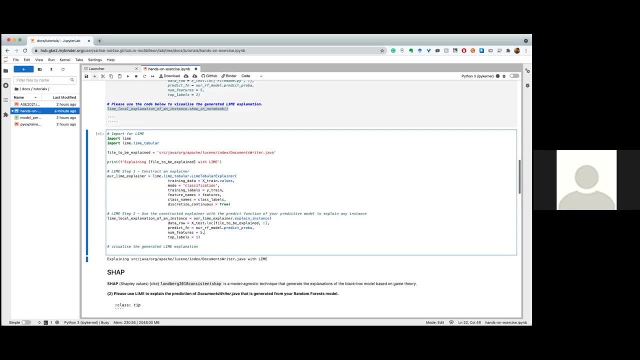 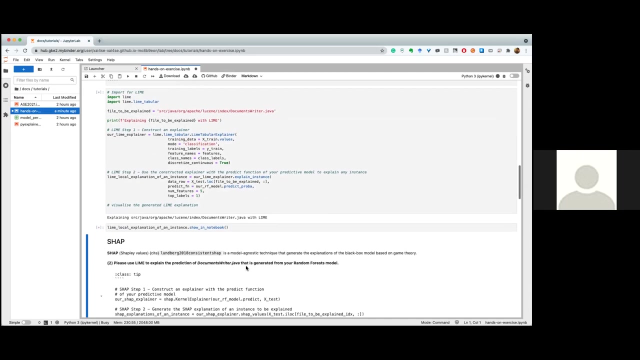 features that we need to um. uh, we want to explain and then we um run this one. okay, done, and now to visualize this um lamb local explanation of this instance. we can simply use show in notebook function. then lab will automatically generate the um visualization. okay, so now we can see how we can see that lamb is still, uh, working on generating the explanation. 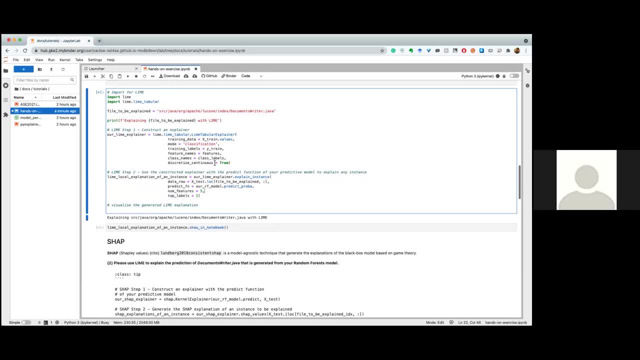 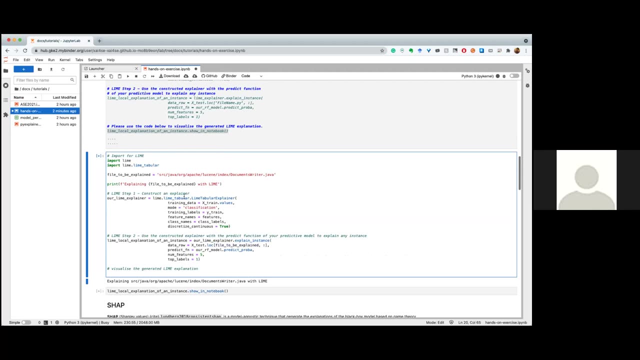 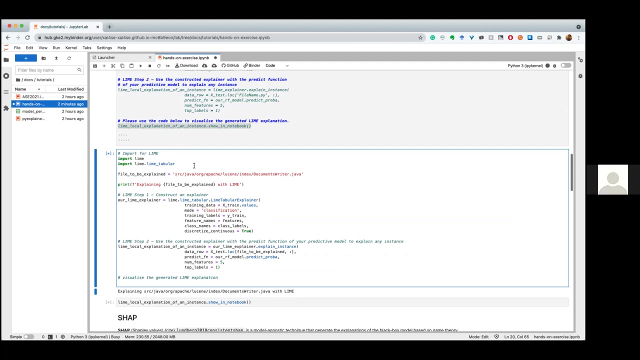 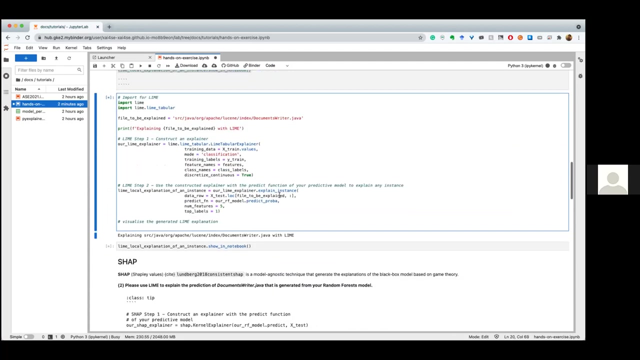 and it should not take long, i hope. at least, that's what, uh, i i discovered when trying this notebook. okay, we will, we'll go um. um, this does not happen when, when i test the notebook. but, um, okay, so let's imagine that we have lamb visualization and and um. 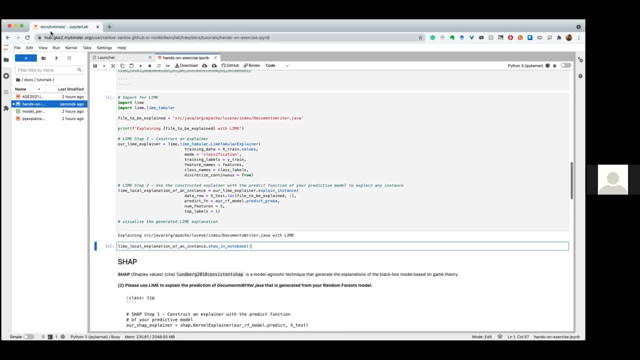 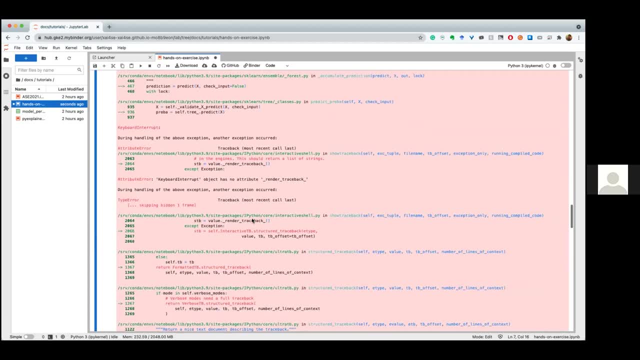 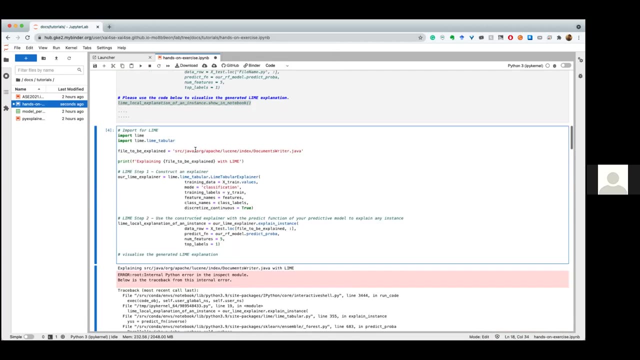 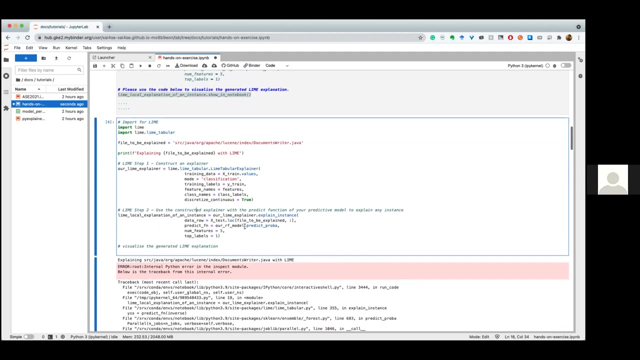 let's try to move on to the next one. um, um, okay, but but what? what i'm trying to emphasize here is that it's only three lines of code and maybe the data set is too small because this is just a sample data, or it has some problem with this environment. but you can try to explore more. 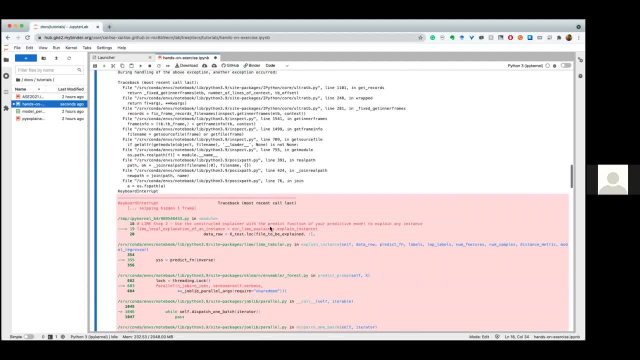 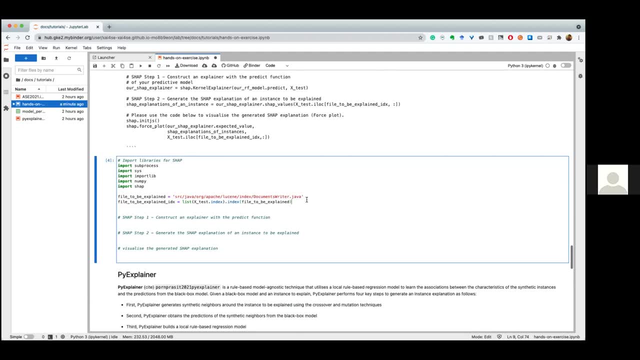 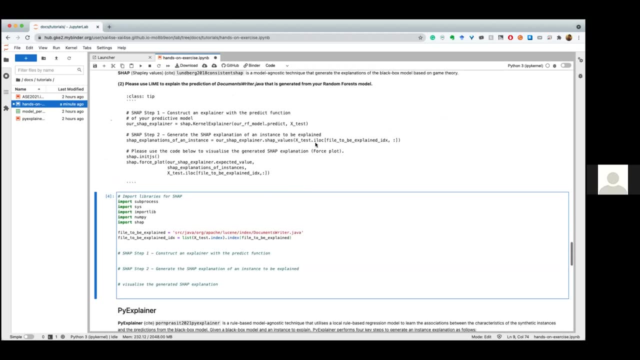 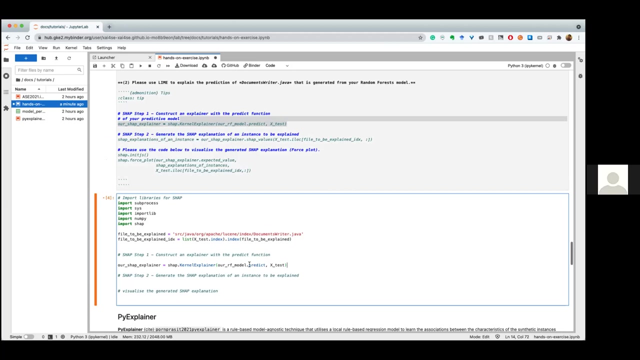 in your environment. it may work for you. and let's move on to the next one. okay, so here for SHAP as well. you can simply explain in two steps. no three, two. the first one is you need to construct the explainer similar to LAM, and to do so you just input here the expected. 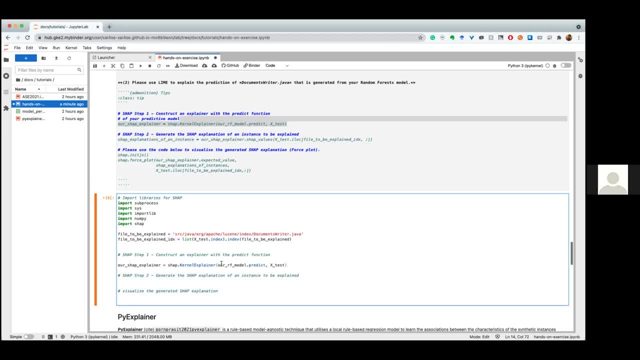 input for this function is your model, the predict function of your model and the data that you want to explain. so, in our case, is our IF model and X test. so here we are done with the first step, and then we can move on to the second part, which is generating the explanation for, for. 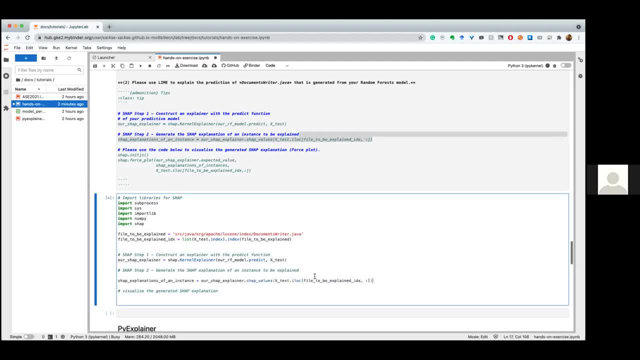 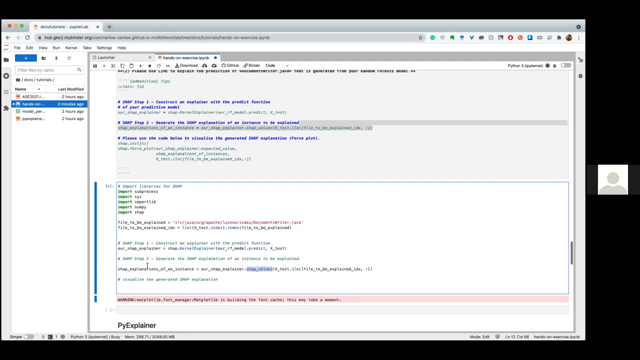 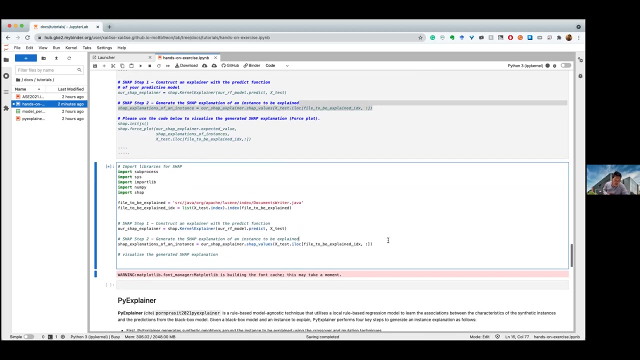 the file you want to explain. so, to do so, you just use the explainer and then use the SHAP value function. the expected input for this one is the, the instant that you want to explain, and hmm, so, so, so, so, so, so, um, okay, so, okay, so. 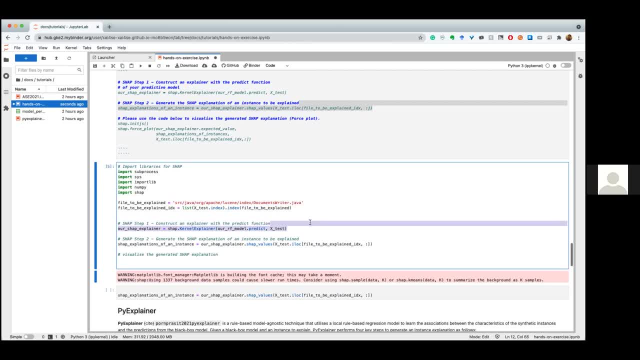 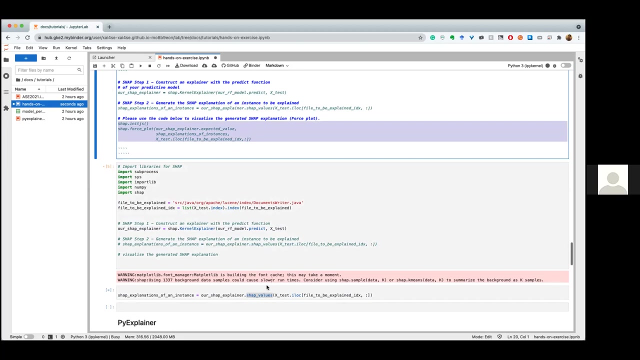 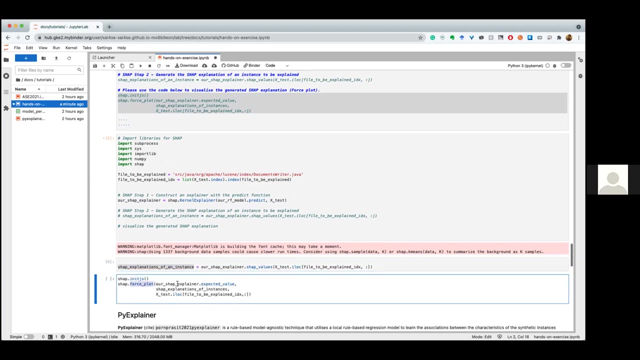 i did see that to uh the binder, to repeat this process, this line again. so here you can generate the explanation for this specific file with, just with this, simple functions, and after you have that, this explanation, to visualize using SHAP, you just use the force plot function, actually SHAP also. 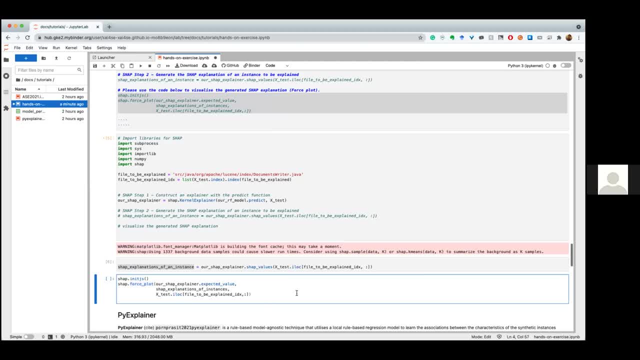 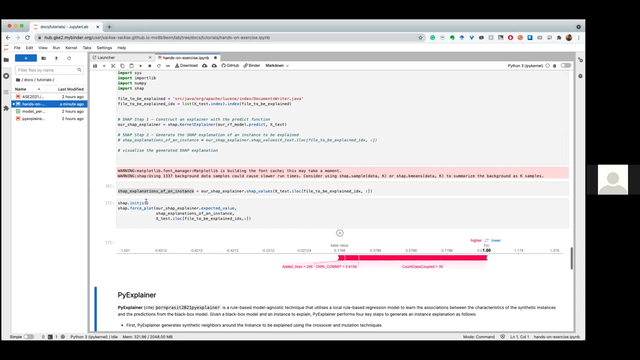 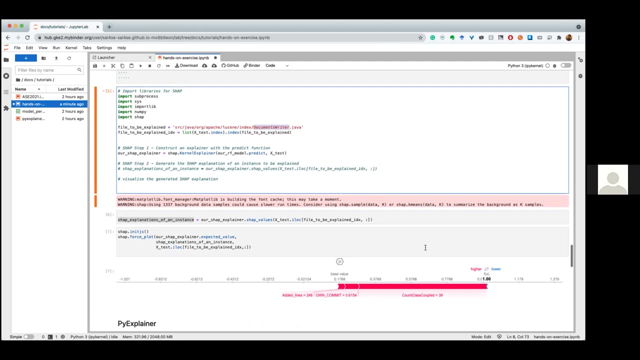 present other forms of visualization which you can explore in the repo page, but here you take this instance here to replace what you want to visualize and then press okay, oh, here. so here you can see that um SHAP generate the force plot for this um. um documents writerjava. and here in this example you can see that the predict probability of this. 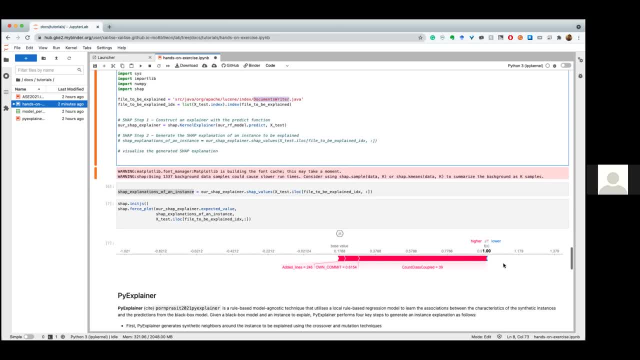 file being defective is 1.0 and the three top supporters, I mean the three top um variables that come together, are the one that's showed at the bottom of the screen and the ones that are not, because in this case, the these are the highest case, but we don't have to say the exact what's. 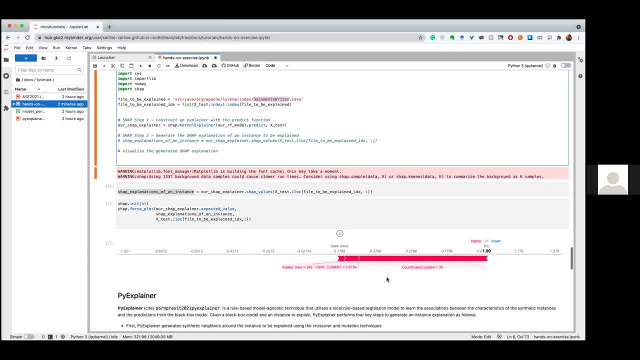 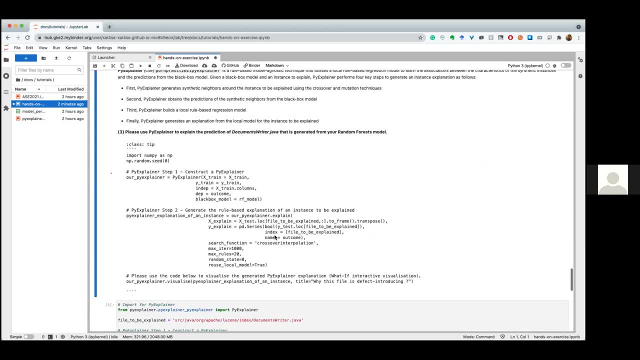 the highest case. but you can see um. this is the reason why we didn't take in. okay, and we're contribute to these predictions are: count class, couple, own commits and added line. Okay, here the PI explainer. Okay, we still have time. 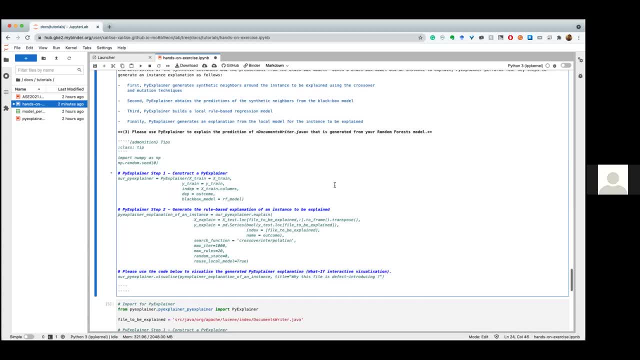 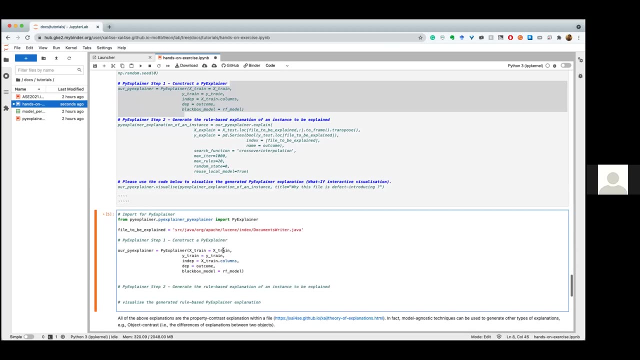 So I'll try to cover this one as well. Similarly, you can explain this- the file- with PI explainer with only three simple steps. So first you construct the explainer. the expected input for this one are the training data for both independent variables. 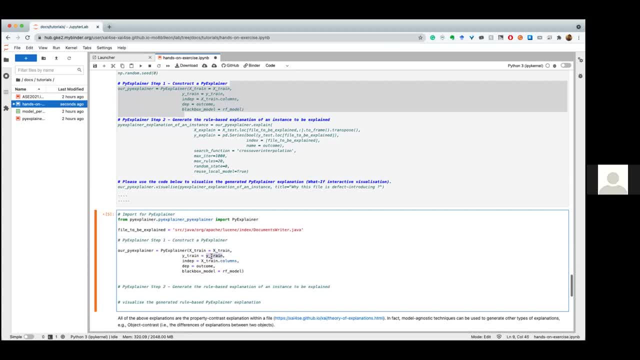 and the outcome on the dependent variables, And then you just input the column names of the independent variables and then you need the black box models. So in this case the name is our RF model, and then this one should run fine. And then 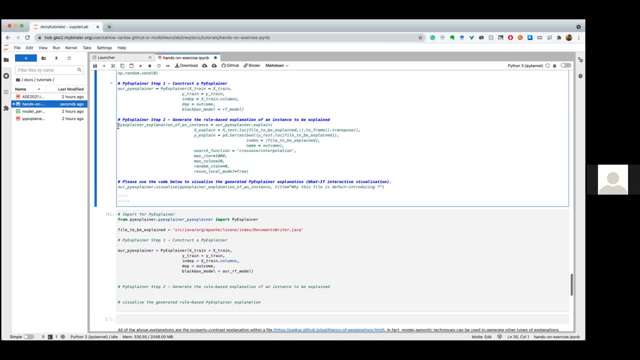 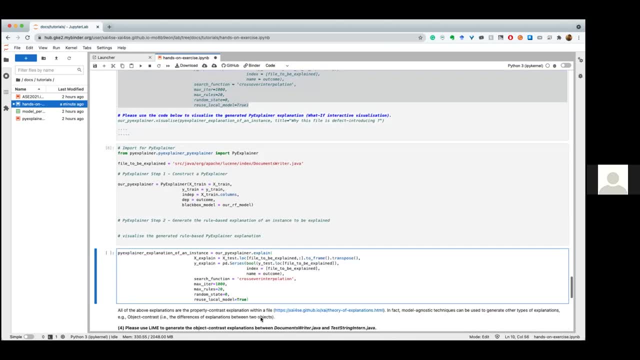 After you have the explainer, you similarly explain the instance with this function. So it's called the explain function and the expected inputs are: first: the instance that you want to explain in our case is document writerjava. You just input it here. 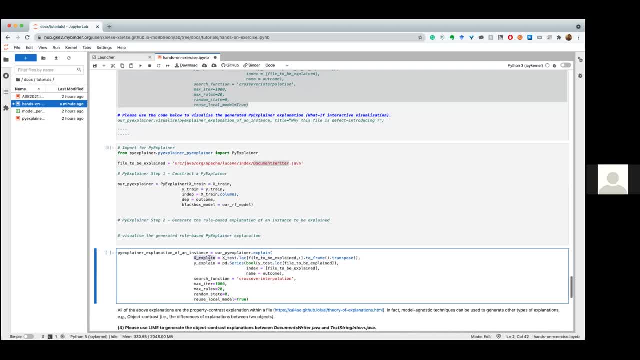 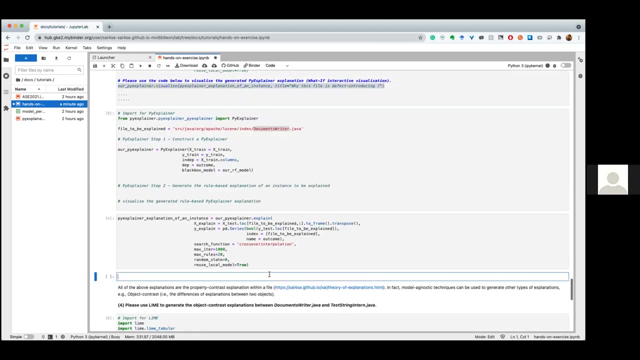 And then the level of this is the name of the file that you want to explain. Then you select the search function- max, The number of max, extremation, number of rules and so on, And then you run it here And finally, after you have the explanation, 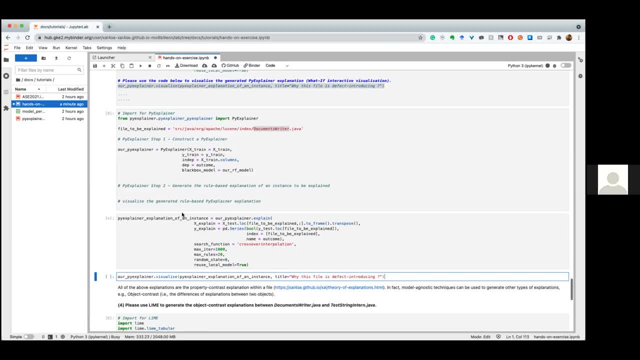 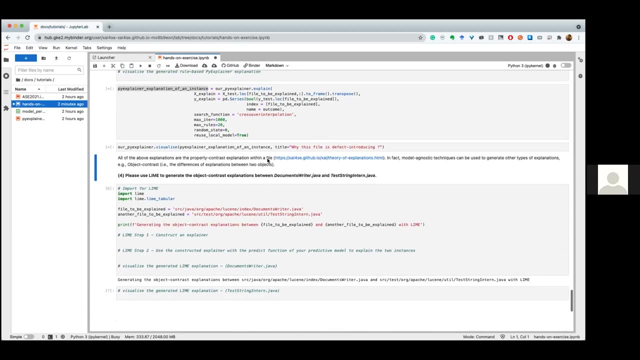 to visualize the PI explainer explanation. you just take the instance No, this instance, and then you visualize with this function. okay, this will may take a while, so i'll move on to the fourth one. so the last one is a bit tricky. here, please use slam to generate the object. 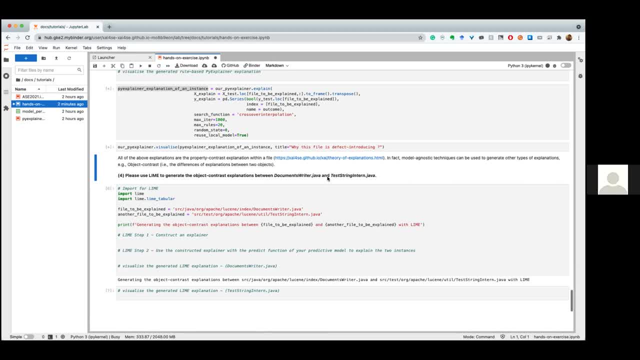 contract explanation between document writer dot java and test string internal java, so in in the presentation class- has already covered several types of contrast contrast explanations, for example property contrast, time contrast and object contrast. so to recap that explanation, that definition, object contrast is the contrast between two objects. so you are so in this exercise. 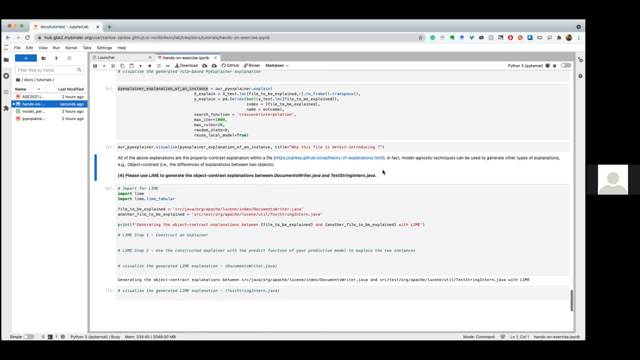 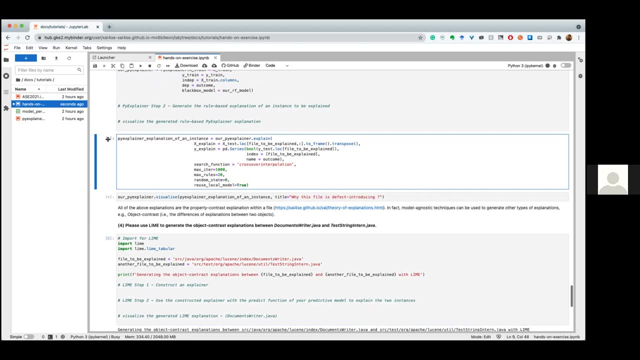 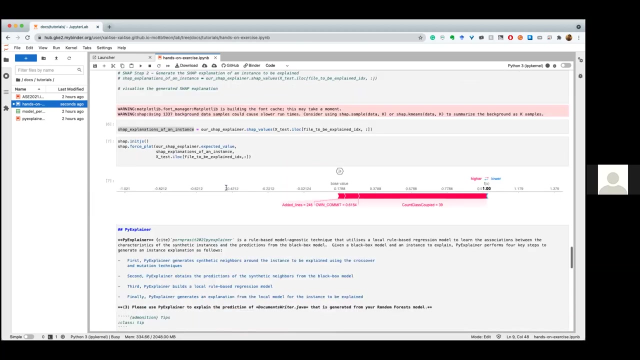 we are. we are going to generate two explanations for document writer and test string intern and try to compare and contrast between the two of them. okay, so it seems that vinyl is still working on this cell, so i will first prepare some code, so i'll go back and take the code from this one. 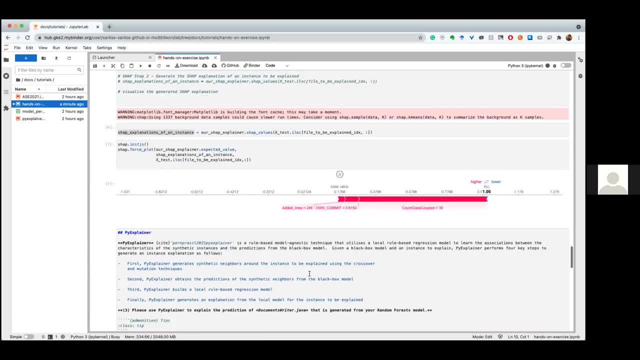 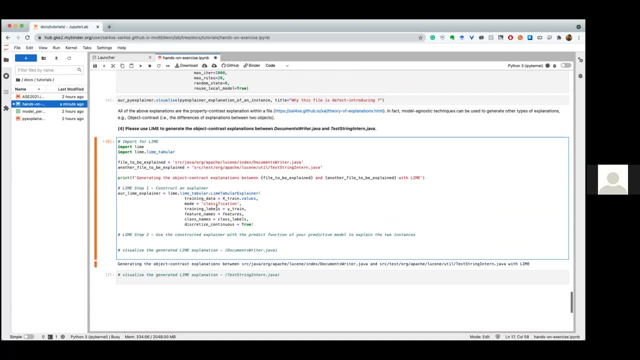 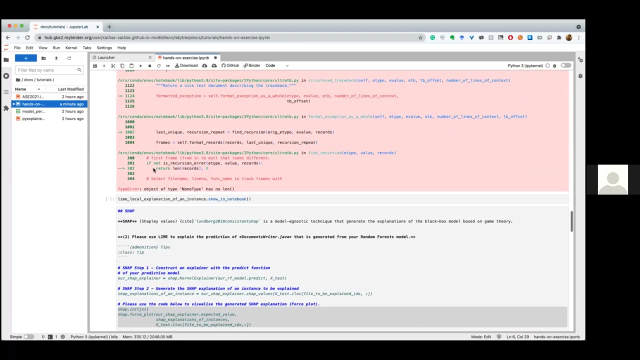 okay, so we have already, uh, finished the first step here, because here the first step is very simple: you, you construct the explainer with this one, and then you need to to generate the prediction for the first file and the second file that you want to compare with the first one, and to do so we need two lines here. 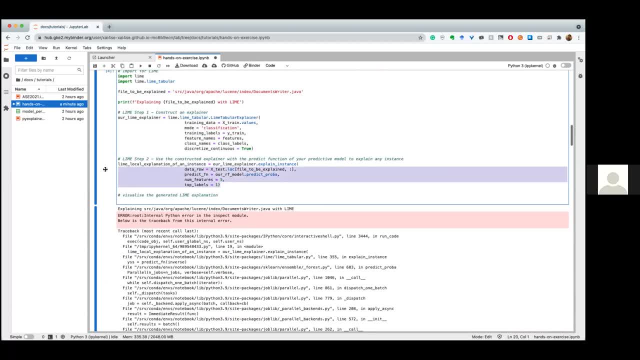 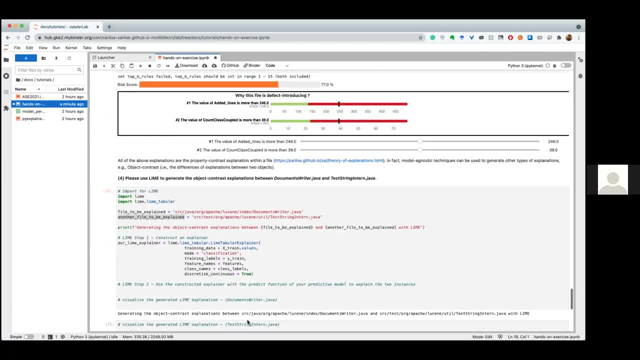 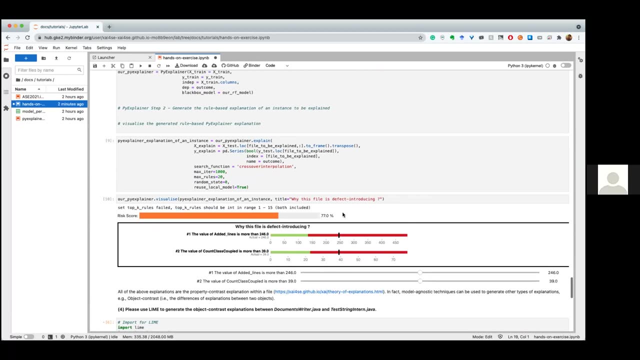 let me go back, okay, okay, so i will just make sure this one is correct. oh, here i explain. it is done with the job. so here you can see the um explanation here. so the risk score here is the predict probability of this five being defective and here you can interact with the visualization and it will try to 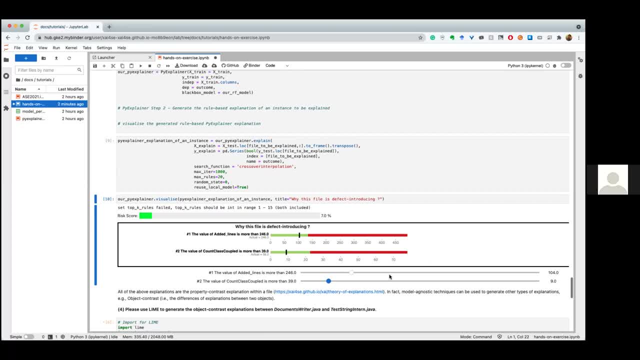 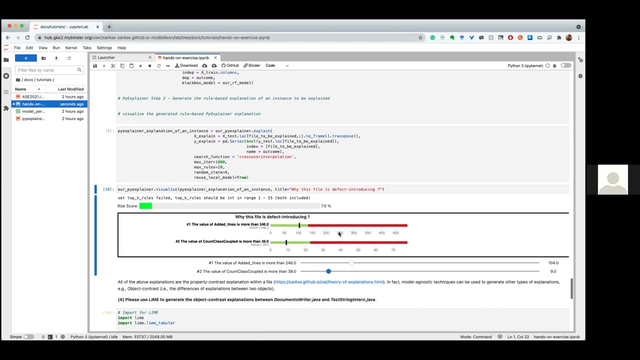 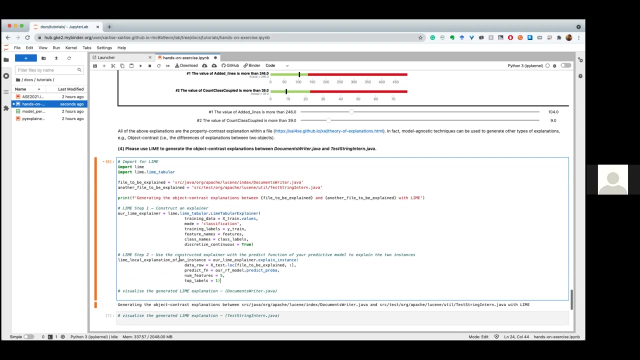 regenerate the predict probability, ah here. so if you lower the added line and count class couple, you can see that the predict probability of this one being effective is reduced to seven percent. and that is the basic idea of what is visualization of pipe planner. now, um. so here, here's how, um. so of the first instance. so the first one is: 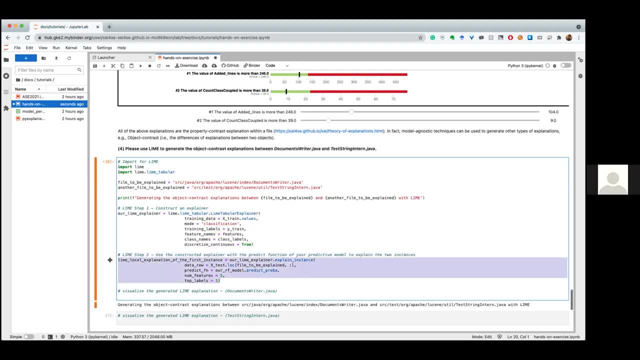 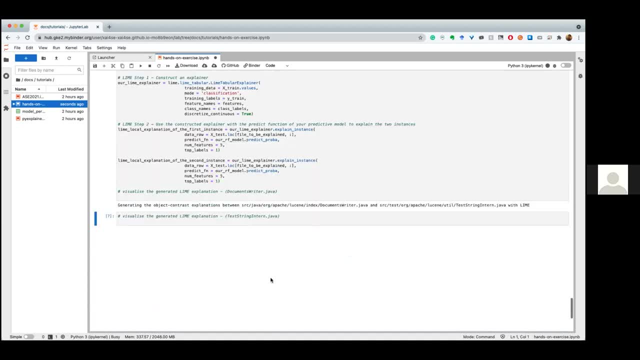 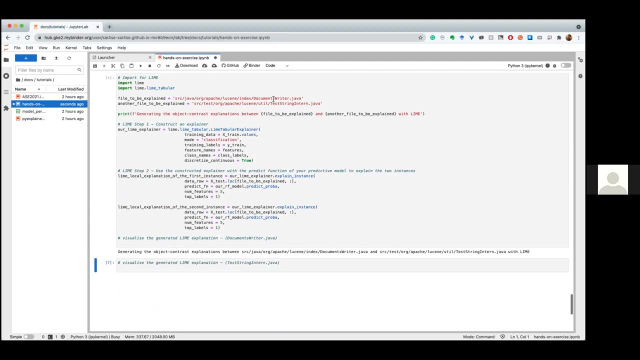 uh, the file to be explained, right, and the second one is um. here the second instance. executing these two lines, you can generate the um, the property contrast of documents, writer and test spring intern. and to generate the object contrast of these two one, two files, you need to visualize both of them. so to do so, let me go back and have a look on how to. 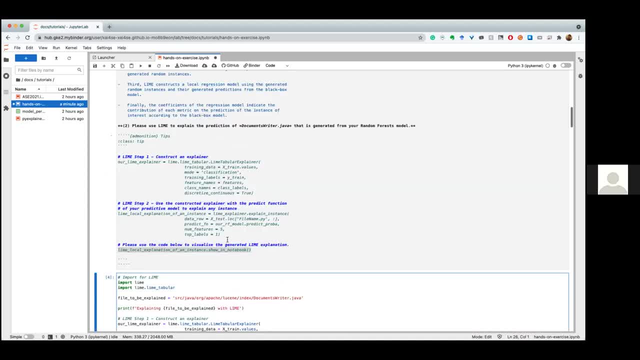 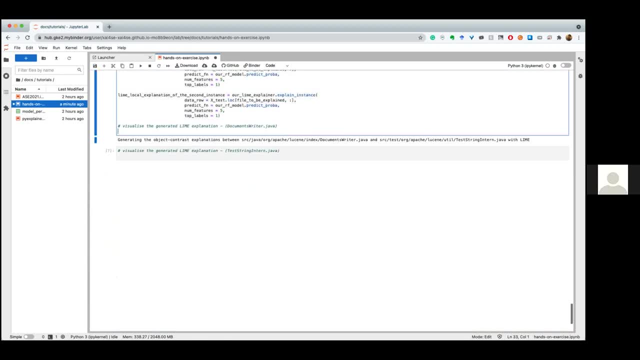 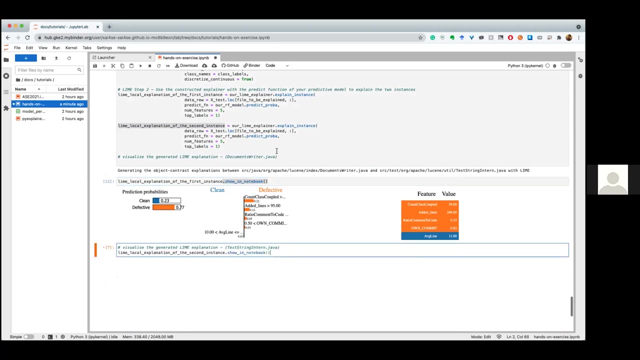 you know here. okay, so it's very simple. it's just a showing notebook. so first you need to show in notebook for the first file here and you also need to show in notebook for the second one. okay, so it works now. i didn't make any changes for the. i mean, the first file wasn't the first one i set in my muchas. 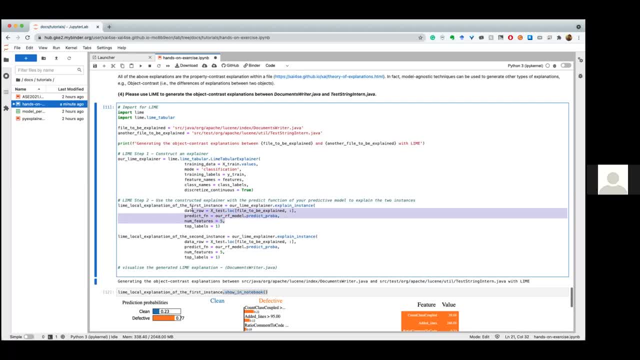 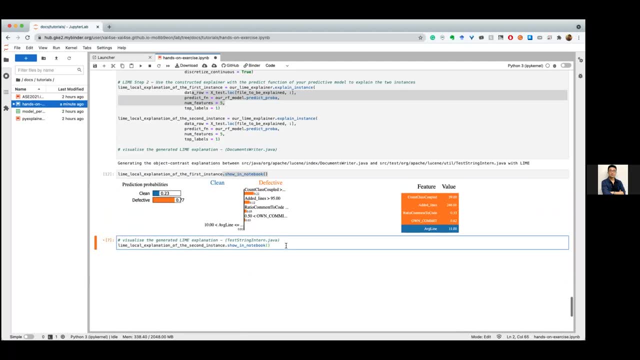 same uh file with the previous roles, i mean previous sales. but, um, yeah, please go ahead. can you please ask again in english, please should be fine. i think someone is unmuted. yeah, please go ahead. okay, sure, so here we can see that uh in in cell number 12. 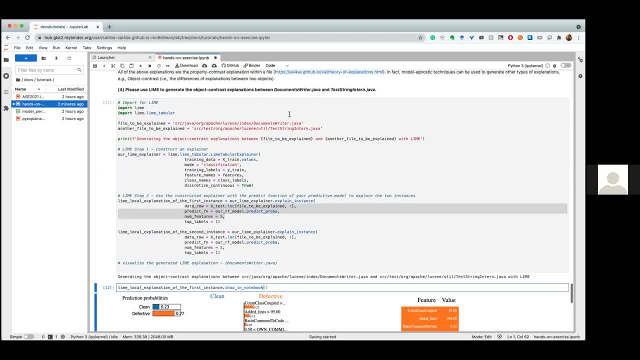 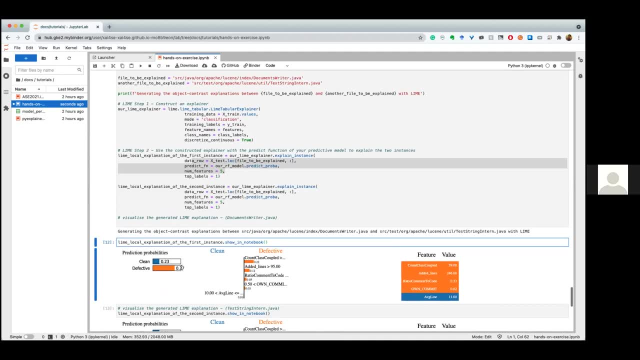 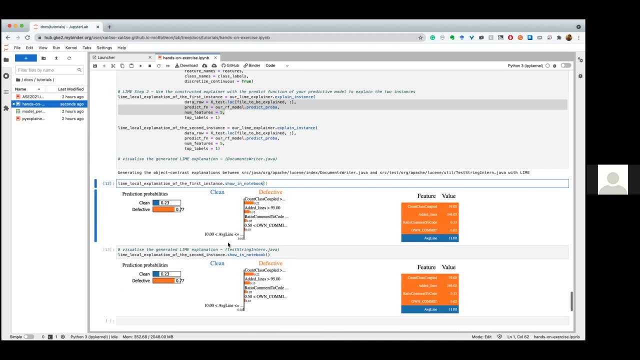 we can see the property contrast of the first file or documents writer. it says that this one has the predict probability of being defective for 77 percent and the three main reasons are here. similarly for the second one. this one has a second instance. ah, i made a mistake. i need to. 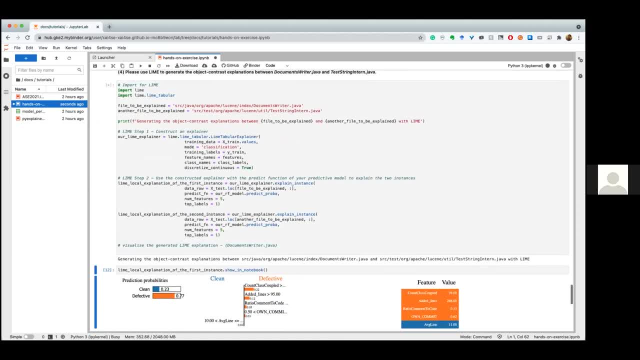 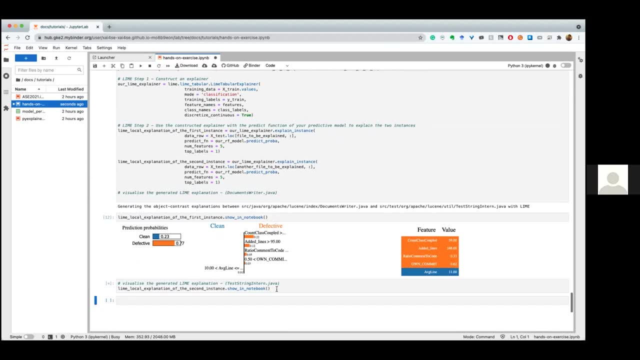 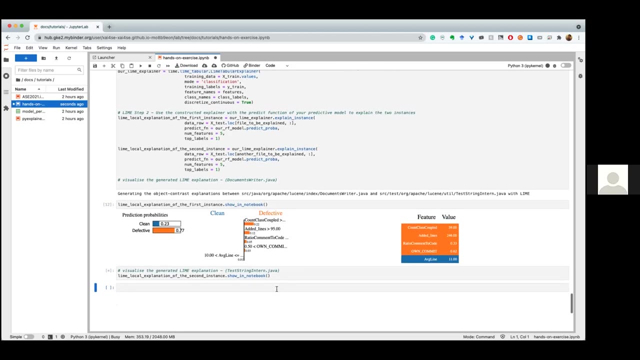 change. okay, sorry, uh, i will regenerate the explanation and if it is done, then we should get the the explanation for the second one. but, um, basically you get the idea. we went to generate the object contrast. you just generate two property contrast of the two files and yeah, basically that's it, that's all. oh, here we can see that for this. 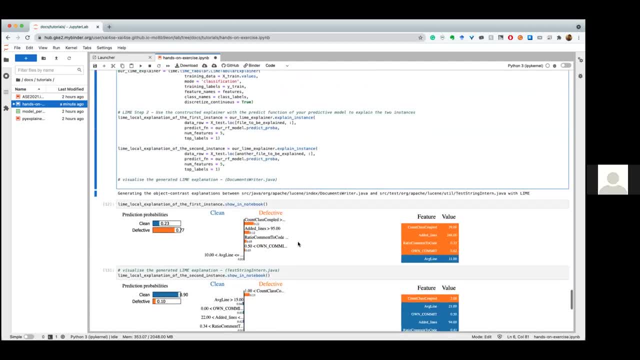 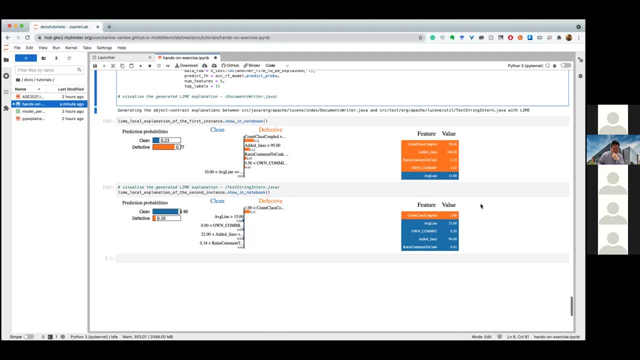 um documents, right? uh, no, test string internsjava. this one is likely to be clean. so the same thing with the predict probability of 90 and the. the main reasons are these: um four values, and that's all for the um hands-on um exercise. thank you very much. now, uh, passing. 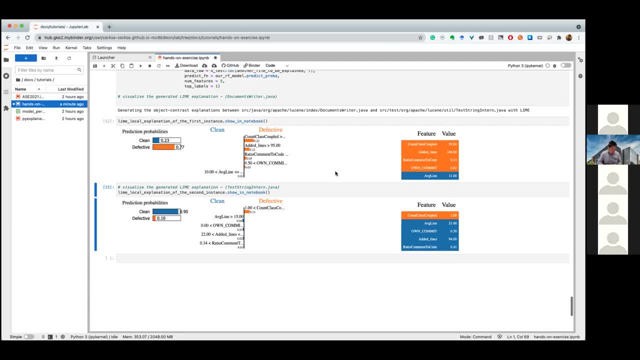 on to class. hello, thanks, uh, tirayut. yeah, i think, uh, we did great. uh, the the hands-on is successful, yay, yep. so i think uh, yeah, i think uh, maybe go. I think I'll just open the opportunities for the audience, If you have. 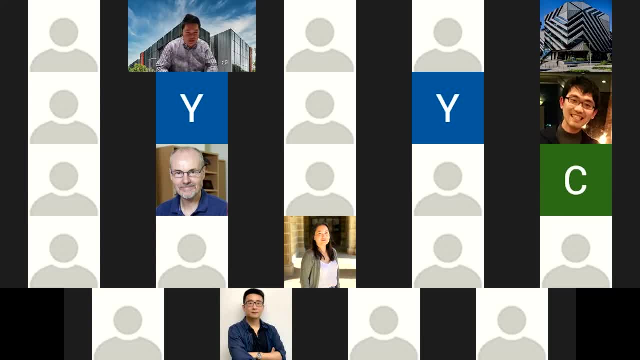 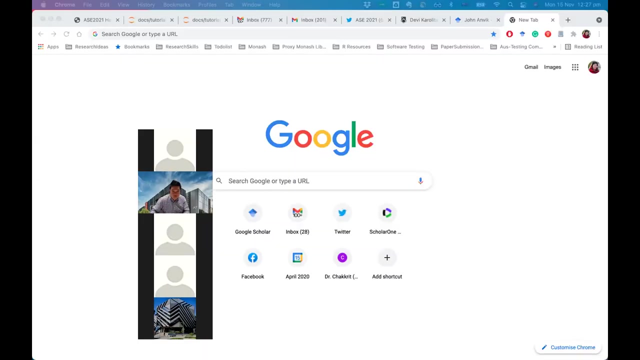 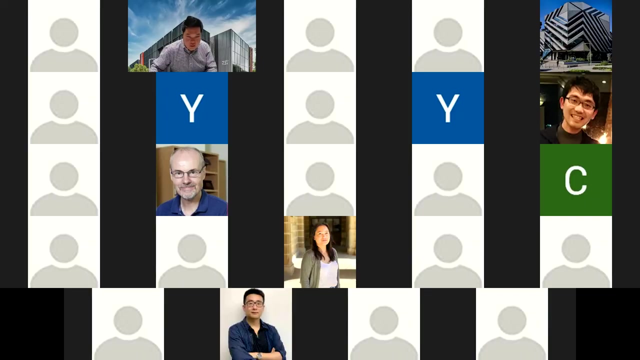 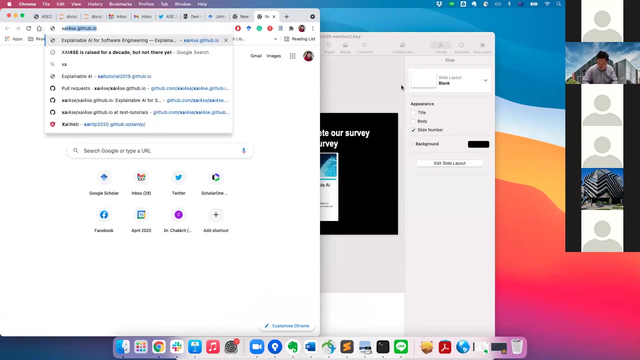 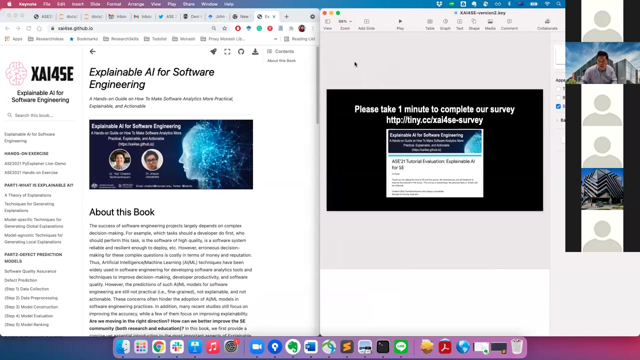 any question. please feel free to ask me Questions. Questions No, Then yep, Yep, So maybe I will just open the wrap-up. Okay, I think we did great. We have two more minutes, So anyone in? 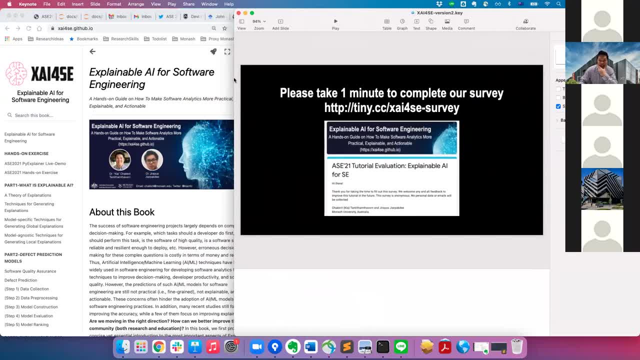 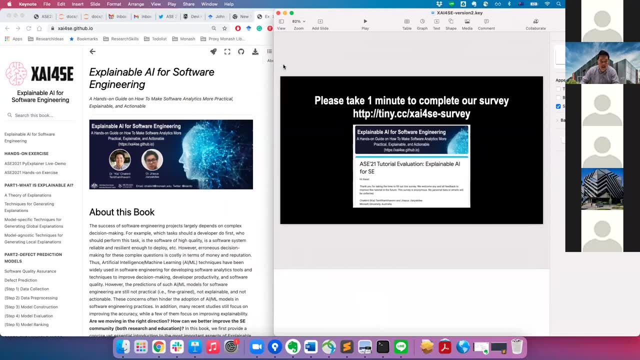 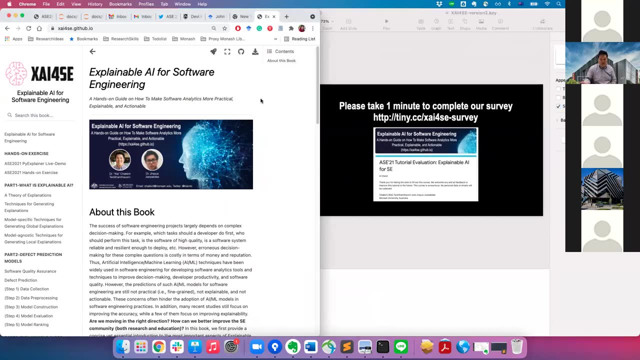 this tutorial. could you please complete the survey? tinycc slash xai4se dash survey. Yeah, any feedbacks or comments are really appreciated. Okay, So just want to wrap up the tutorial. today We make lots of. we discuss a lot about. 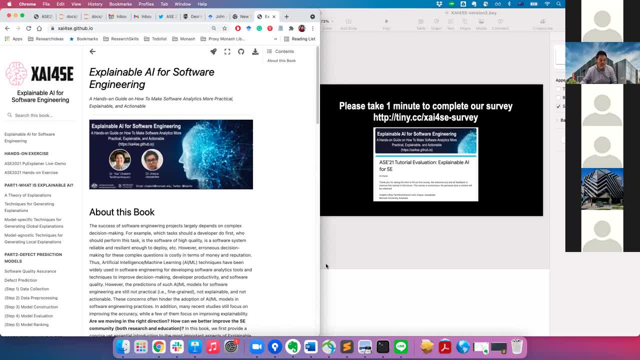 how can, why the explainable AI is very important in software engineering and how can we make it useful. We also discuss about the potential use of scenarios, about how can we make the different prediction models more practical, more explainable and more actionable. 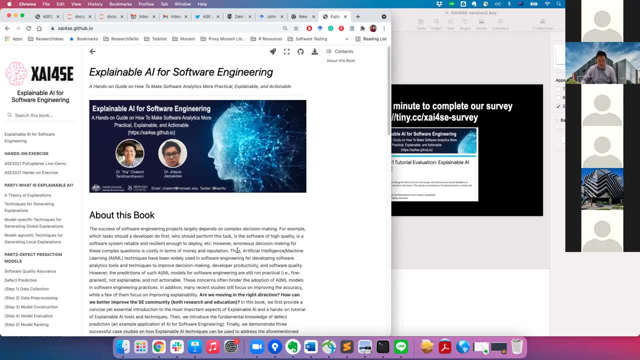 So if you are interested and if you would like to learn more, please feel free to contact us. Please feel free to go to our book xai4segithubio. If you want to run any code, just go to here and go to click. just launch the. 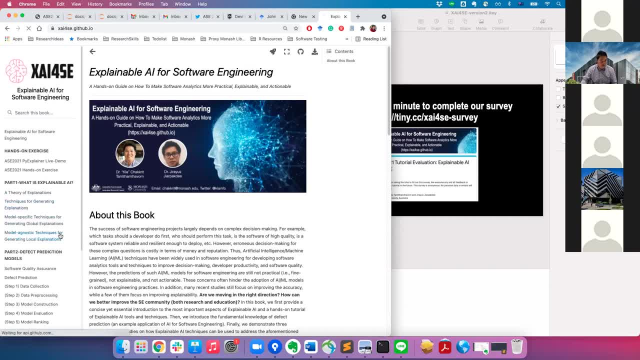 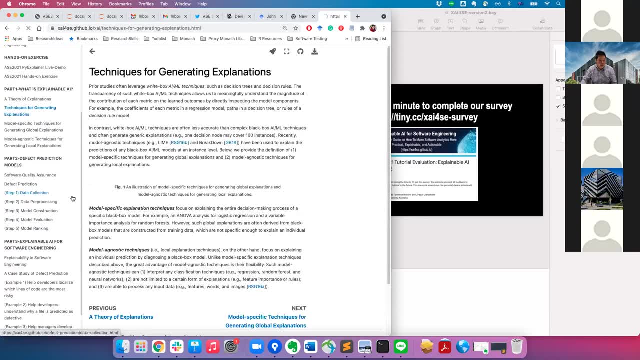 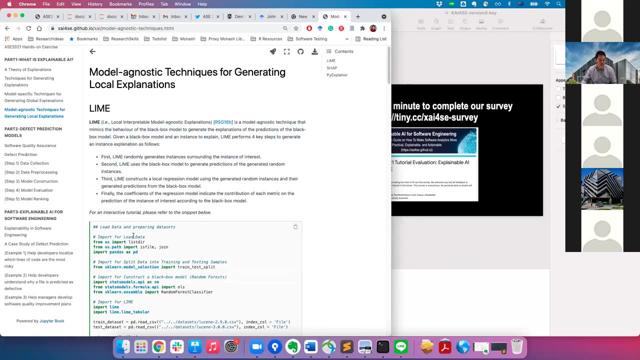 bider and then you can enjoy Yep. So in this tutorial we talk about what is the theories of the explanation and we talk about what are the techniques to generate the explanation. We also discuss about like how can we use LAMP.